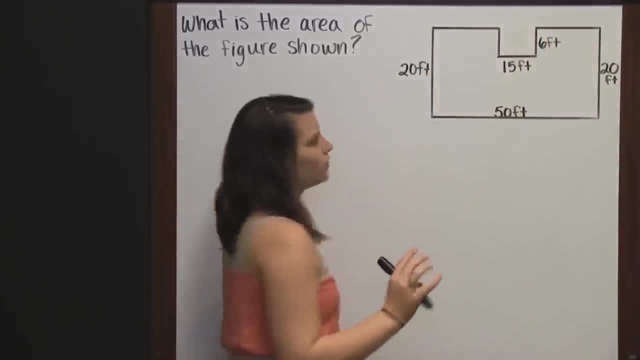 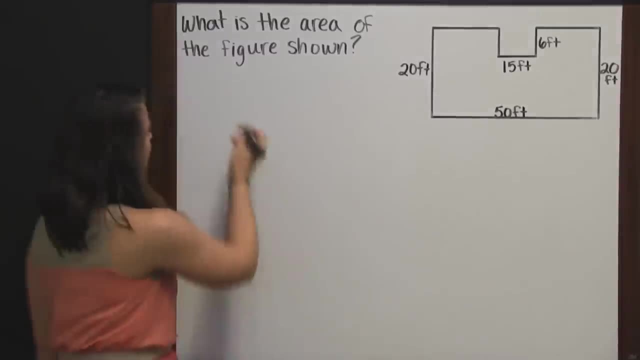 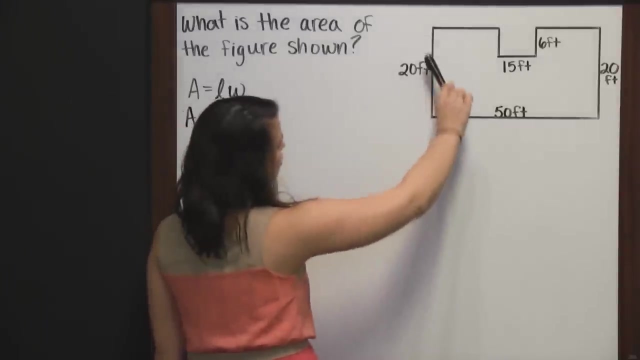 the only part that's missing out of this large rectangle. So first we'll find the area of the large rectangle, and the area of a rectangle is the length times the width. So the area of the large rectangle is 20 feet times 50 feet. 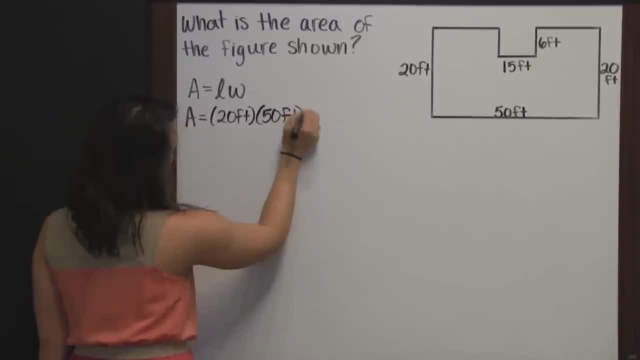 So the area is 2 times 5 is 10, 0, 0, 1,000 feet times feet feet squared. The area of the large rectangle is 1,000 feet squared. Now I need to find the area of this. 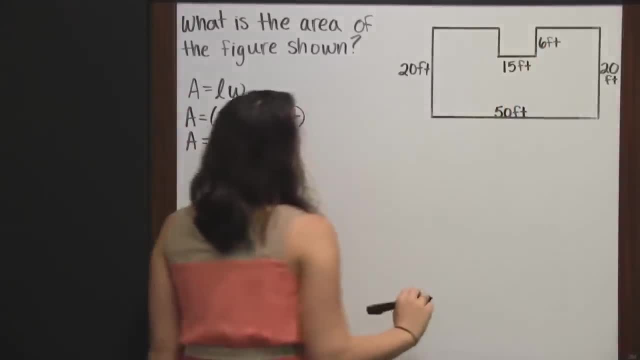 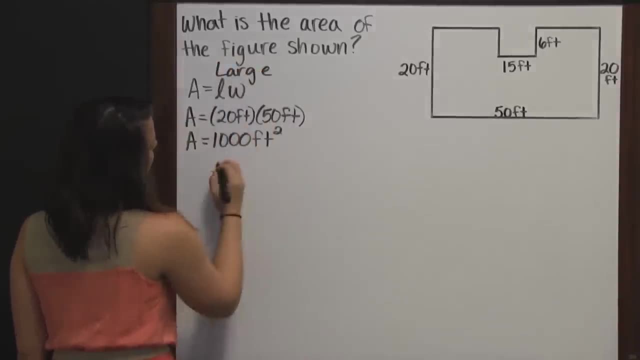 smaller rectangle, the only part that's missing out of our large rectangle. So I'm going label this: This is the area of the large rectangle. Now we're going to find the area of the small rectangle. So, again, area is the length times the width And we have the 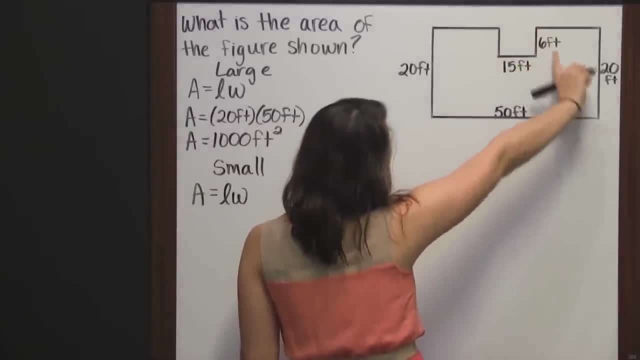 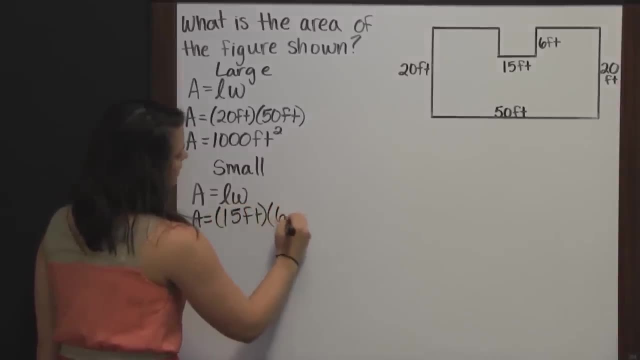 length and the width for our small rectangle as well. Fifteen feet and six feet. So the area is fifteen feet times six feet. Six times ten is sixty. Six times five is thirty. So thirty plus sixty is ninety. Feet times feet is feet squared. So the area of this little 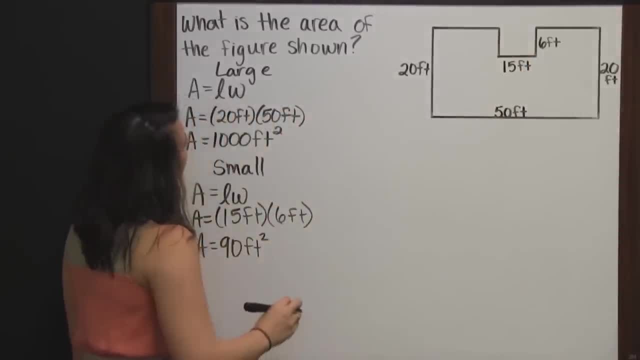 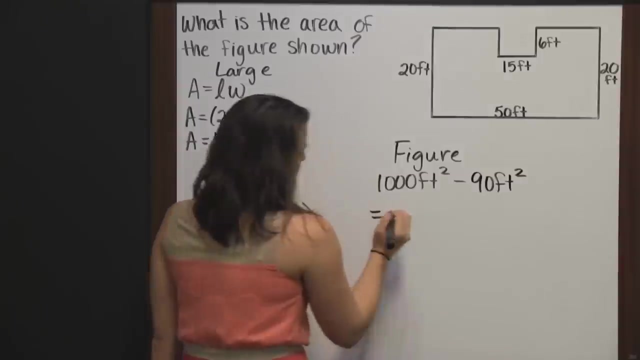 rectangle is ninety feet squared. So to find the area of this figure we're going to need to subtract the area of our large rectangle one thousand feet squared, minus the area of that small rectangle cut out which is ninety feet squared And a thousand minus. 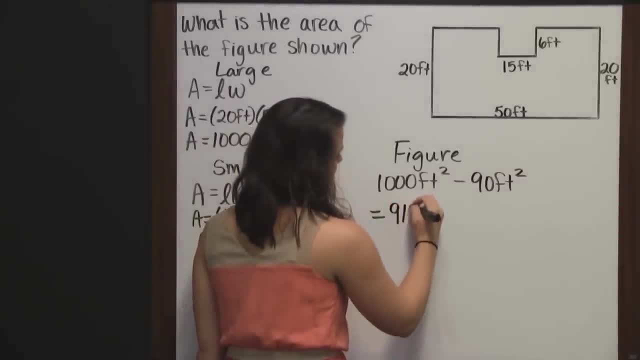 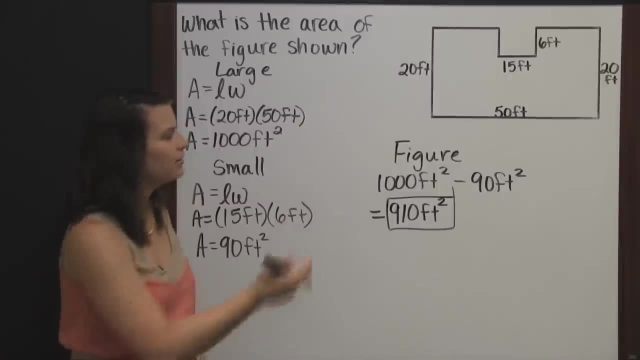 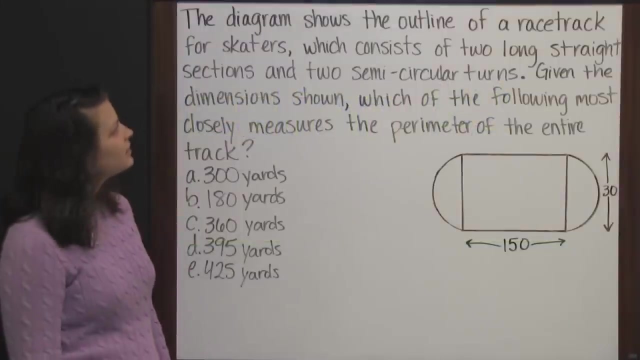 ninety is nine hundred ten feet squared, And that's the area of our large rectangle. So that's the area of our figure. The diagram shows the outline of a race track for skaters which consists of two long straight sections and two semi-circular turns. Given the dimensions shown, which of the following? 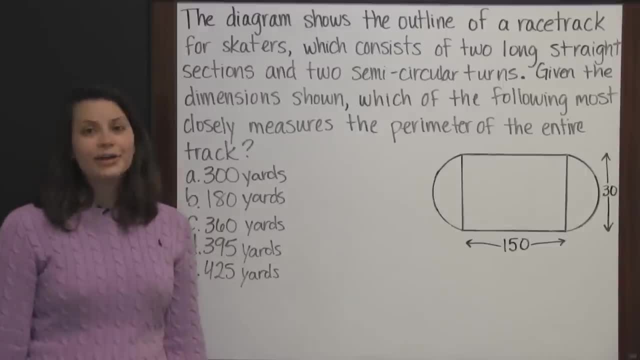 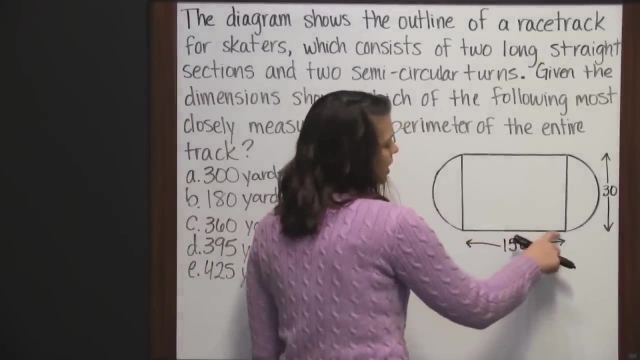 most closely measures the perimeter of the entire track. Well, they've got to be the Richard Scruggs bragmesiating sides to start with, Alright. so they range over nine inches from the square of one hundred and fifteen, So we have about three hundred and seventy. 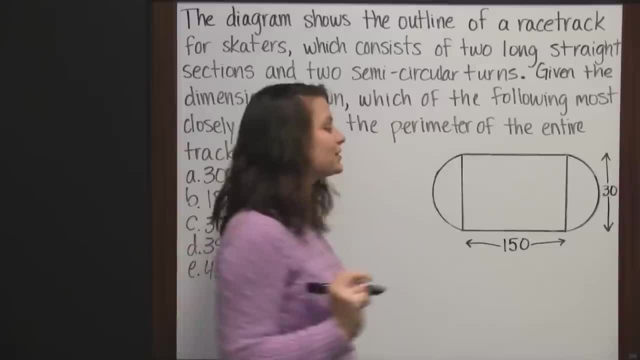 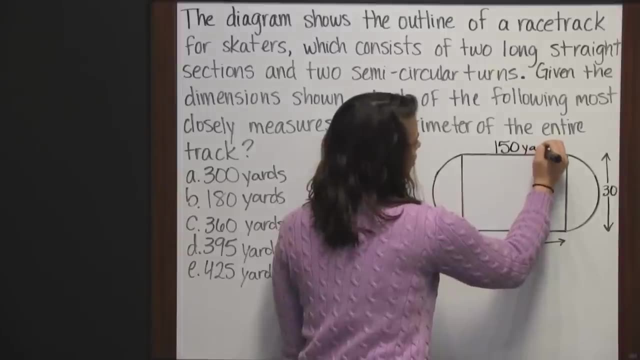 and fifty four inches in length, So the length of that side here are two hundred and seventy four inches. They are roughly the same length but they're not straight Yards, although they have already been derived from the top of this Σ axis. that is going to equal the length. 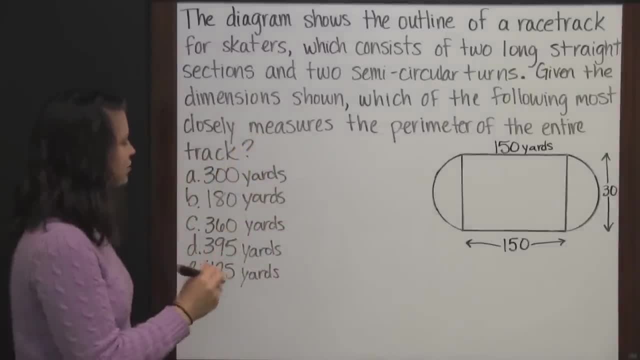 of the bottom. So it is one hundred fifty two inches, not three hundred and fifty four inches of length. And then we have the non- Mustang distance between them: One hundred and fifty four inches, not three hundred and fifty four inches, Adjusting two y cours of. 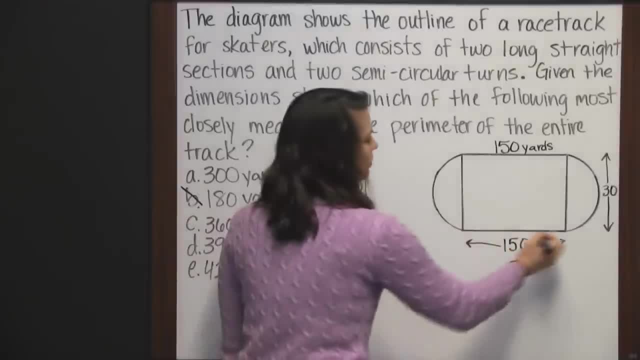 our diagram is one-をn- ers, The value of one hundred and fifty four inches. the value or radius would also include two y cousins, so that we already see thaturan感覺. not enough, because I've got 150 and 150.. So we're going to have to skate this. 150, skate. 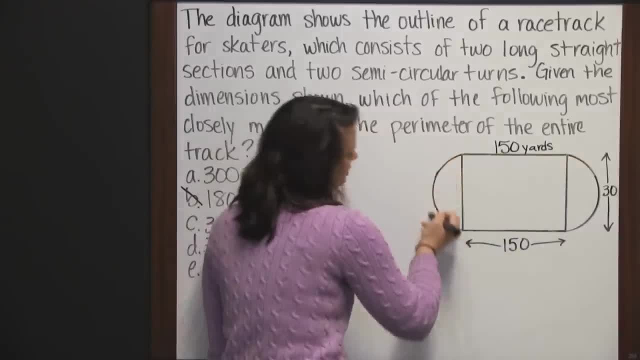 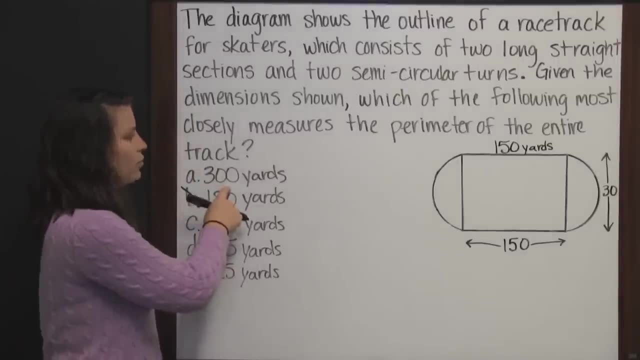 some more, skate another 150, and skate some more. So we know we're already over 180 yards. We also know it's going to be more than 300 yards because just the two straight sections are 300 yards. So we can already eliminate that answer choice And we're down to these. 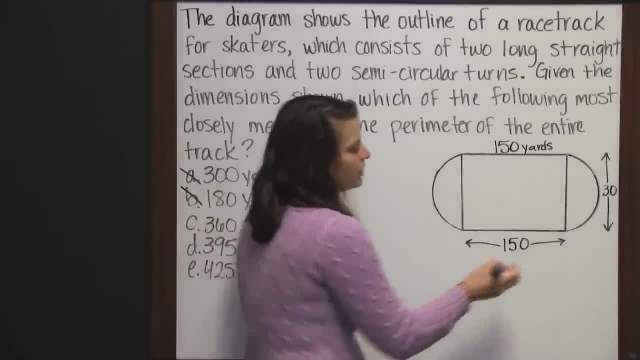 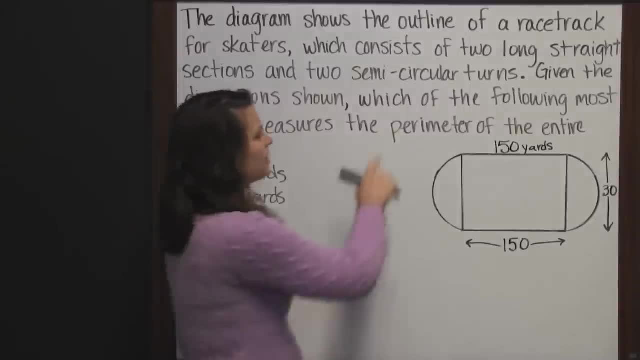 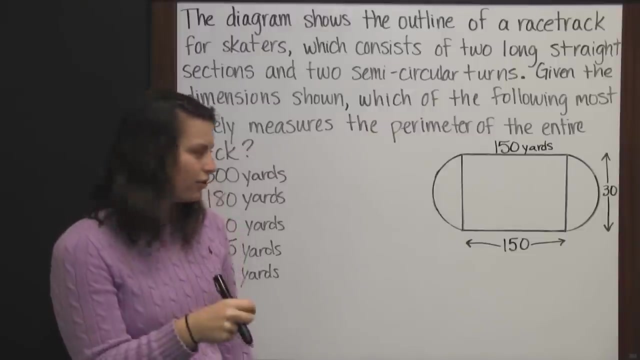 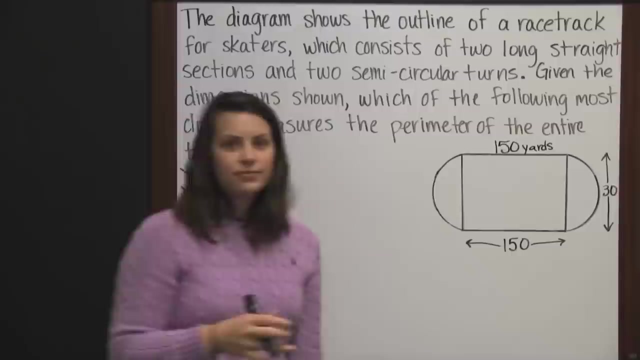 three possibilities. So that means we need to figure out what this distance is here and here. They told us that these were semicircular turns. That means that semi- that semi means half a circle. So if you take these two halves of a circle and you put them together, 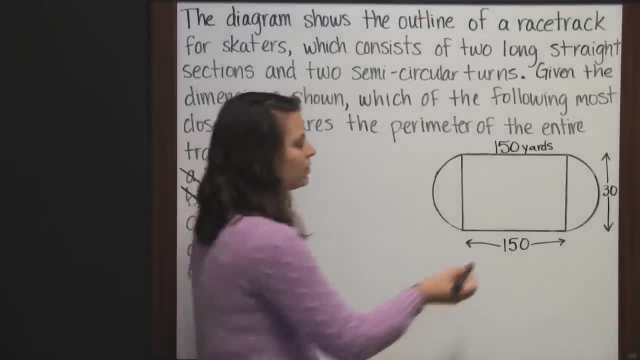 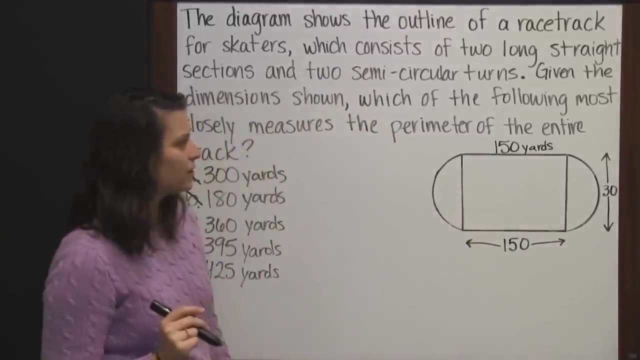 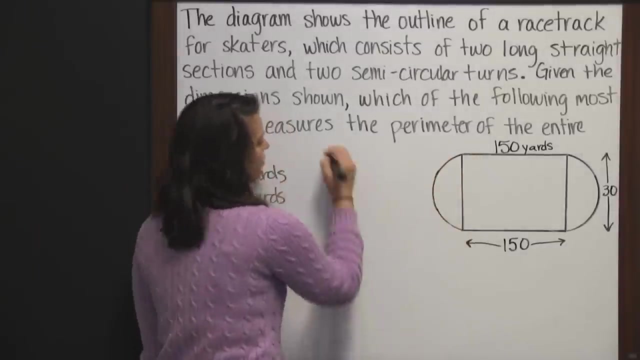 you get one whole circle. So really they're travelling the distance of 80 yards of one whole circle, in addition to these straight sides here, which means we need to find the circumference of our circle, to find the distance around the circle. That's what circumference? 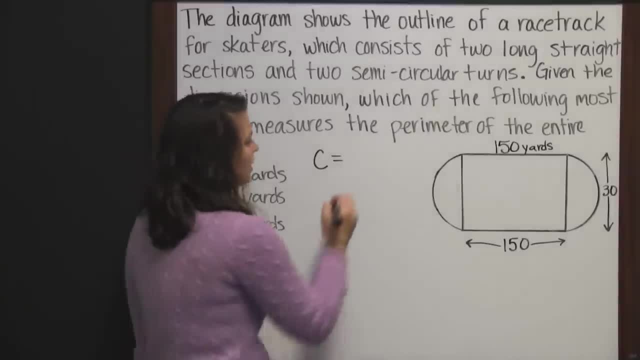 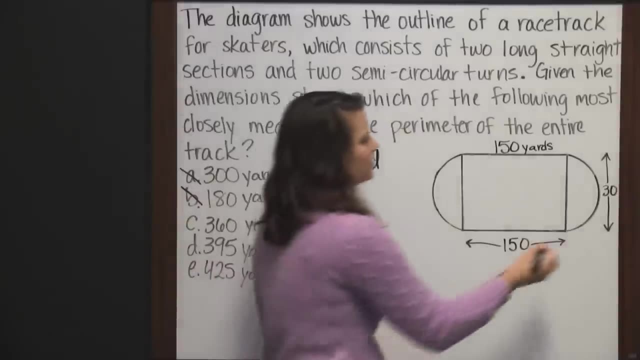 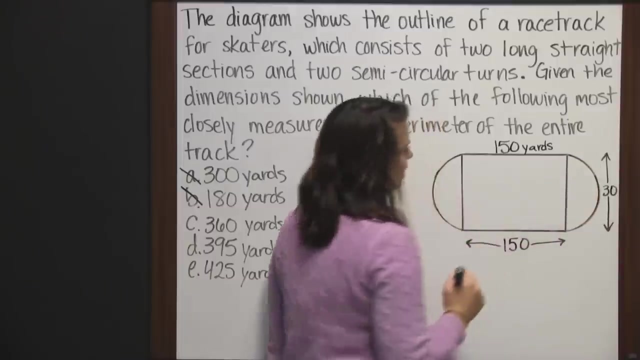 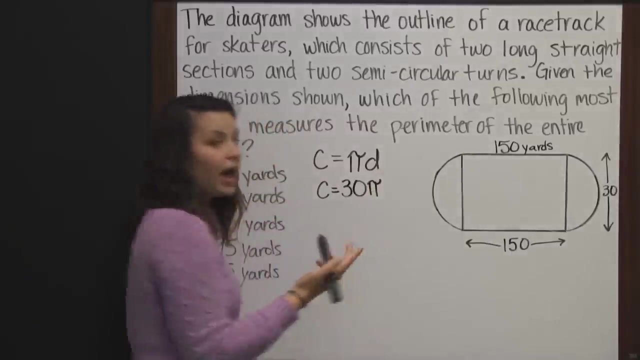 is, And the circumference of a circle is pi times the diameter of the circle which they gave us. They told us that this distance is 30. Well, that goes all the way across my circle. so that's my diameter. So my circumference is 30, pi And pi is about 3.. It's actually 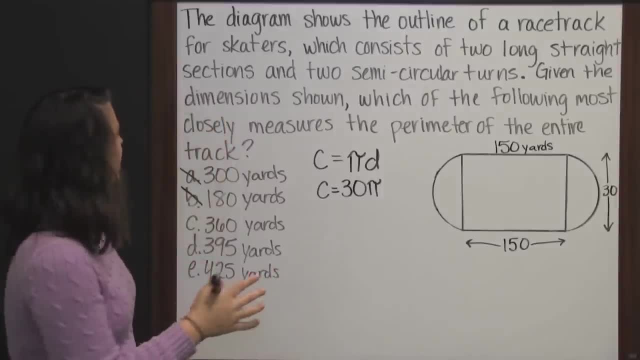 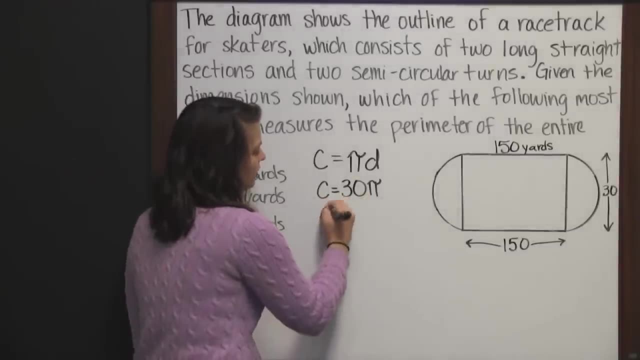 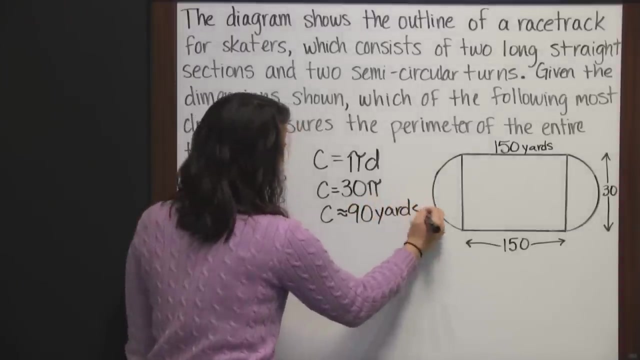 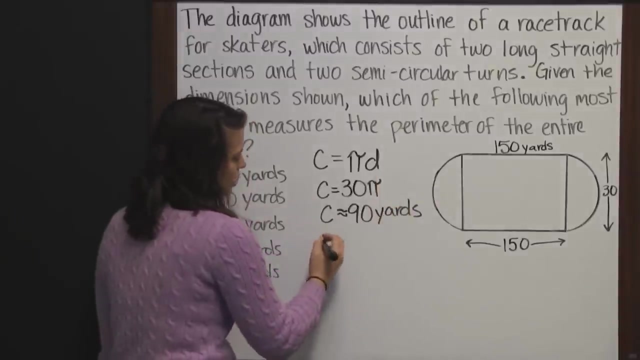 a little over 3, but since they said most closely measures, we'd probably be okay just using 3 for pi. So our circumference is about 90 yards, Plus we have these straight sides, so the total distance around the race track would. 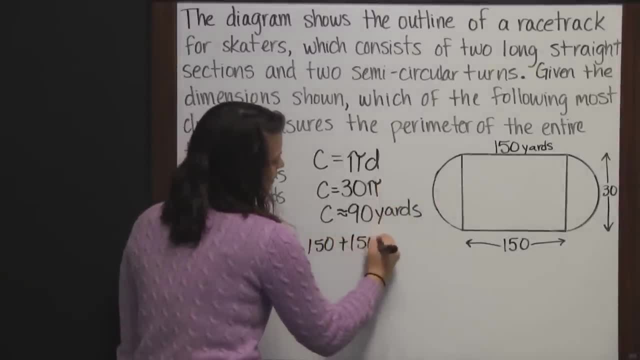 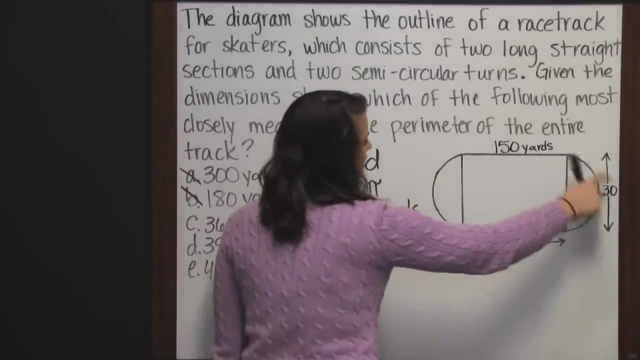 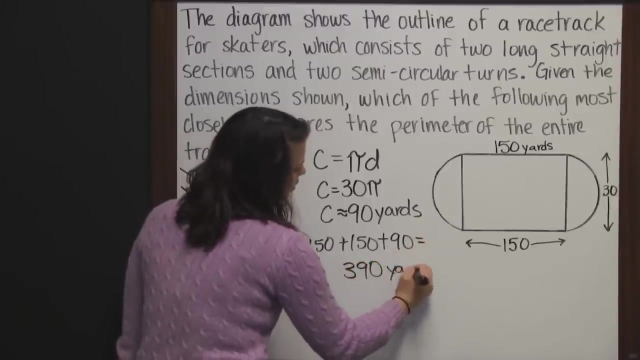 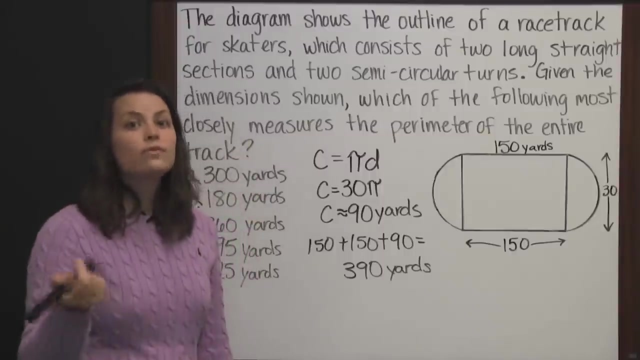 be the 150 yards, plus 150 yards for our two straight sides, plus the about 90 for these two curved sides, the semicircular, which is 390 yards. Now, if you'll remember, we rounded pi down, It's actually over 3.. We rounded it down to 3.. So really, our answer is a little bit higher. 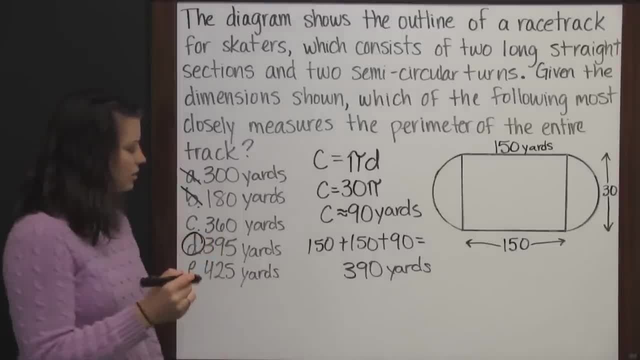 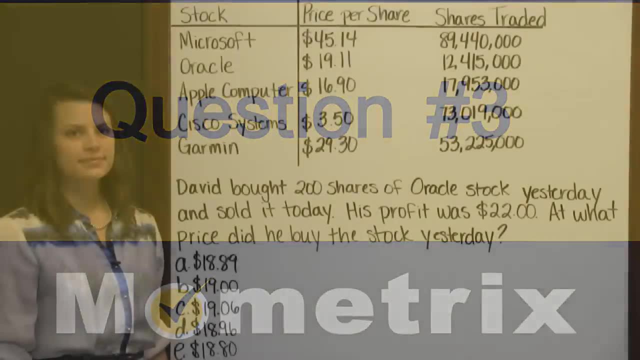 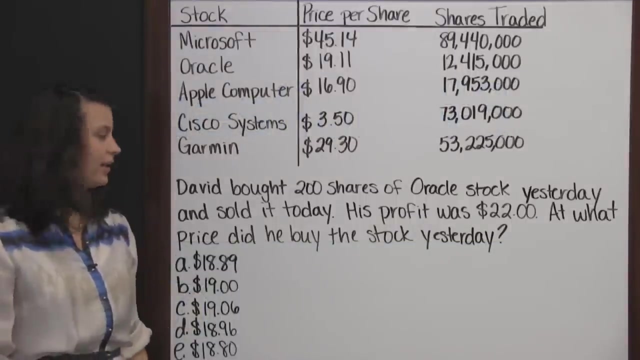 than 390, which is answer choice D: 395 yards. David bought 200 shares of Oracle stock yesterday and sold it today. His profit was $22.. At what price did he buy the stock? He bought the stock yesterday And we have this table of information to use, So we're. 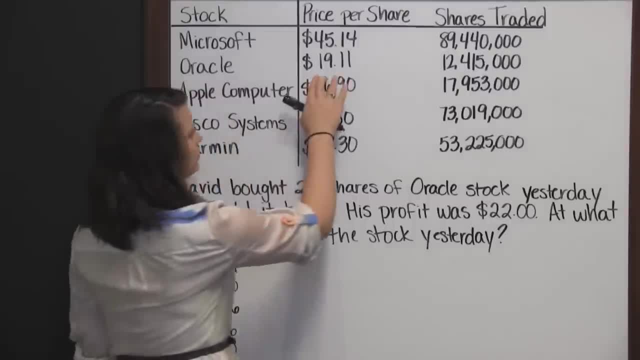 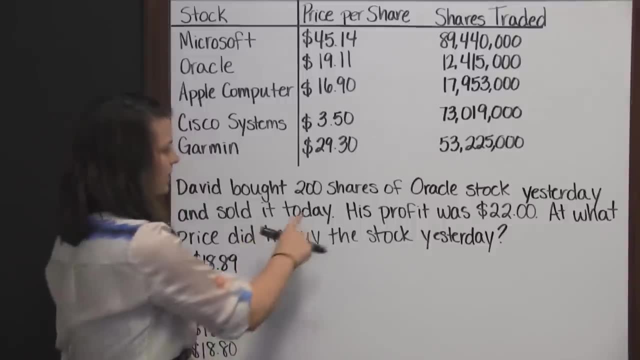 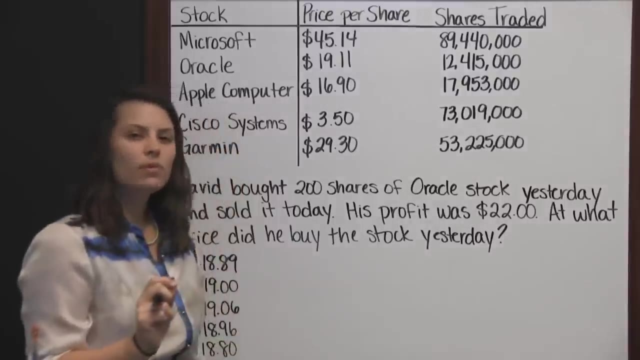 only focusing on Oracle stock, which presently is being sold for $19.11 per share. It tells us that he bought 200 shares and made a profit of $22.. So the first thing we want to do is find out his profit per share, which means we need to divide it up. So we're going to 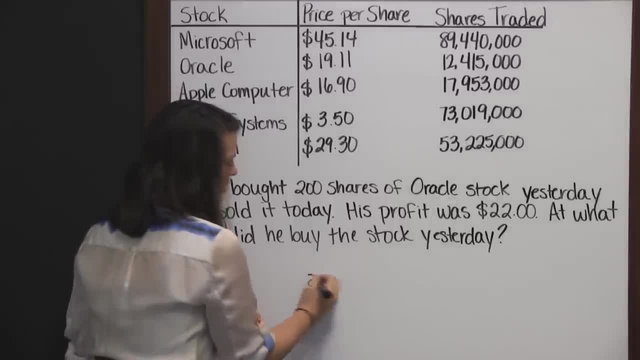 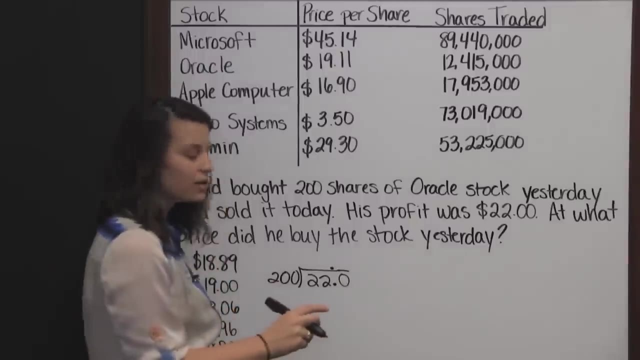 find out his profit per share, which means we need to divide it up. So we're going to divide his profit by his number of shares. 200 does not go into 22,, so I have to add a decimal and a zero. Now 200 will divide into 220.. 200 goes into 220 one time And 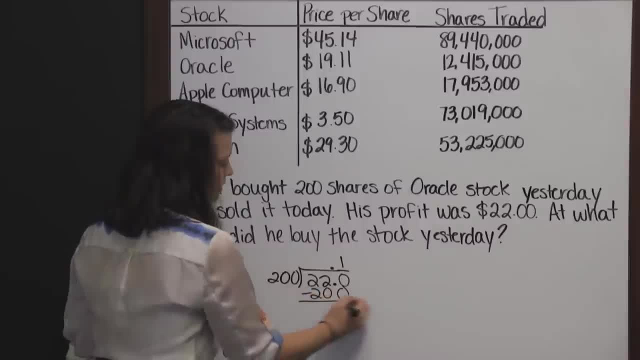 200 times 1 is 200. We subtract and we get 20.. So we add another zero and bring it down. 200 goes into 200 one time. 200 times 1 is 200.. We subtract and we get zero. Now we know that he made 11 cents per share. If today's 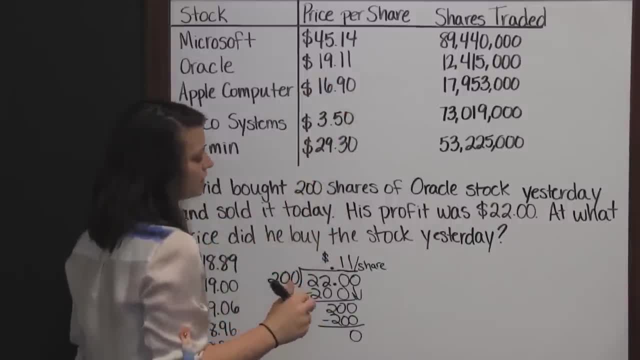 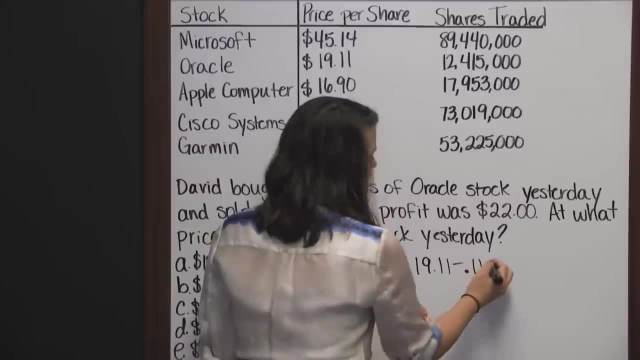 price per share is $19.11, then we have to divide it up, So we're going to divide it in half. At the same time, again, the balance goes up after the other $20 Cookies. At the same time, again, the balance goes up after the other $20 Cookies. So we're going to go. 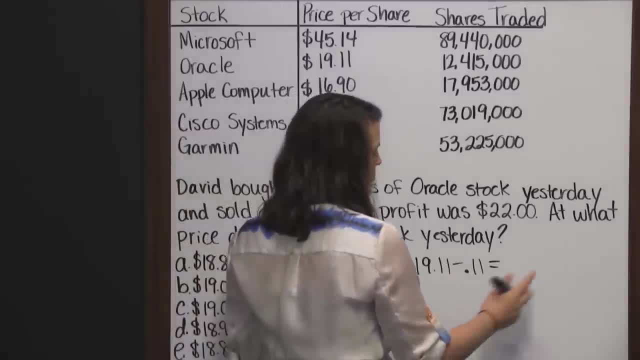 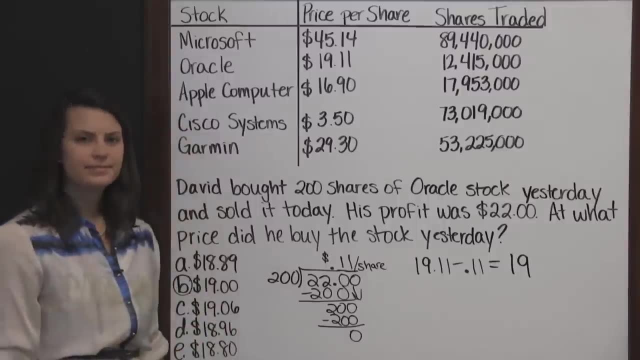 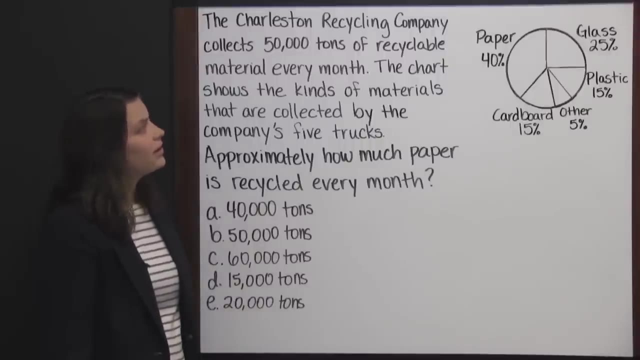 on to number 4.. At the same time again, we're going to divide it up, So we're going to mit our 2 nations. This will also track our total, If at all. it comes down to approximately 130 Cookies. 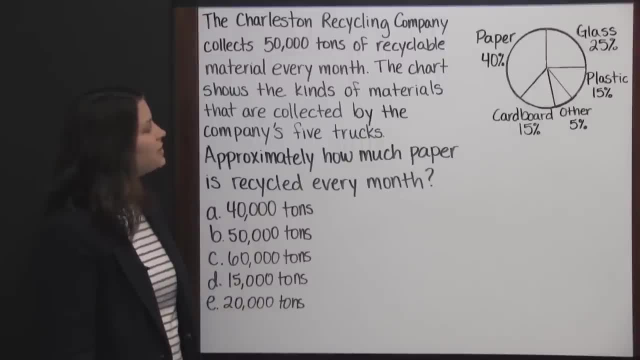 Here in the Great regulating system you have to divide the difference between 22 and 320.. of recyclable material every month. The chart shows the kinds of materials that are collected by the company's five trucks. Approximately how much paper is recycled every month? This: 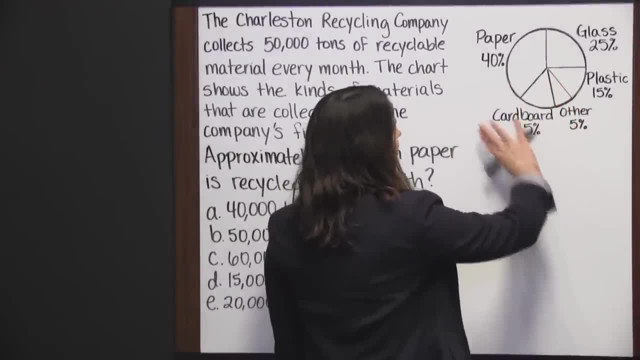 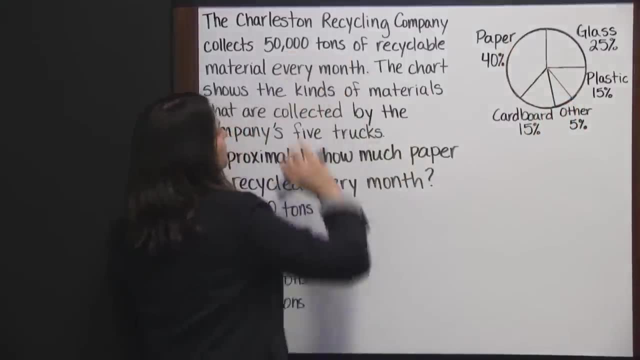 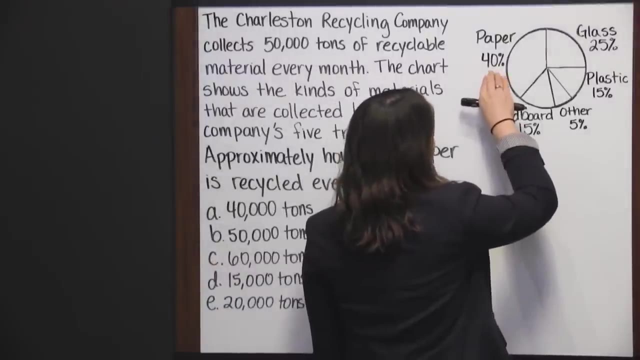 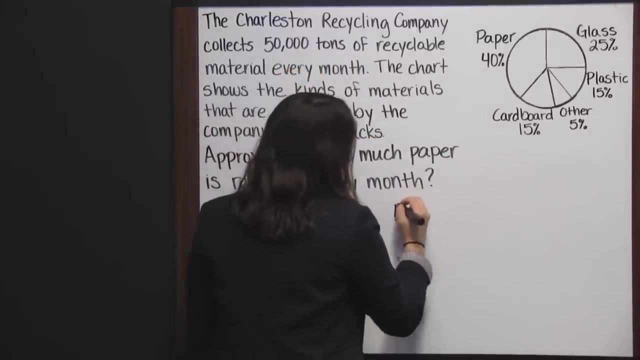 pie chart is a total of 100 percent and it's a total 100 percent of 50,000 tons. So this 40 percent means 40 percent of the total Paper is 40 percent, so 40 percent of the total DONG. 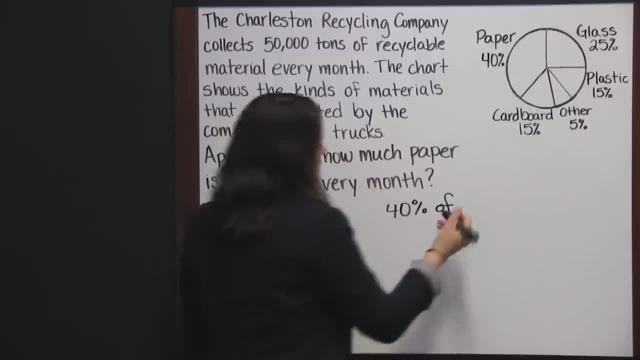 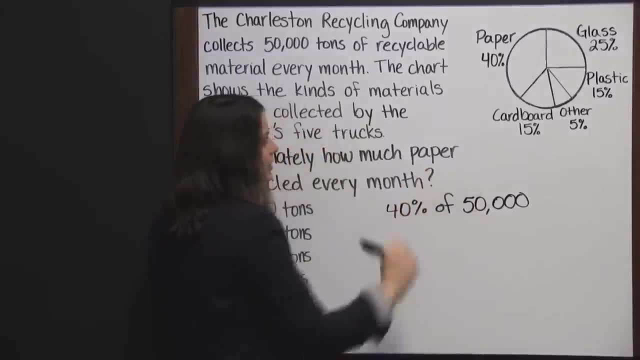 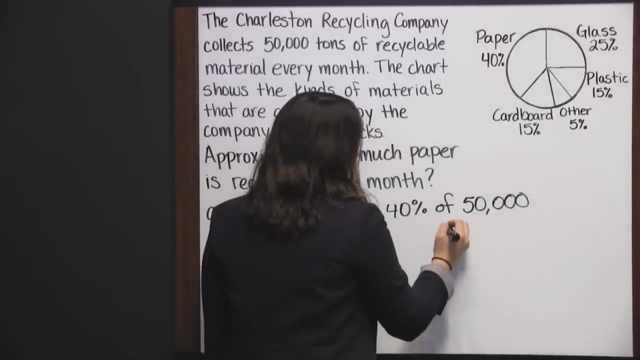 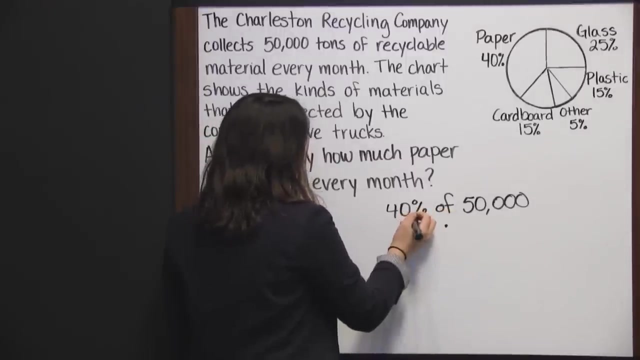 amount of recyclable material collected, or 50,000 tons. 40% of that is paper, and that's what we want to find. is: how much is that? Well, of means to multiply, and I'm going to multiply 40% and 50,000, which means I need to change 40% to a decimal. So move the. 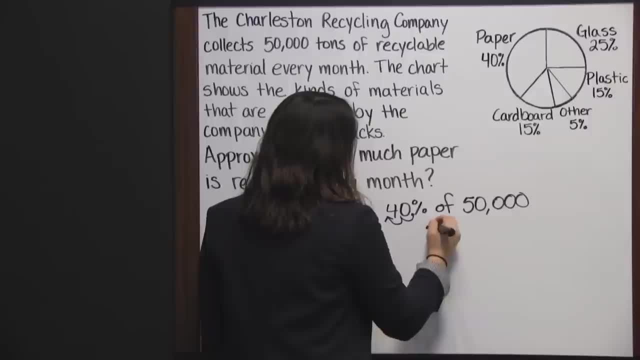 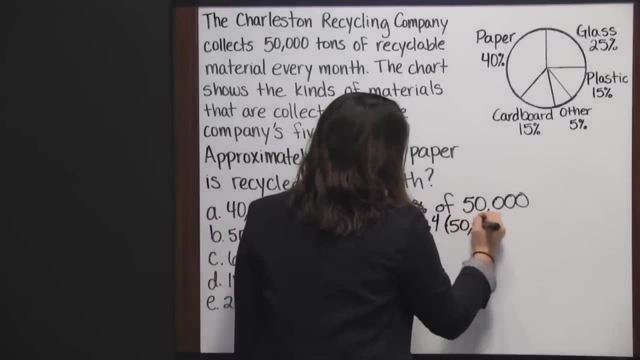 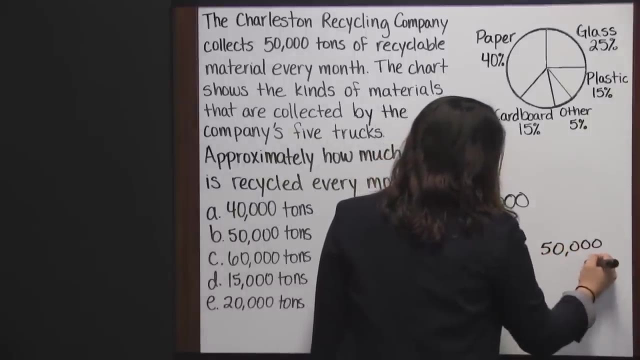 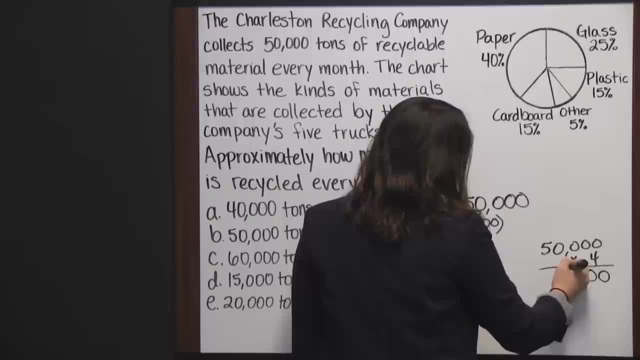 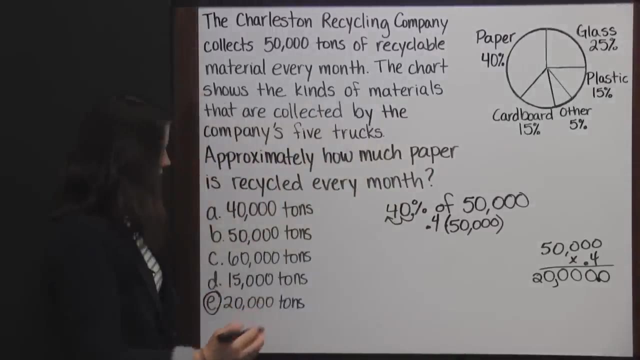 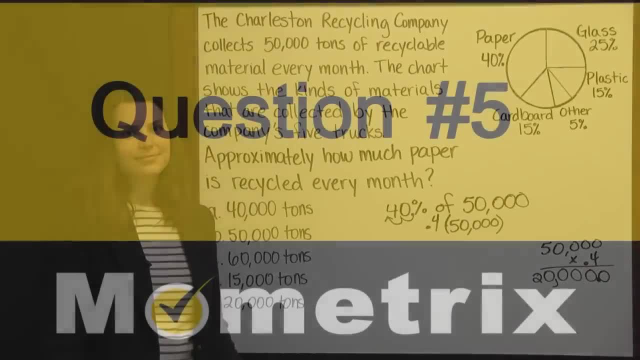 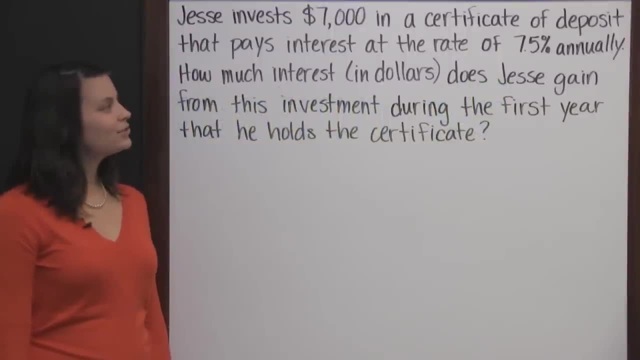 material is paper. Jesse invests 7,000 dollars in a certificate of deposit that pays interest at the rate of 7 and a half percent annually. How much interest in dollars does Jesse gain from this investment during the first year that he holds the certificate? This is a great problem to 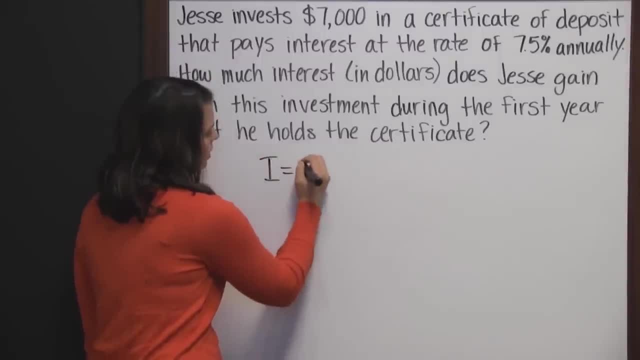 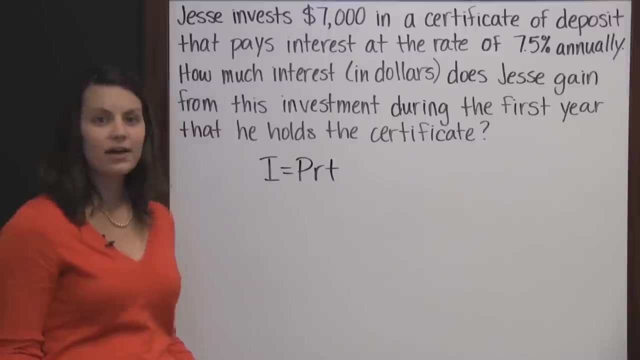 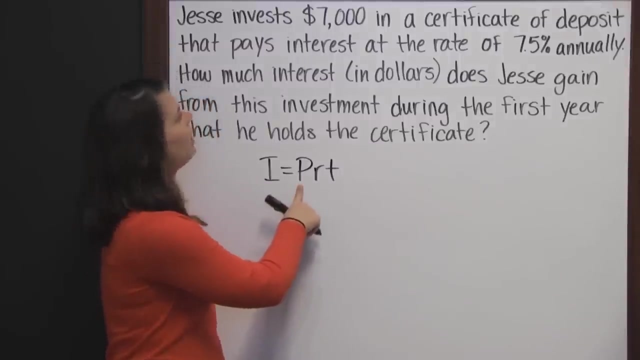 use this formula on, And some people call it IPERT just as a way to remember it. The I stands for the interest, The amount of interest in dollars, like what we're trying to find. P stands for principal, or the amount that's being invested initially. That would be our 7,000 dollars. The R is 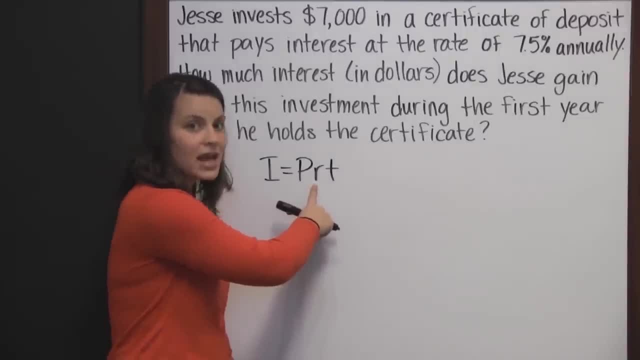 the rate or the percentage, but written as a decimal. So we're going to take 7 and a half percent and write it as a decimal. That'll be our rate, And then T stands for time, So you may want to make a note of that. This: I is the interest, P is the principal, R is 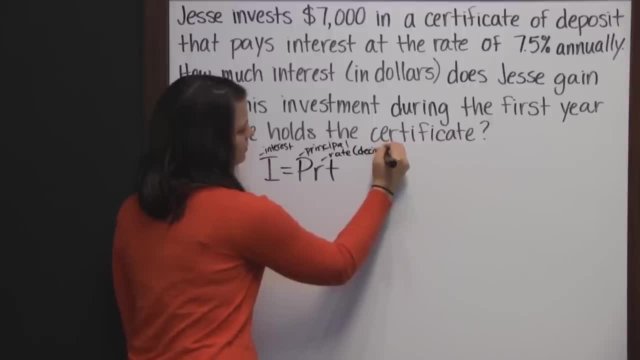 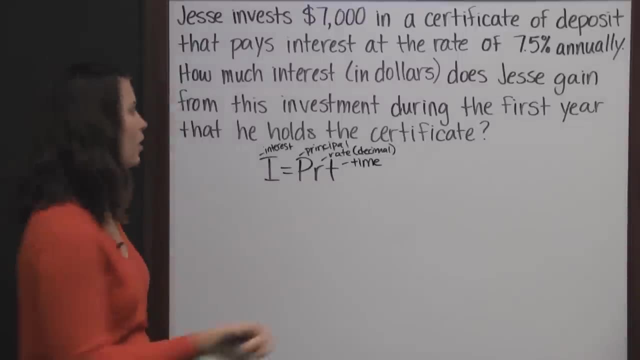 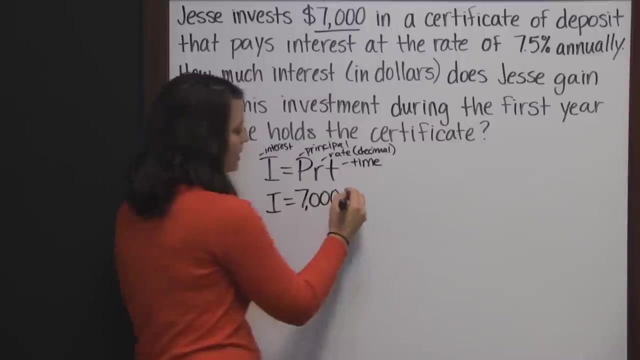 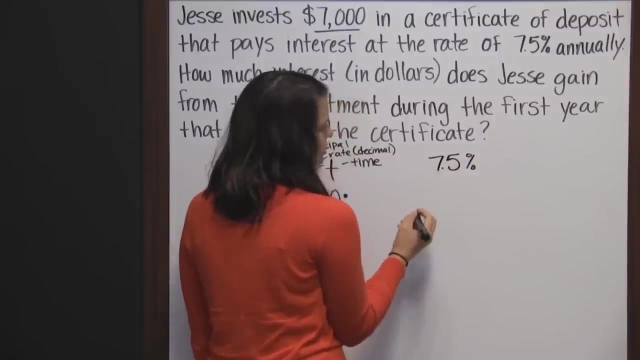 the rate as a decimal and the T is the time. So we're going to take our information from our problem and plug it in. So our amount of interest is equal to the principal 7,000 dollars times the rate as a decimal again. So we're taking 7 and a half percent and changing it. 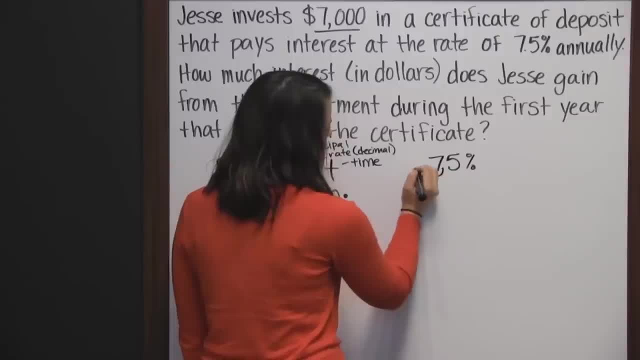 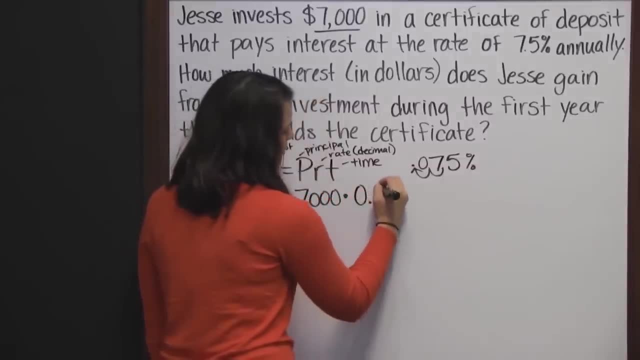 to a decimal, which means taking the decimal and moving it two places to the left. So you add that zero, so it's seventy-five thousandths, and then times the year or the times. the year times the time, and we're just trying to find out about the first year. So that means 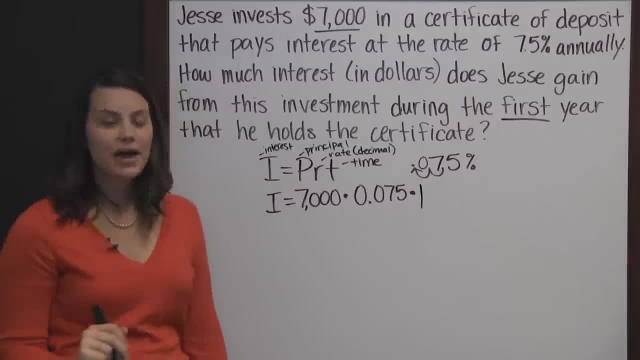 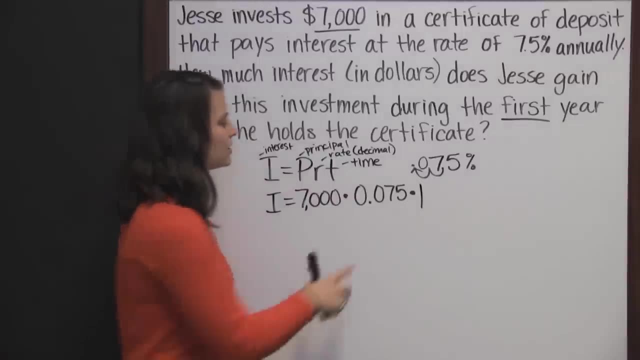 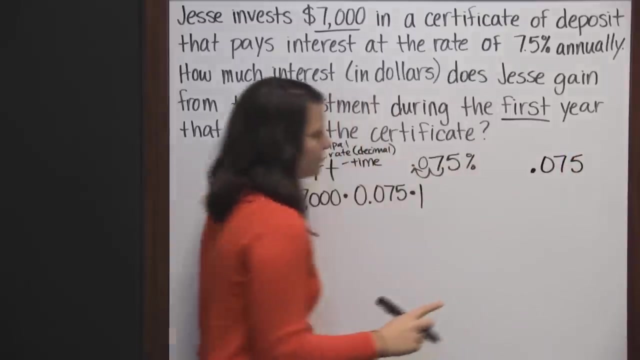 it's been in there for one year, And then we just need to multiply those things together, So one times anything is just that. so I can really kind of ignore that. So I just need to multiply these two numbers together, So I have this seventy-five thousandths, and 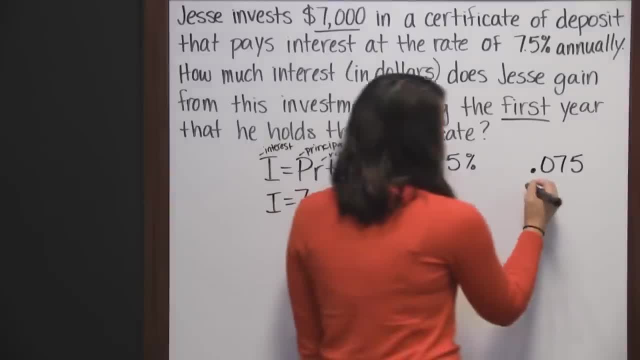 I'm going to put it on top because it's very easy to multiply times 7,000, since the first thing I'm going to do is just write down those three zeros And then the only number I really have to multiply by is the seven. So the seven times five is thirty-five. Write the five. 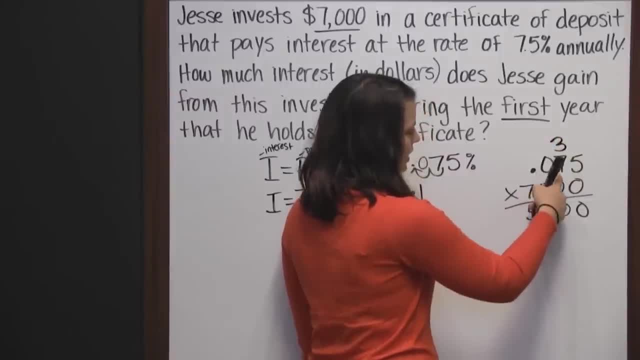 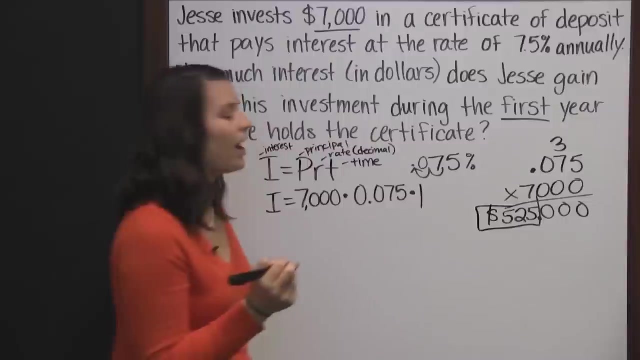 carry the three, Seven times seven is forty-nine plus three is fifty-two. And then we have three numbers behind the decimal. so three numbers behind the decimal. And that means that he's going to make five hundred twenty-five thousandths. So he's going to make five dollars off of his investment. So that's the number you would. 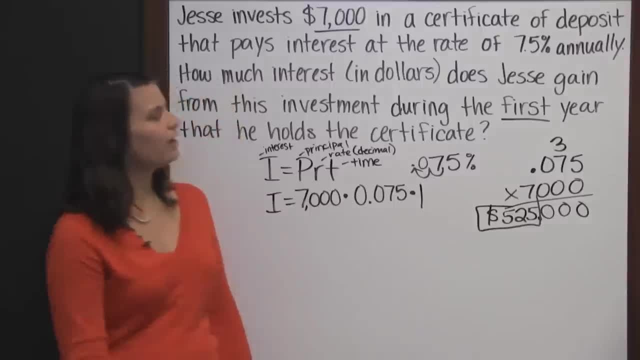 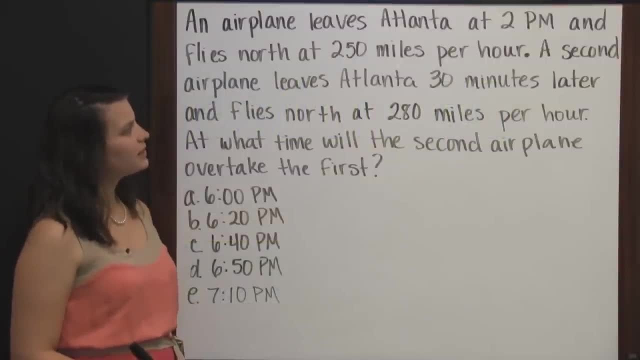 need to bubble in is five-two-five. An airplane leaves Atlanta at 2 pm and flies north at 250 miles per hour. A second airplane leaves Atlanta thirty minutes later and flies north at 280 miles per hour. At what time does an airplane leave Atlanta? At 2 pm and flies north at 280 miles per hour? 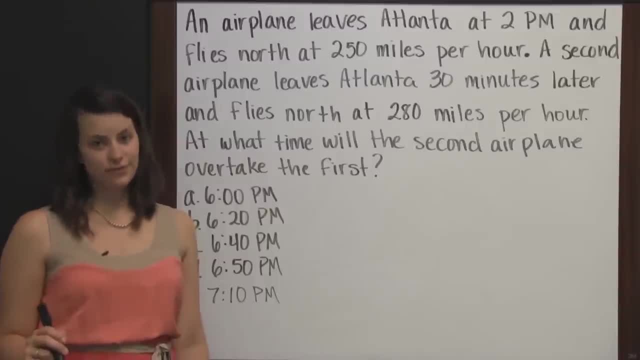 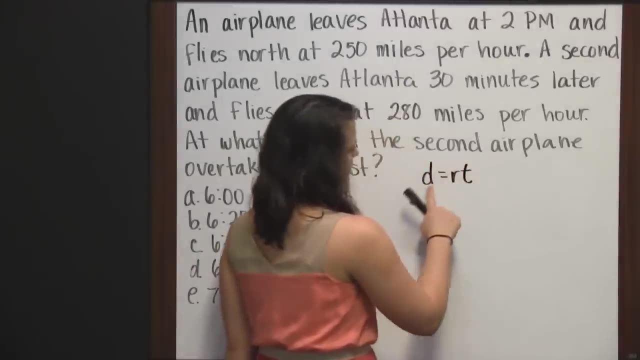 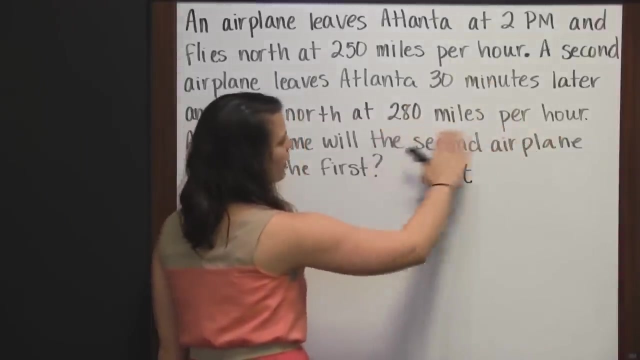 At what time does an airplane leave Atlanta? At 2 pm and flies north at 280 miles per hour? At what time will the second airplane overtake the first? Well, this is a dirt problem. where distance equals rate times time. You see, we've got time. thirty minutes later, We've got rate. 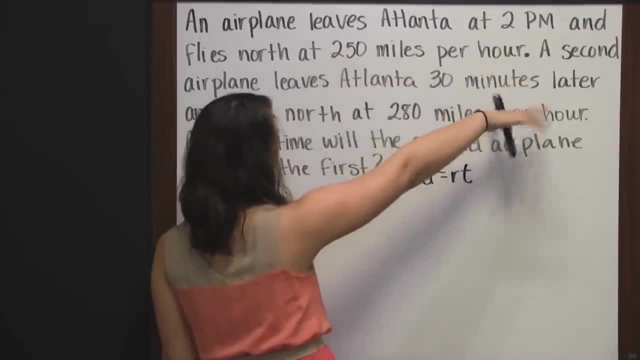 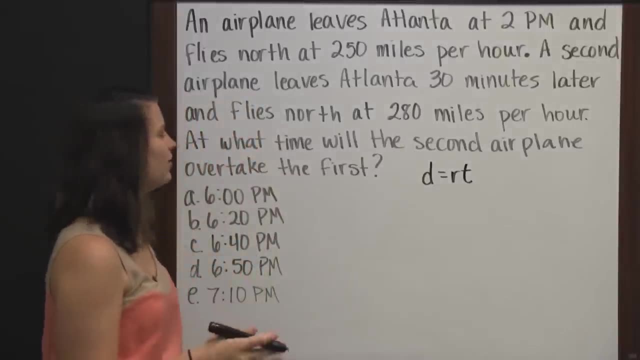 280 miles per hour. 250 miles per hour. We've got distance here, because both these planes are flying a distance and that's how their rate and time are related, So we need to use this formula to help us organize our data. 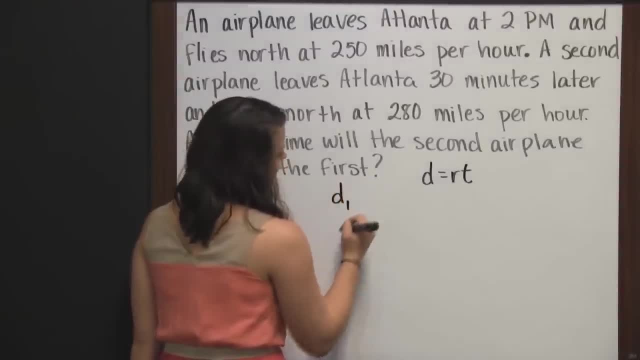 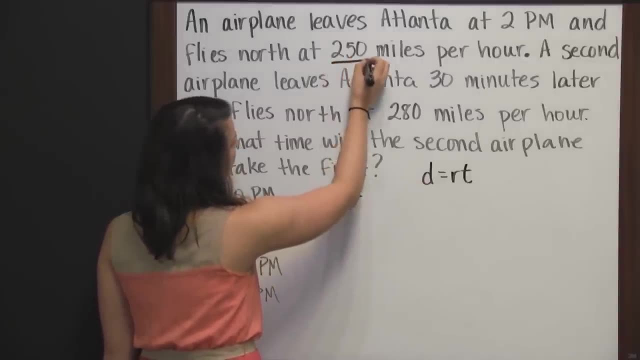 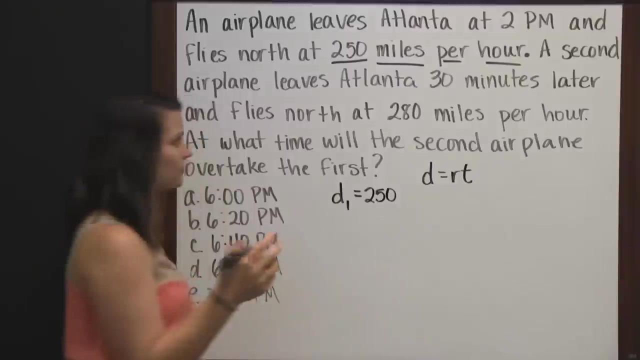 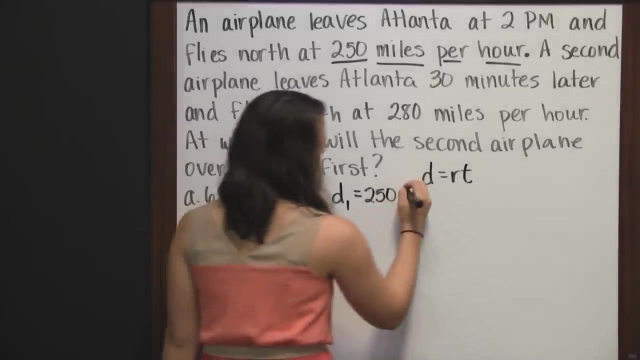 So first let's find the distance for the first airplane. The rate of the first airplane is 250 miles per hour, So 250 times. and then all we know is what time the first airplane left. We don't know how long that airplane flew, So we've got to use t for time there. 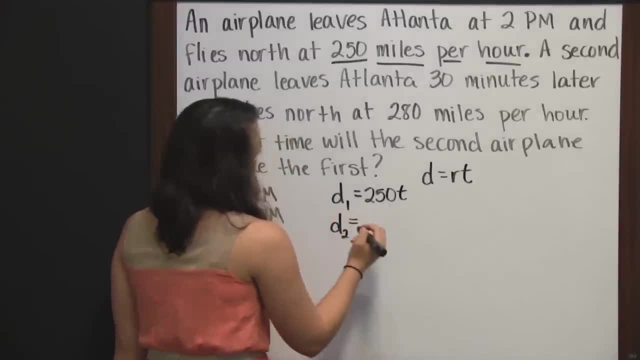 Now the distance for the second airplane. the rate is 280 miles per hour and we do know a little bit about the time that the second airplane flew. If you'll notice, the second airplane is going faster than the first one, So if they left from the same place. 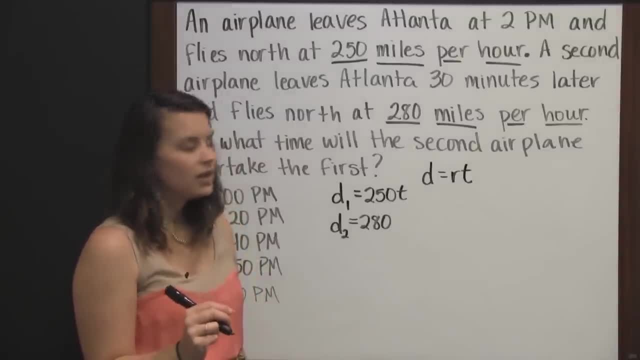 and they go in the same direction, they're going to fly north at 280 miles per hour. So if they left from the same place and they go in the same direction, they're both going north. then the second airplane is eventually going to catch up with the first. 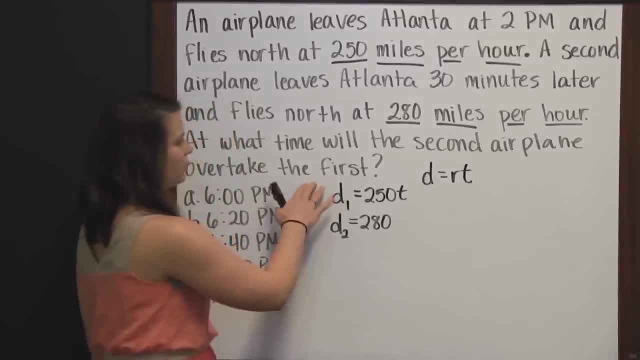 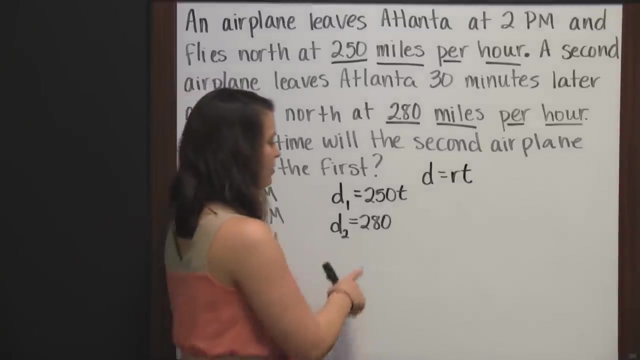 and actually pass the first. And that's what we're trying to figure out is: at what time will the second airplane catch up to or overtake the first? So the second airplane won't have been flying as long as the first airplane. when it catches up, It's going faster and 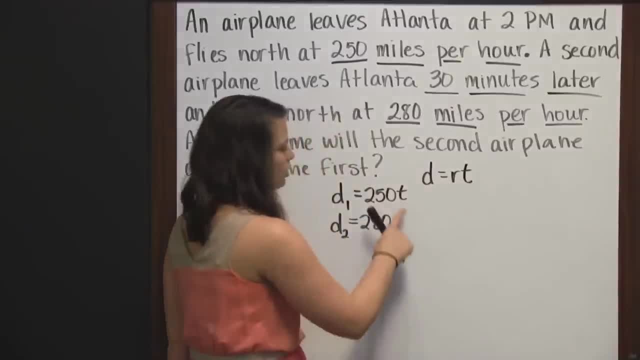 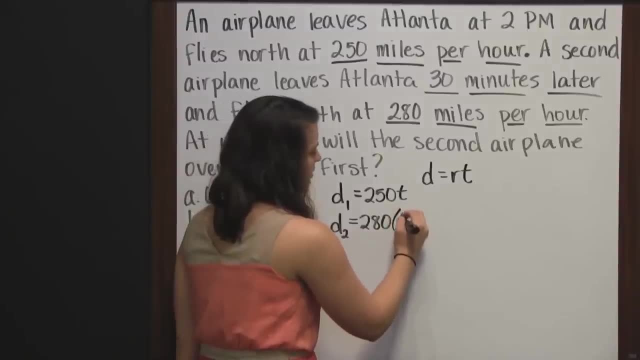 it left 30 minutes later. So however long the first airplane flew, we know that the second airplane left 30 minutes later. So however long this first airplane has been flying, the second one will have been flying that time minus 30 minutes, since it left 30 minutes later. 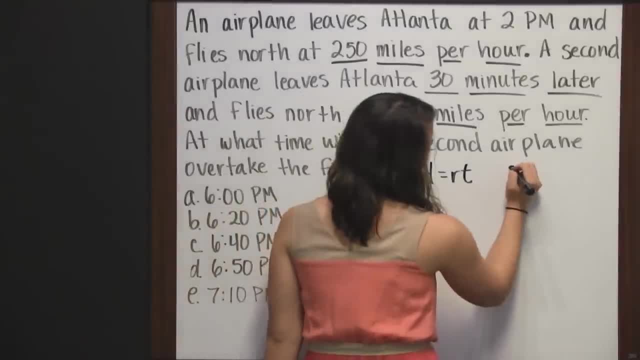 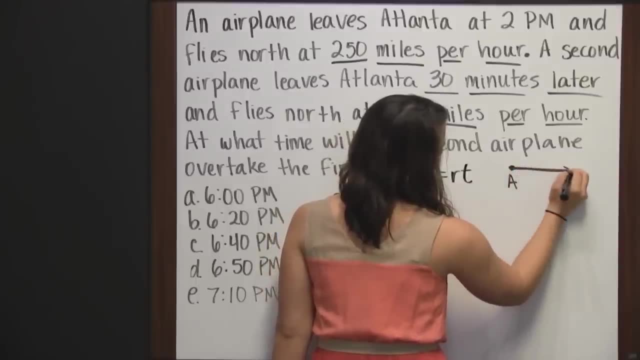 Now, if you think about this, you've got two planes leaving from Atlanta. They're both flying north, and the question is: when will the second one overtake the first one? Well, this is what we're trying to find out is what time that will happen. Well, at that. 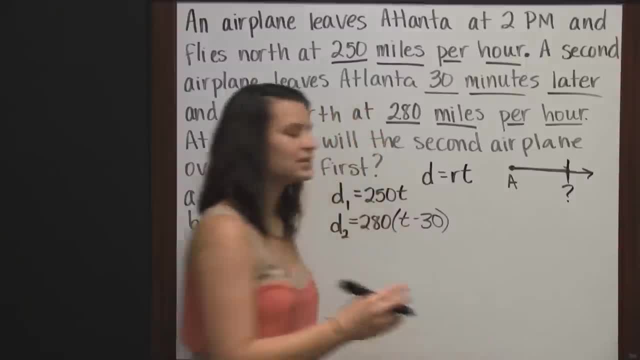 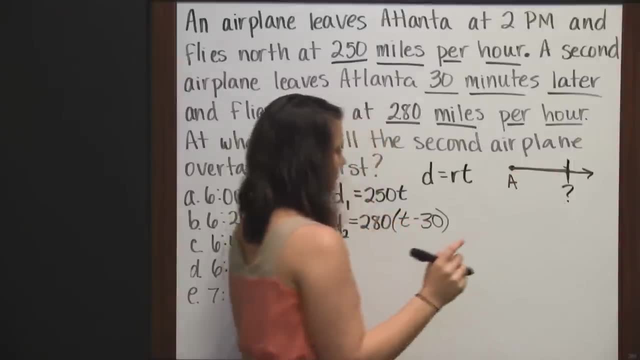 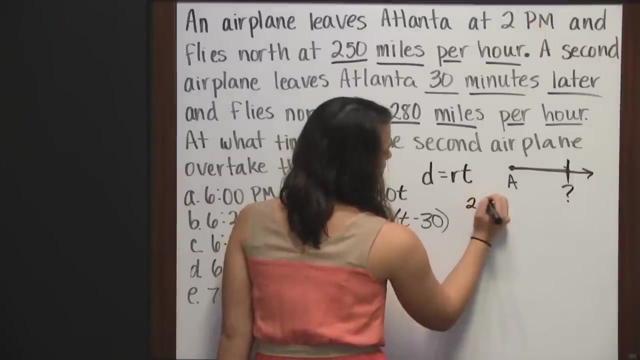 time, both of these airplanes will have flown the exact same distance. We don't know what that distance is, but we know that it's the same, So we can take these two distances and we can set them equal. So the distance of plane 1, 250t is equal to the distance. 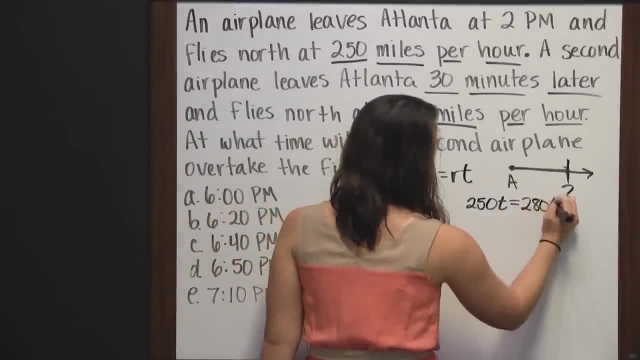 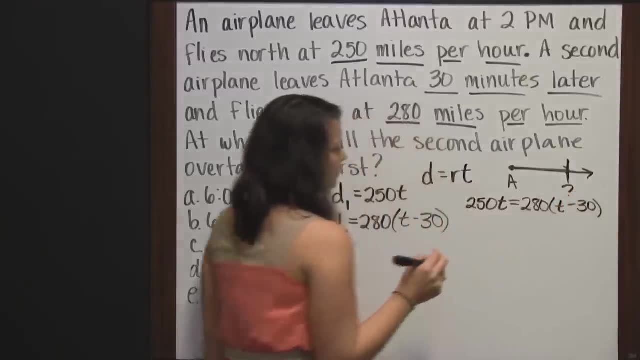 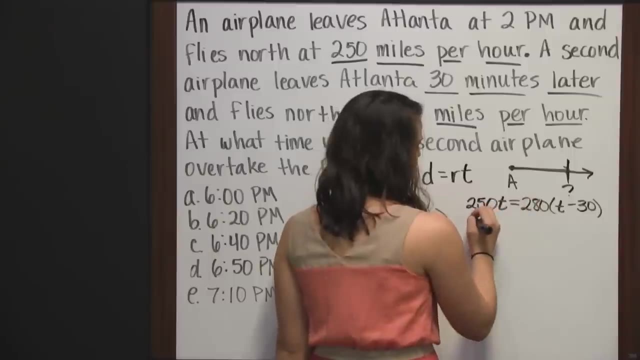 of plane 2.. 280 times the quantity t minus 30.. And now we need to solve for t. So the first thing we want to do is distribute our 280.. So I'm going to bring down this: 250t equals 280. 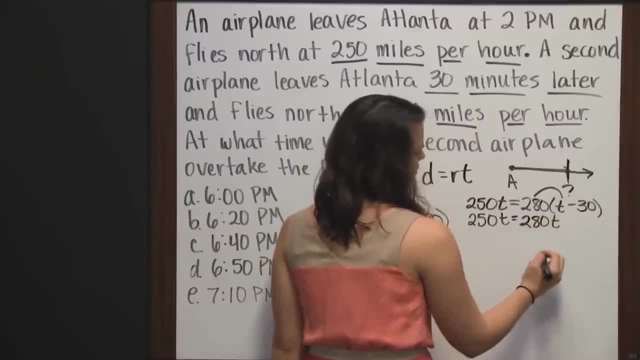 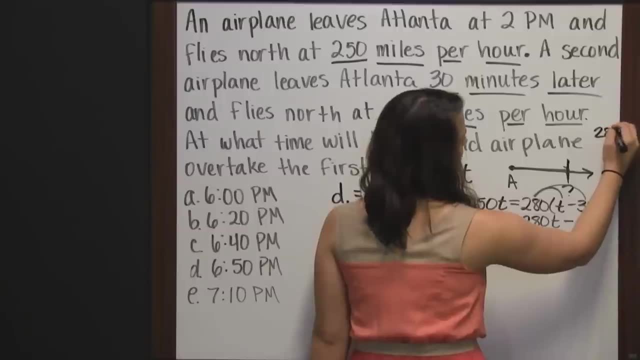 times t: 280t minus 280 times 30.. 280 times 30,: 0. placeholder. 3 times 0 is 0,. 3 times 8 is 24,. 3 times 2 is 6, plus 2 is. 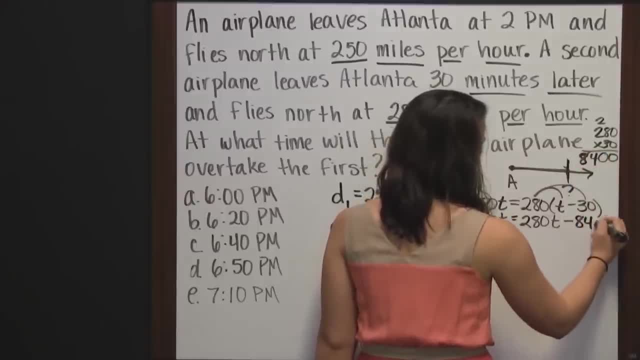 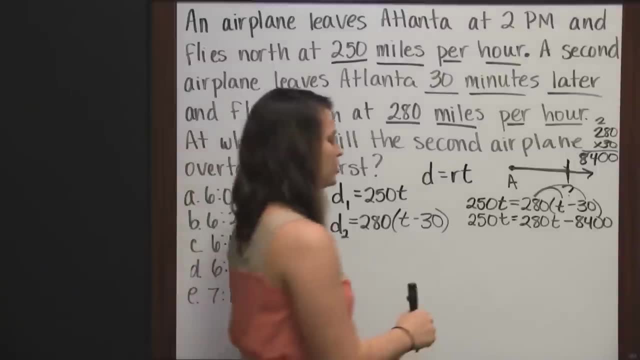 8. That's 8,400.. Now we need to get all of our variables on the same side of the equation. We don't want to have t on the left side and t on the right side, So I'm going to subtract. 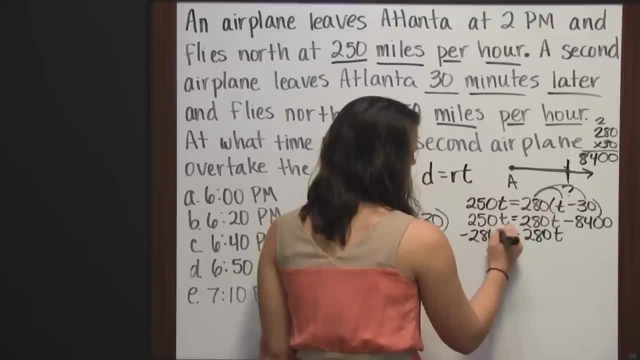 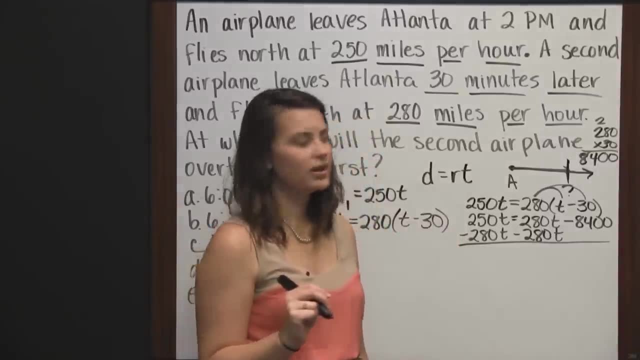 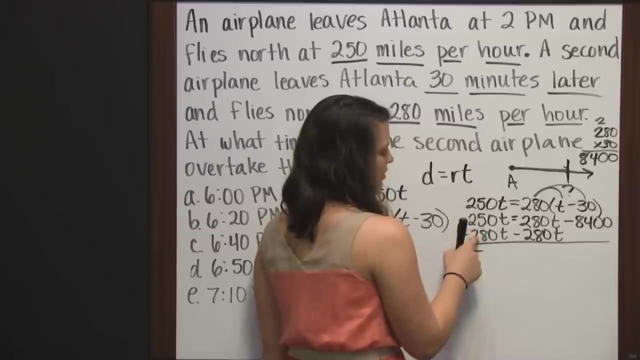 280t from both sides, 250t minus 280t. I'm taking away more than I have. So I'm going to end up with a negative, And the difference between 280t and 250t is 30t, So negative 30t equals- I'm subtracting. 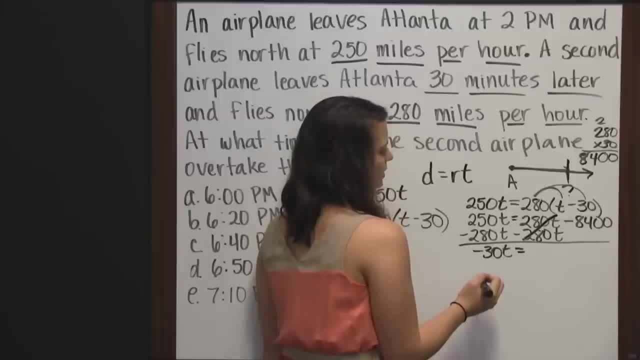 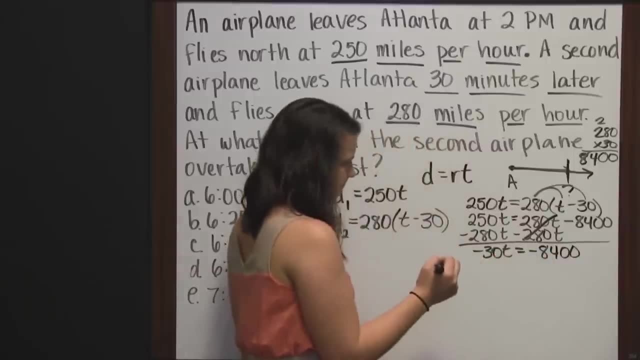 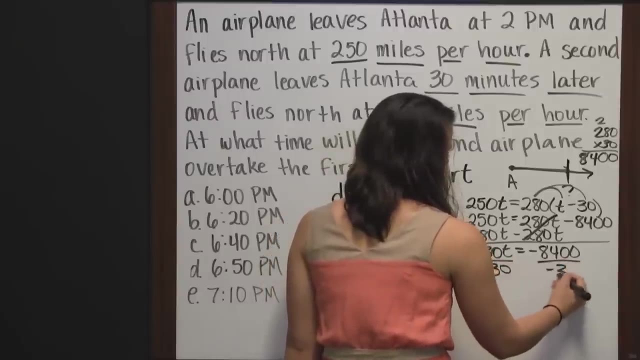 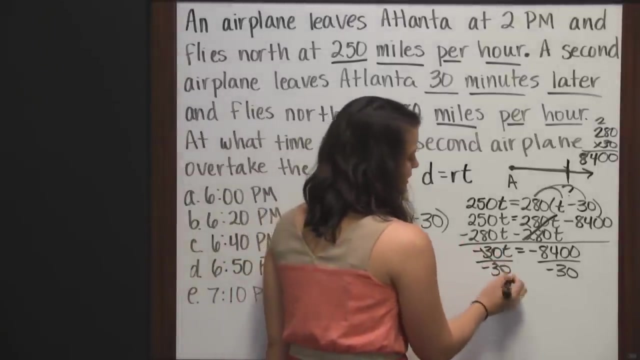 this 280t. I've actually cancelled that term on the right side and I'm left with negative 8,400.. To solve for t then we need to divide both sides by negative 30.. Negative 30 divided by negative 30 is 1, times t, is simply t. 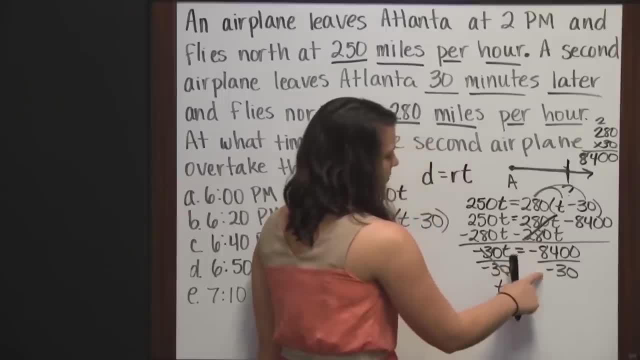 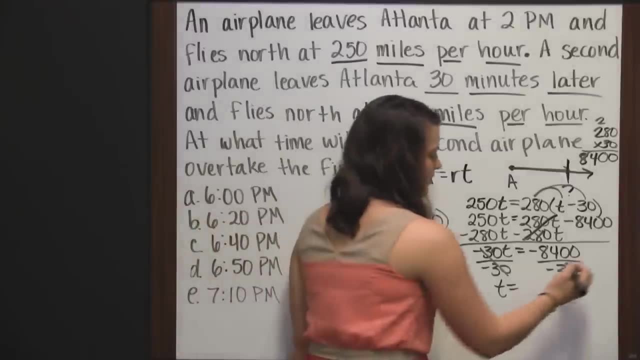 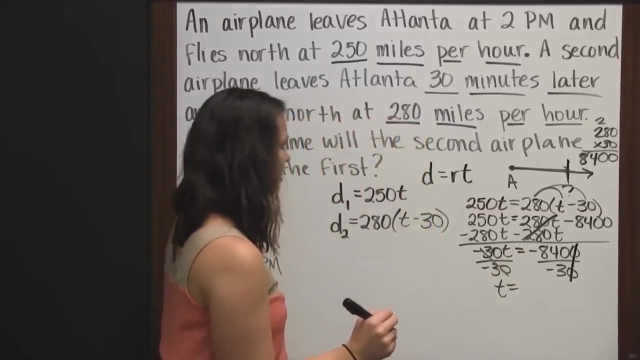 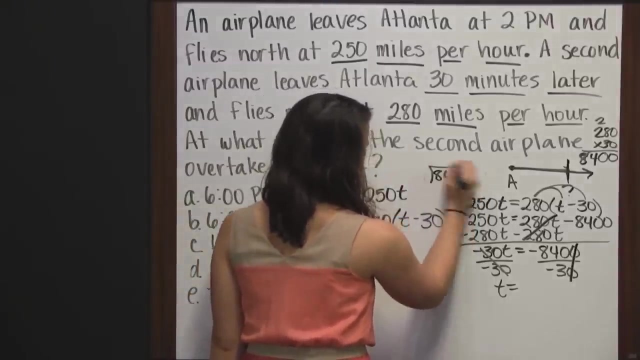 Negative: 8,400 divided by negative: 30,. first of all, a negative divided by a negative is a positive. Then we can cancel a 0, and really all we have to do is divide 840 by 3.. Really, I'm running out of space here. I'm going to get rid of this, so we can divide 840 by 3.. 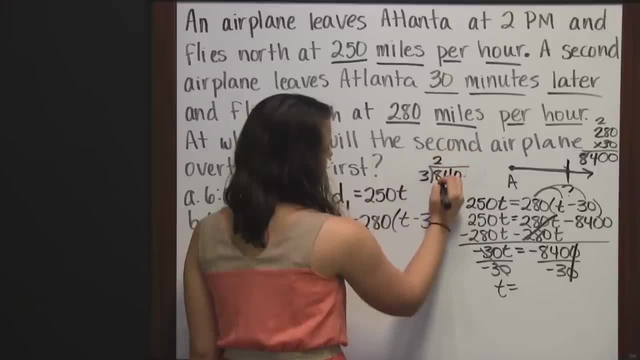 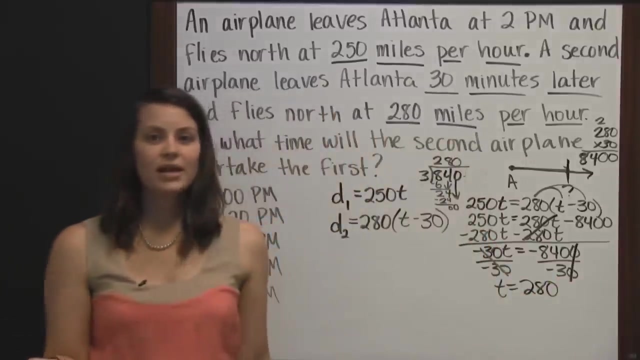 3 goes into 8 two times, That's 6.. Subtract and you get 2, bring down the 4,, 3 goes into 24, 8 times. 3 times 8 is 24.. Subtract and you get 0,. bring down your 0, 3 goes into 0, 0 times, so it's 280, but 280 what? 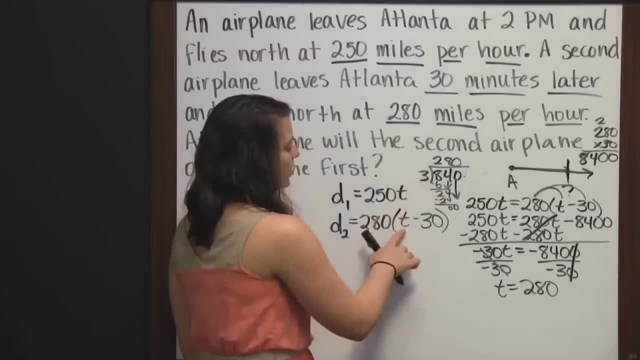 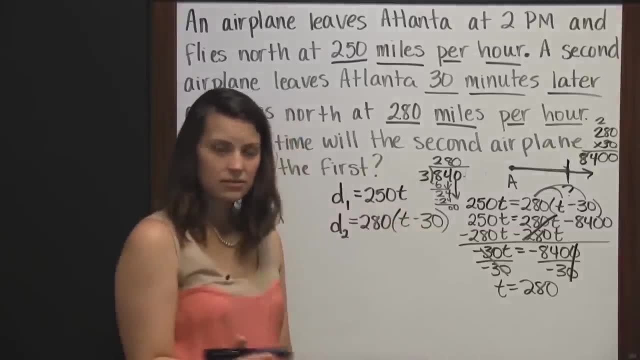 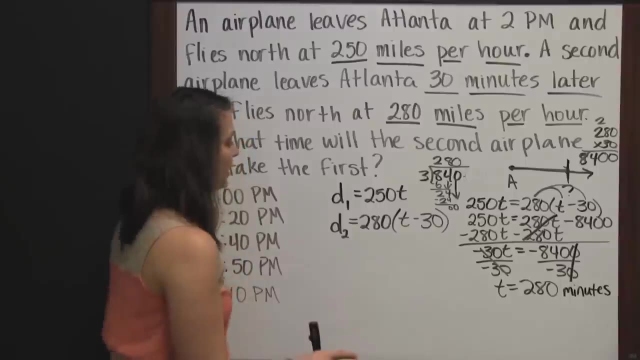 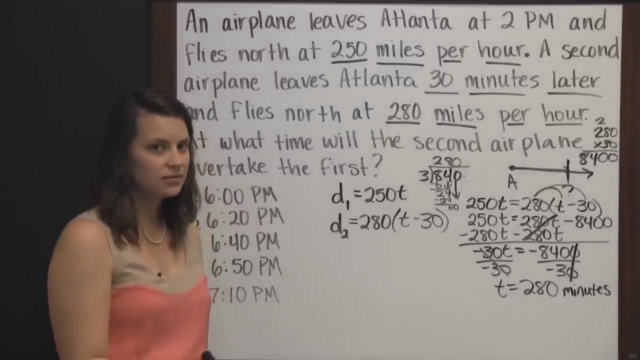 Well, if you'll recall, we did t minus 30 minutes. That would mean that these t's are in minutes, so we just found how many minutes the first plane t- the first plane- would have been flying when the second plane overtook it. 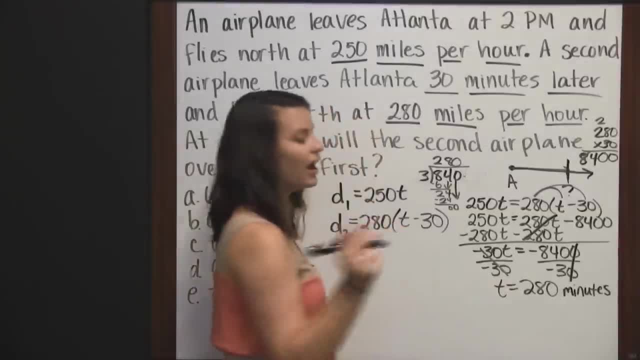 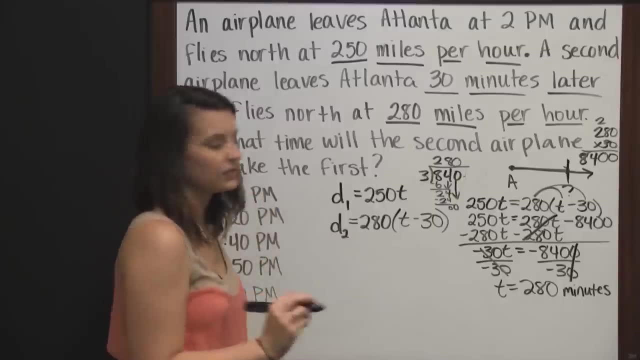 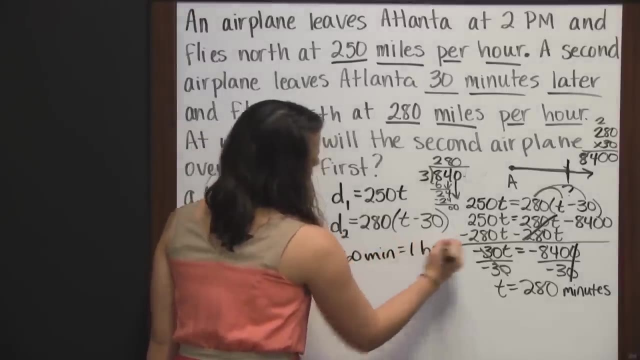 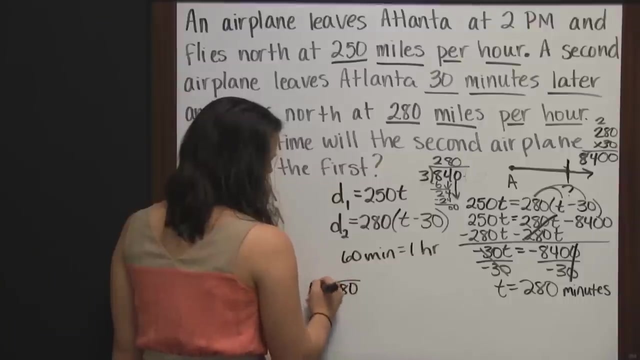 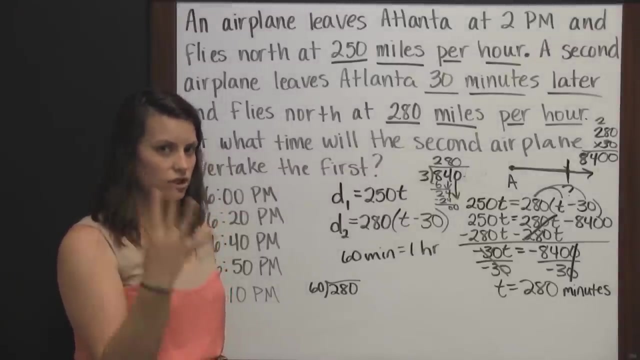 We need to first convert these minutes into hours and minutes so that we can then find the time. what time it will be. flying was when that happened. To convert these minutes into hours, there are 60 minutes in one hour, which means we need to divide 280 by 60. We've got 60, 120, 180, 240.. 60 goes. 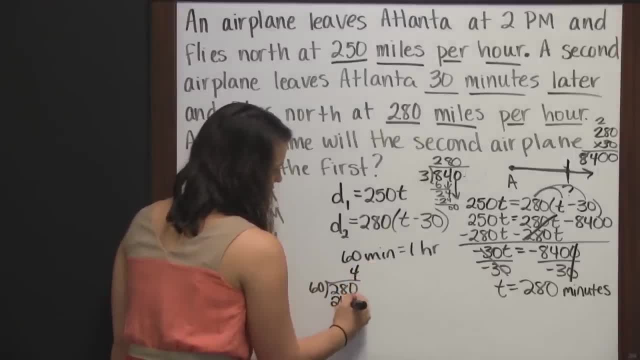 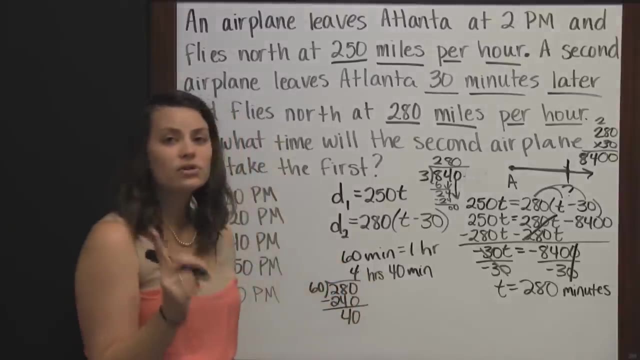 into 280 four times and you get 240.. You subtract and you get a remainder of 40 minutes. That's 4 hours 40 minutes. 4 hours 40 minutes after the first plane left at 2 pm is when the 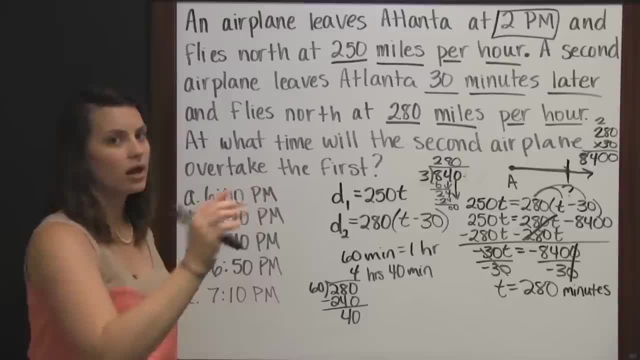 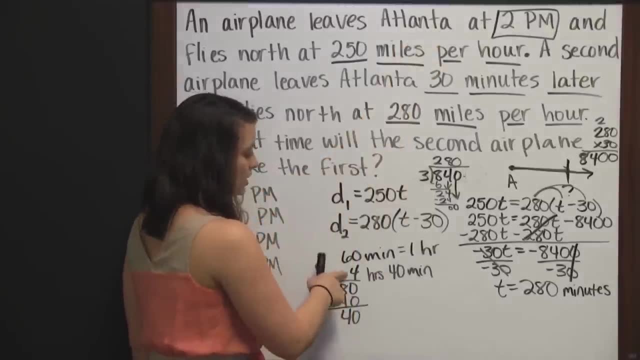 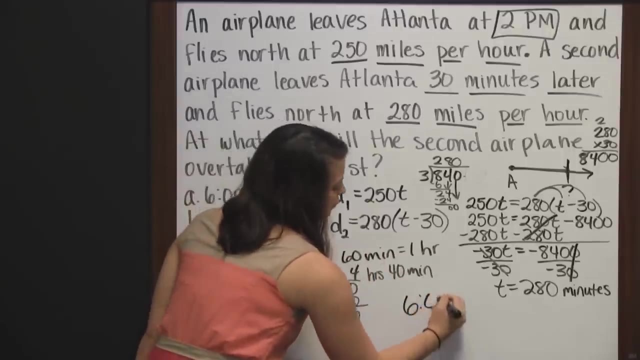 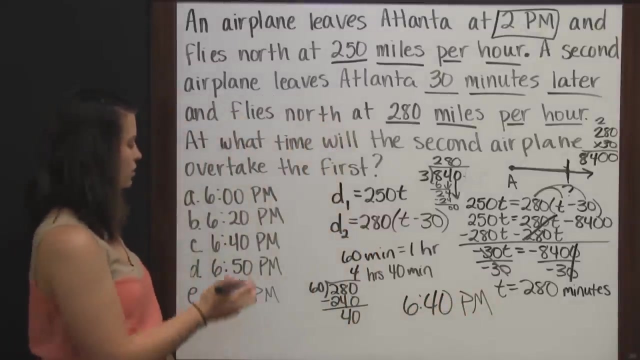 second plane overtook it or caught up with it Or had traveled the same distance. So 2 plus 4 hours is 6 and 40 minutes. So at 6.40 pm is when that second plane overtook the first Answer C. 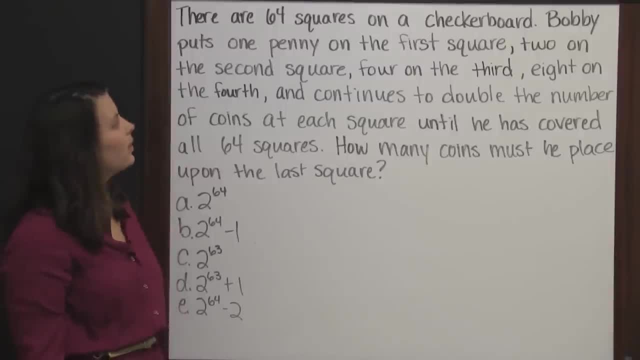 There are 64 squares. There are 64 squares. on a checkerboard, Bobby puts one penny on the first square, two on the second square, four on the third, eight on the fourth, and continues to double the number of coins at each square until he has covered all 64 squares. How many coins must? 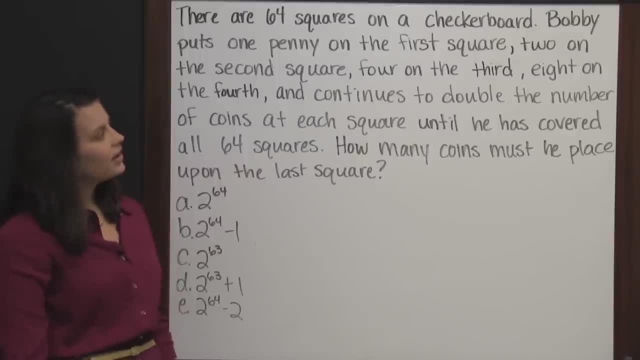 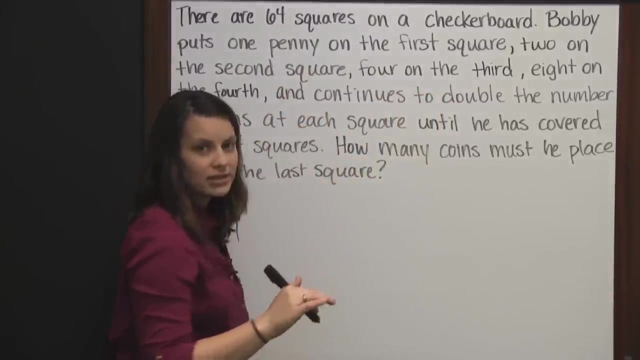 he place upon the last square. The first thing I want to do is take this information out and organize it. So I've got two pieces of information here. I've got these number of squares and also how many coins are on the squares. So I'm going to organize. 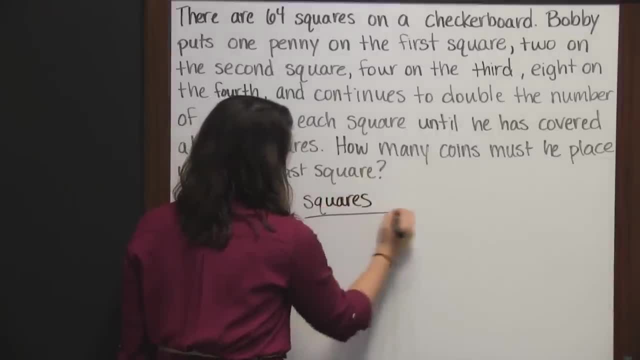 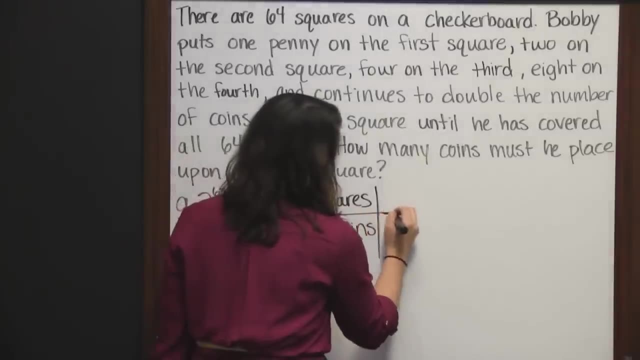 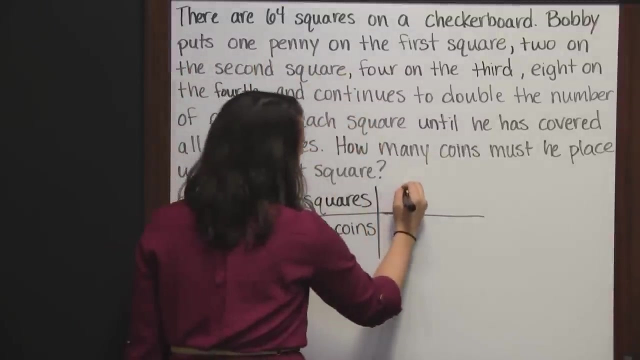 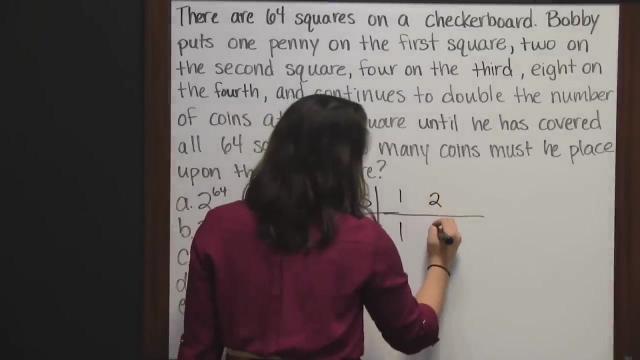 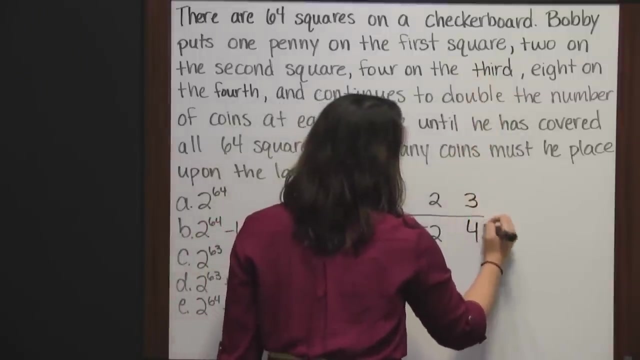 it as squares and number of coins. So it says he puts one penny on the first square, two penny on the first square, so square one, one, penny Two on the second square, second square: two pennies, Four pennies on the third square. so third square, four pennies Eight. 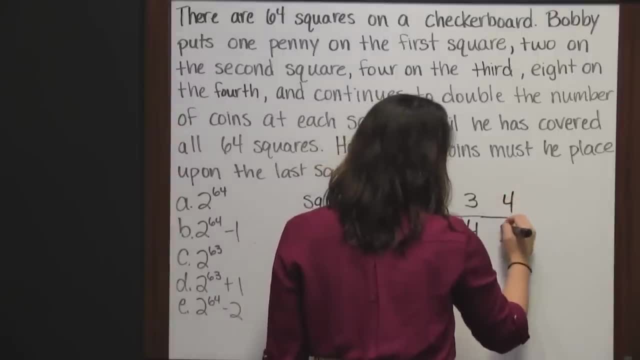 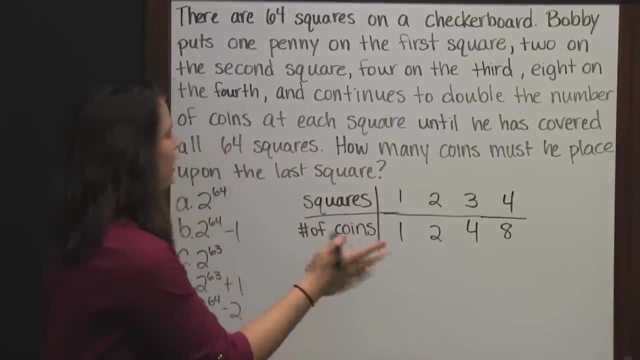 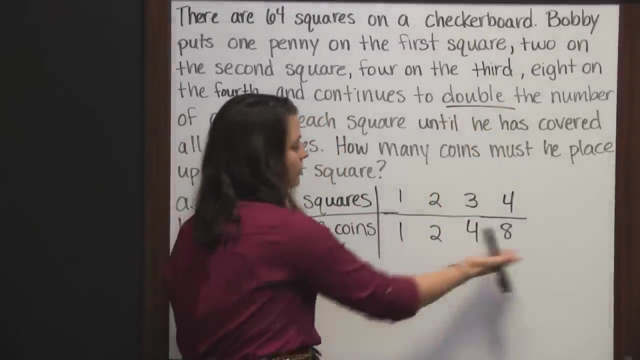 on the fourth square. so fourth square, eight pennies and so on. like that, It keeps doubling. Another important word here is double. Really, we don't even have to find the pattern. They told us what it was. We're doubling. This is one times two is two times two is four. 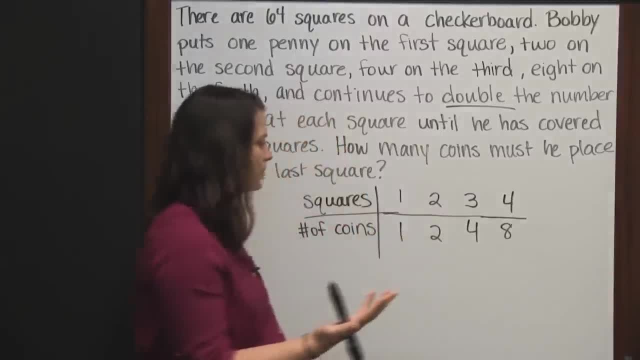 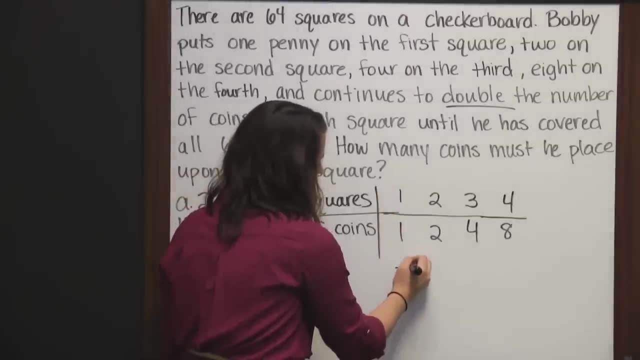 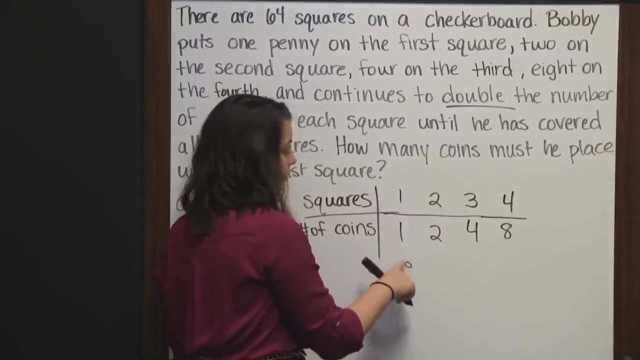 times two is eight. Since I know I'm doubling, then I have a base of two. On the first square, I have two to the power of zero. Any number to zero is one. On my first square, I have 2 to the power of 0 coins. On my second square, I have 2 to the first power coins, 2 to the. 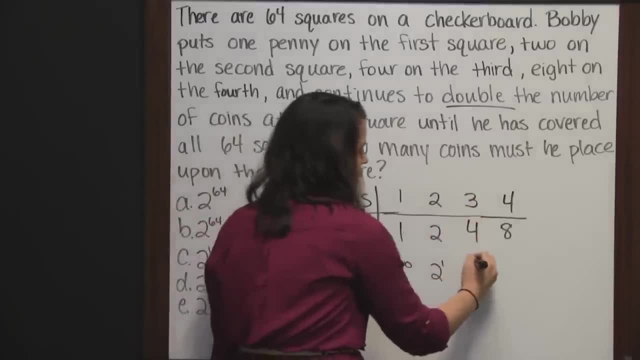 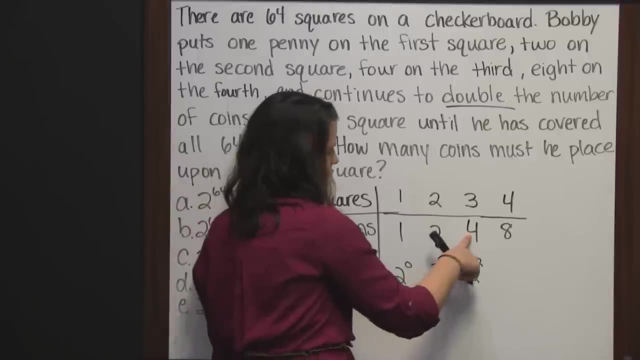 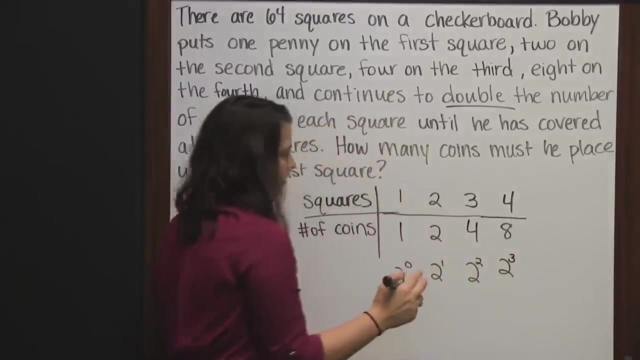 first power is 2.. On my third square I have 2 squared coins. 2 squared is 4.. On the fourth square I have 2 cubed coins. 2 times 2 times 2 is 8.. As you can see, as we increase our 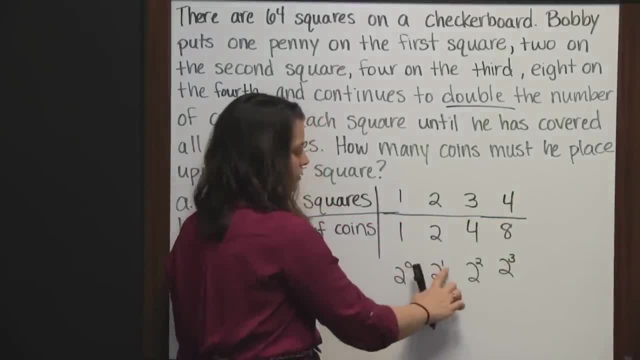 number of squares, our exponent also increases. The first square had 2 to the power of 0 coins. The exponent is 1 less than the square that worked On. the second square- 2 to the first power. The exponent is 1 less than the square we're. 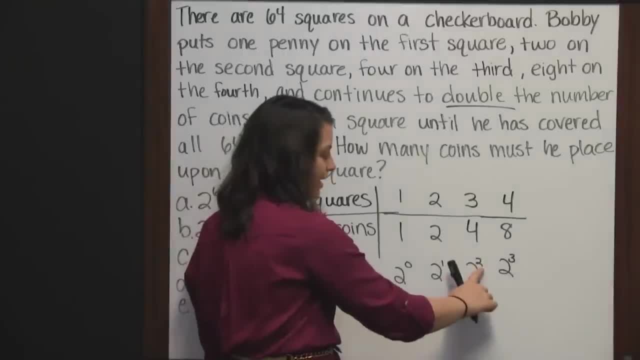 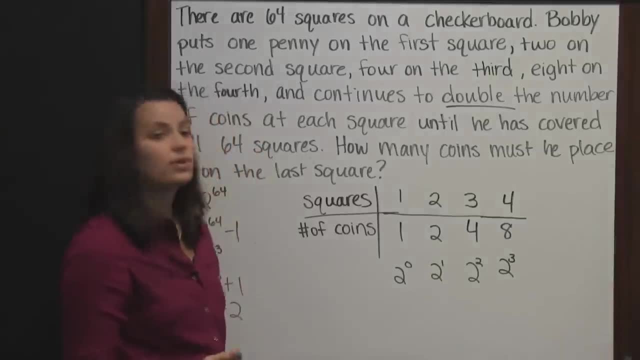 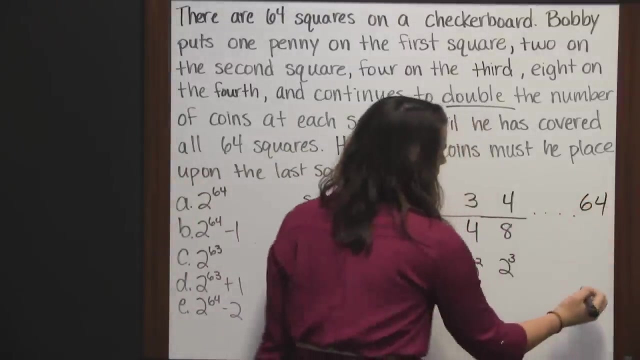 on The third square, 2 to the second power, The exponent is 1 less than the square we're on, and so on and so forth. Then, how many pennies will be on the 64th square? Well, we know that our exponent: we're going to have a base of 2 and our exponent is going 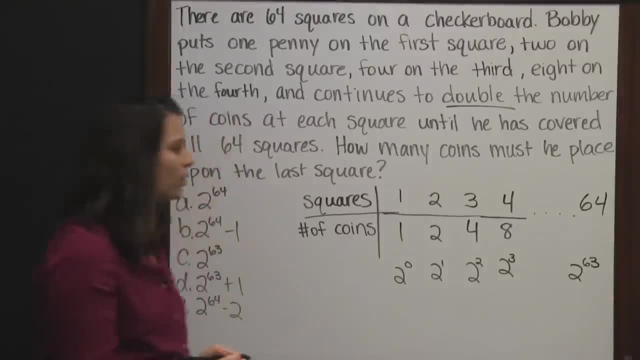 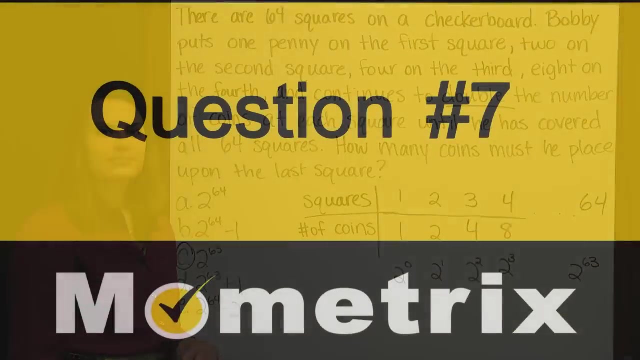 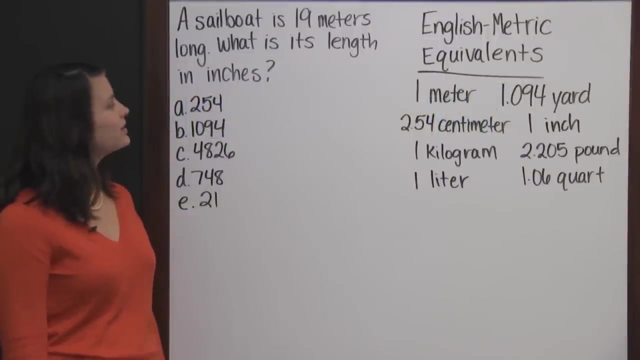 to be 1.. 1 less than the square we're on, so we'd have 2 to the 63rd power number of coins on our 64th square, which is answer C. A sailboat is 19 meters long. What is its length in inches? 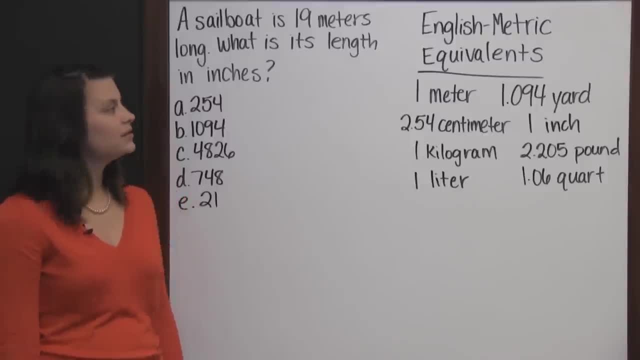 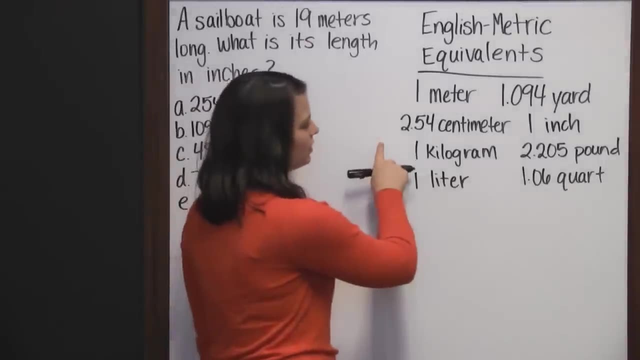 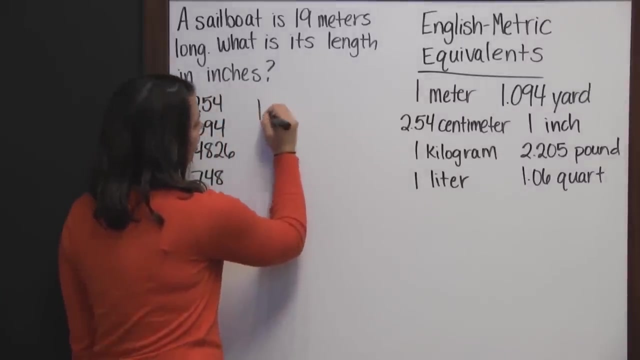 There are many ways to approach this problem and solve it. The first thing I'm going to do is convert my meters into centimeters, because then it's a quick conversion into inches from there. So I know that 1 meter is equal to 100 centimeters and we can use a proportion to solve. 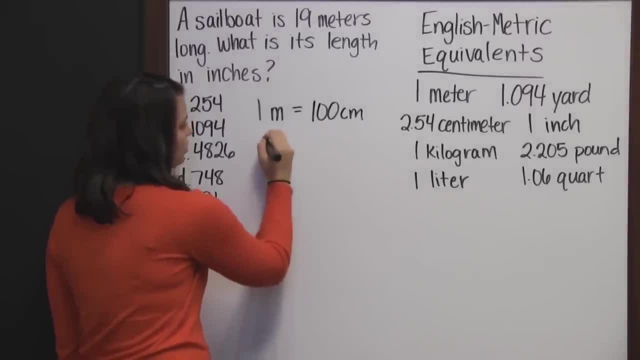 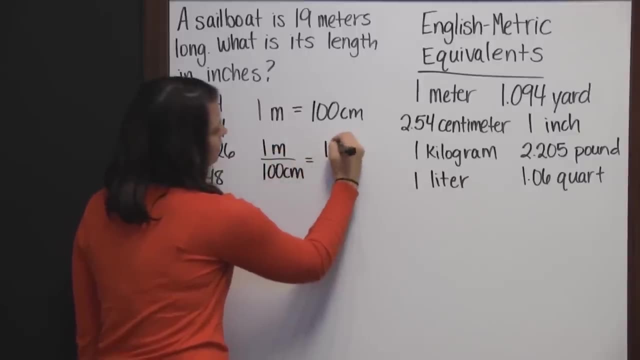 We can take this conversion factor and use it as a ratio. So 1 meter is 100 centimeters, which equals 19 meters. is how many centimeters? And then to solve the proportion we cross, multiply 1 times X is X and 100 times 19 is 1900.. So it's 1900 centimeters. Now I can use another proportion. 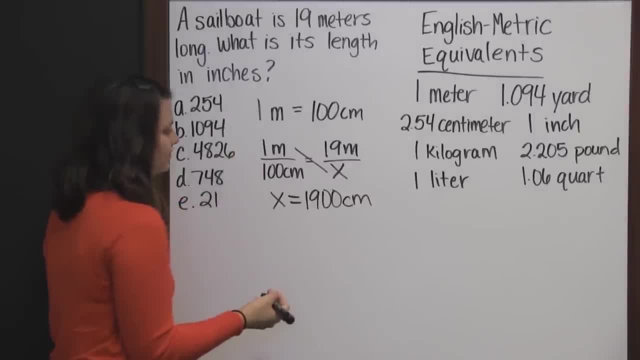 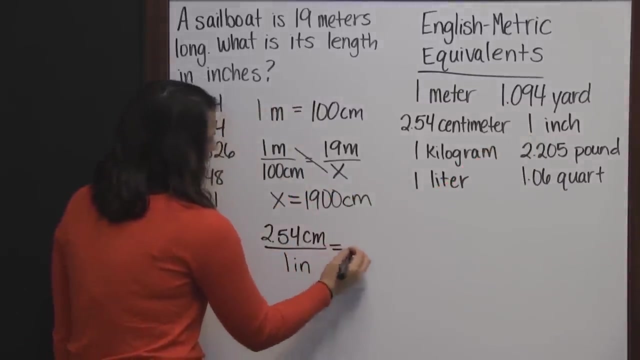 to solve for or to find inches. I know that 2 and 54 hundredths centimeters is 1 inch and I have 1900 centimeters and I need to know how many inches that is. And again to: 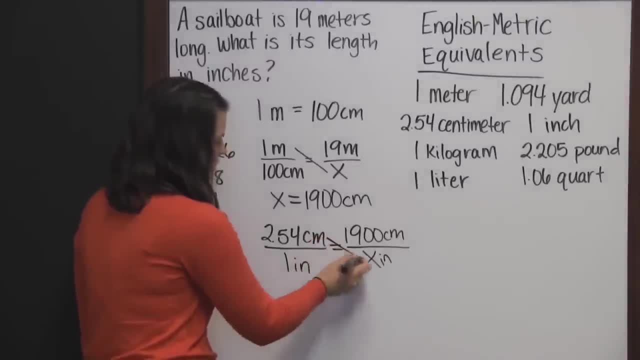 solve a proportion we cross. multiply So 2 and 54 hundredths centimeters times X. 2 and 54 hundredths X is equal to 1 times 1900, which is 1900. And I forgot to put my little line up here, so I'll do that. And now we need to solve. 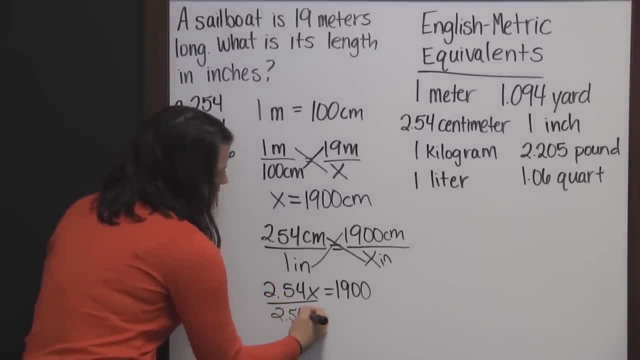 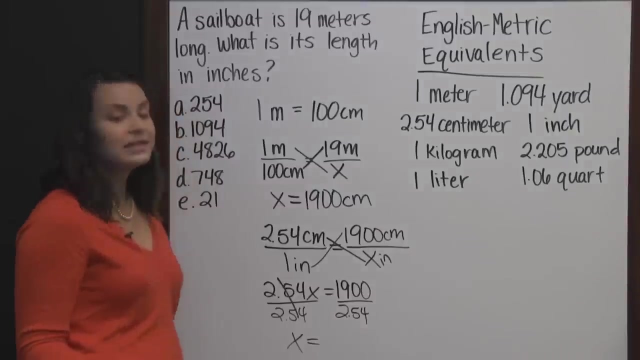 for X, which means dividing both sides by 2 and 54 hundredths. How many centimeters for this? 2 and 54 hundredths, 250?, 250?, 350.. uct: 4 hundredths divided by 2 and 54 hundredths is 1, times X is X, and that equals 1900 divided. 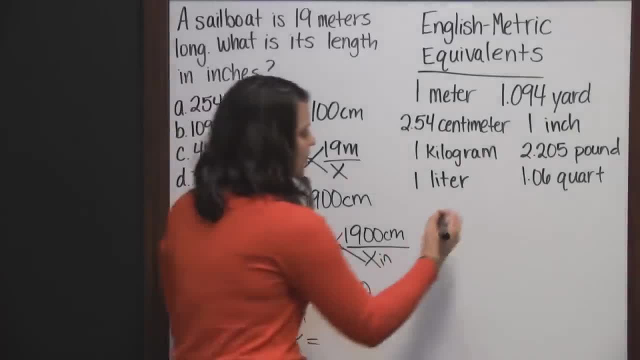 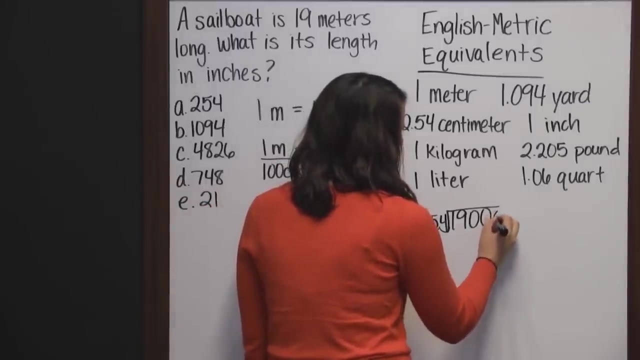 by 2 and 54 hundredths. so we need to do some division, which means I have to move this decimal two places to the right. So I have to take my decimal in 1900 and move it two places to the right, which means adding. 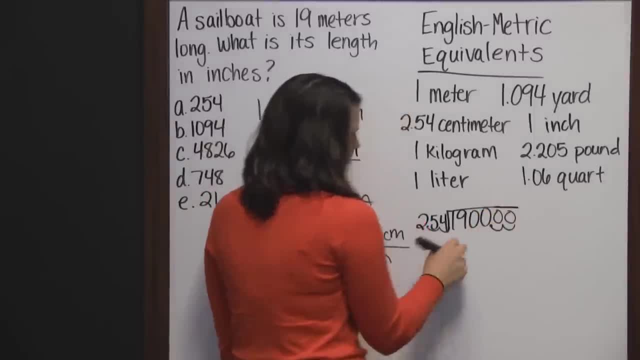 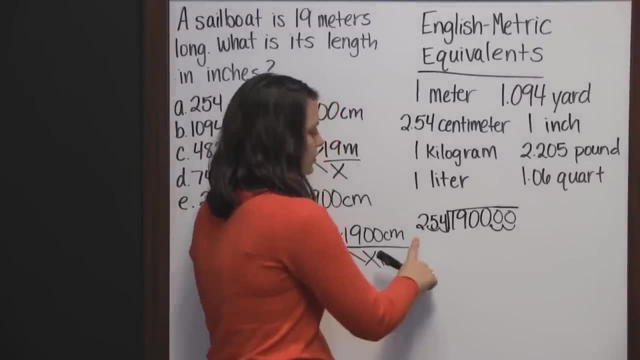 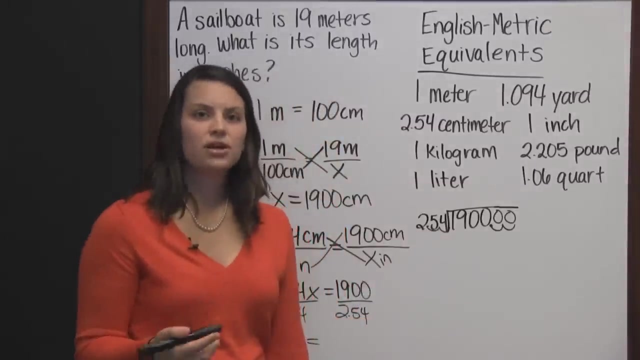 two zeros. So now my number is 190,000 being divided by 254.. So 254 does not go into 1, or into 19, or into 190,, but it does go into 1900.. And we can use compatible numbers here to get a very quick estimate of how many times. it goes into 1900.. So 254 is very close to 250. So 250,, 500, 750,, 1,000, 1,250, 1,500,, 1,750, 1,800.. 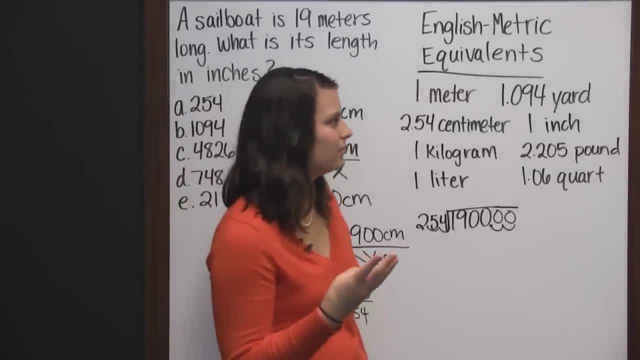 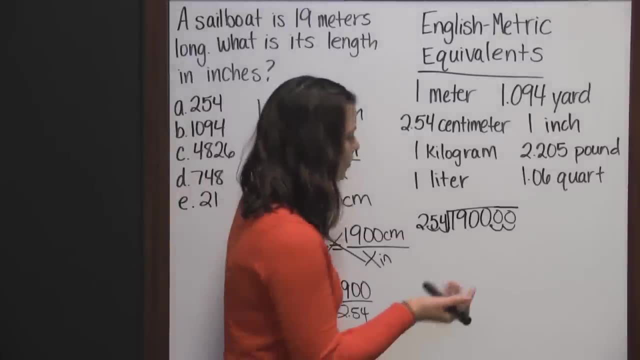 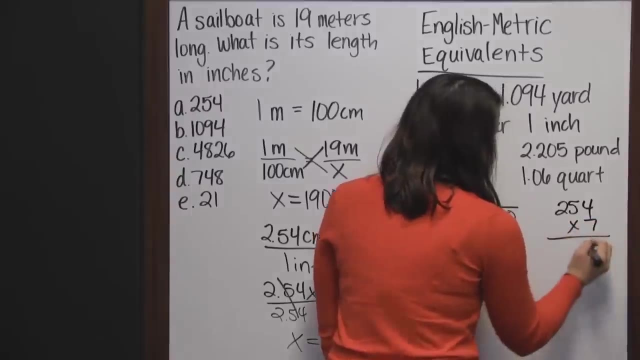 So it would sorry 1,750 and then 2,000. So it only goes 7 times 2,000.. 2,000 is too much, So 254 only goes 7 times into 1900, and we can see what that is right here. 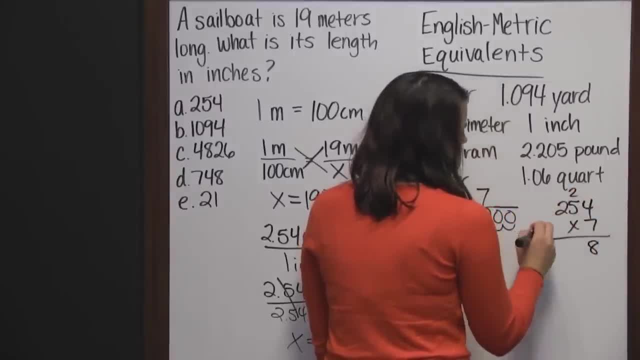 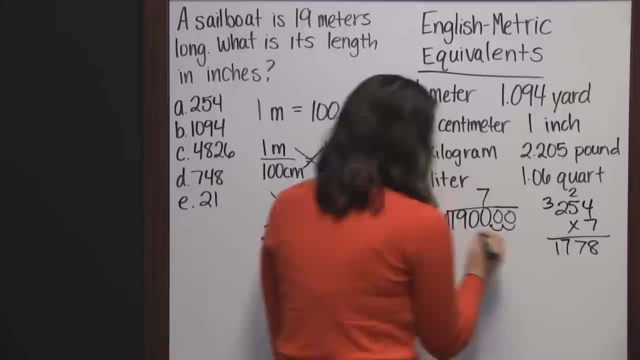 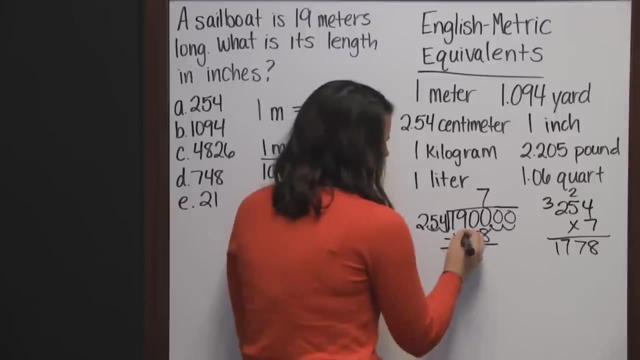 Seven times 4 is 28.. Seven times 5 is 35,, 36,, 37.. Seven times 2 is 14, plus 3 is 17.. So it's 1,778, and then we subtract those. 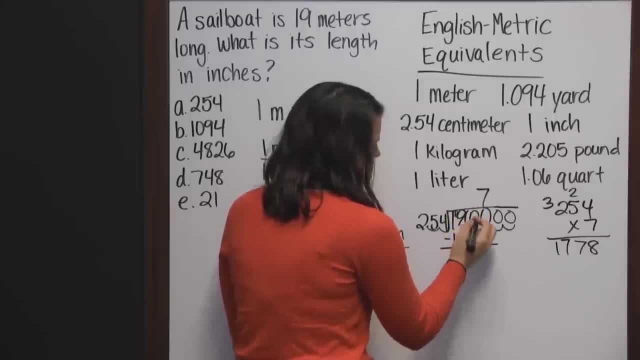 And we have to borrow from the 9. And that becomes an 8.. So this is 10.. And we borrow from the 10., It becomes a 9.. This is 10.. So 10 minus 8 is 2.. 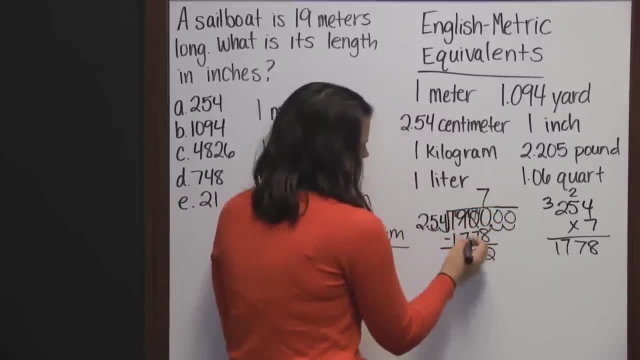 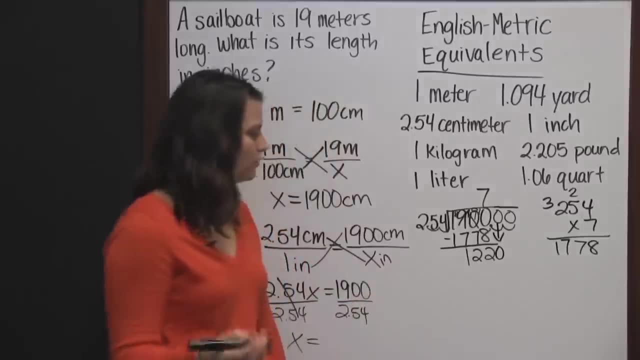 9 minus 7 is 2. And 8 minus 7 is 1. 122.. So now we bring down our next 0.. And again we can use that 250 rule to see how many times it goes into 1,220.. 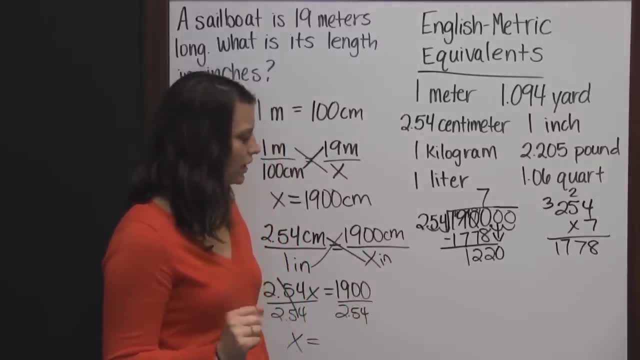 So 255 minus 9 is 1.. 9 minus 7 is 2.. 9 minus 7 is 1. 1,000.. 1,000.. 500,, 750,, 1000, and then it would be 1250,, but 1250 is too much, so it only goes four. 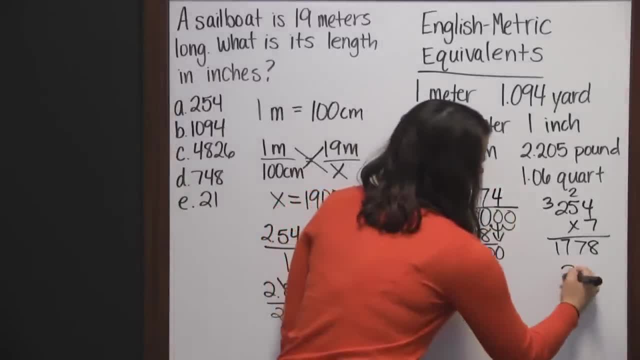 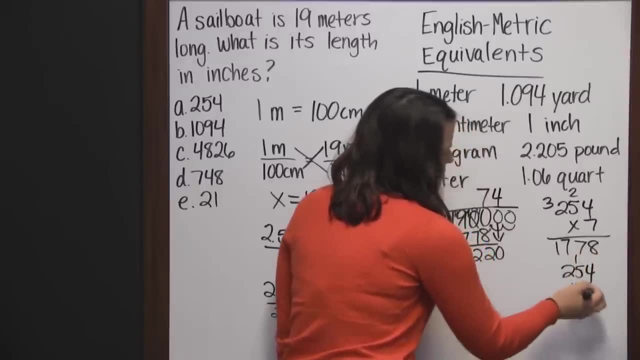 times. So let's see 254 times 4,. 4 times 4 is 16,. carry the 1, 4 times 5 is 20, plus 1 is 21,. 4 times 2 is 8, plus 2 is 10, so that's 1,016, and then we subtract. 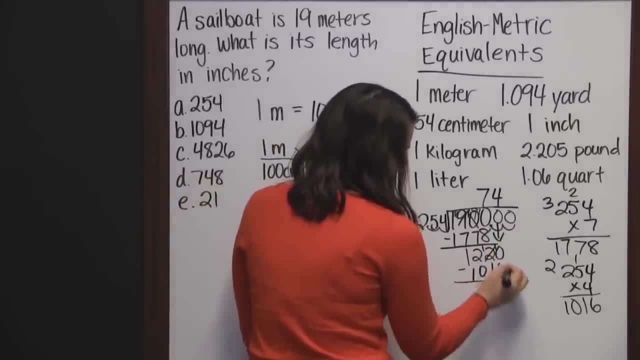 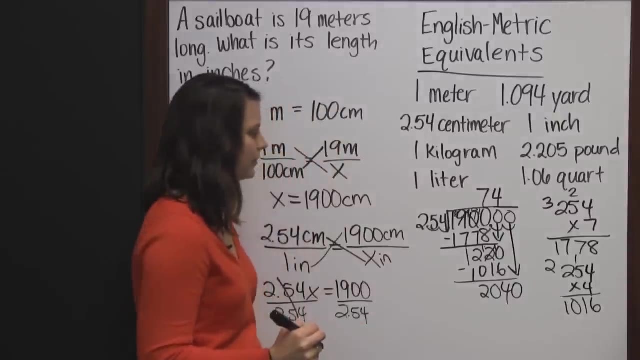 So we need to borrow from this 2, that becomes a 1, so this is 10 minus 6 is 4,, 1 minus 1 is 0, and 2 minus 0 is 2, so that's 204, and then we bring down our 0 here. So again, how many times does 250 go into 2000? 2040, so we have 250, 500, 750, 1000, so 4 more times for 2000,. so it looks like a total. 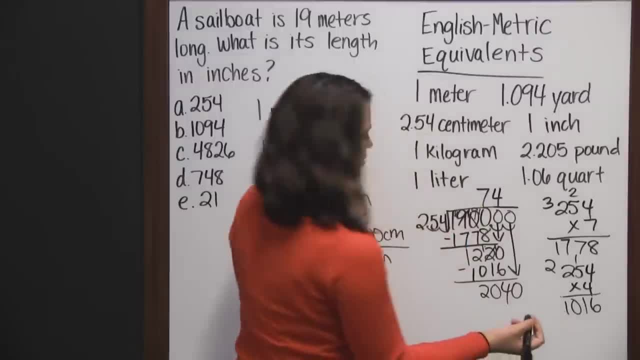 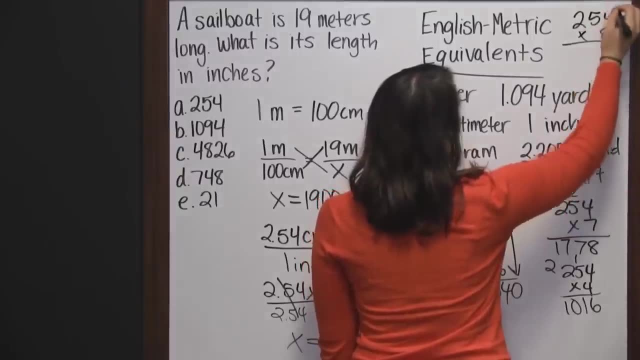 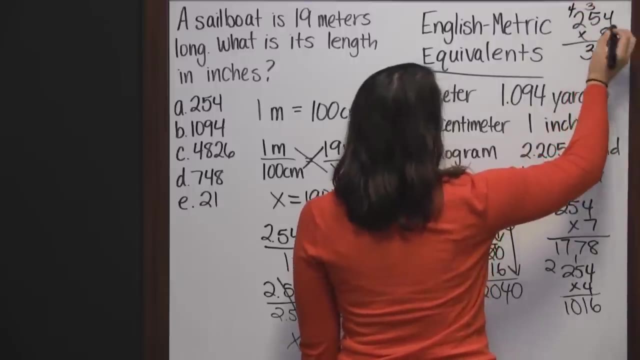 of eight times. So let's see, let's check that, see where I have some room. we'll just do it up here. 254 times 8,, 8 times 4 is 32,, 8 times 5 is 40, plus 3, 43.. 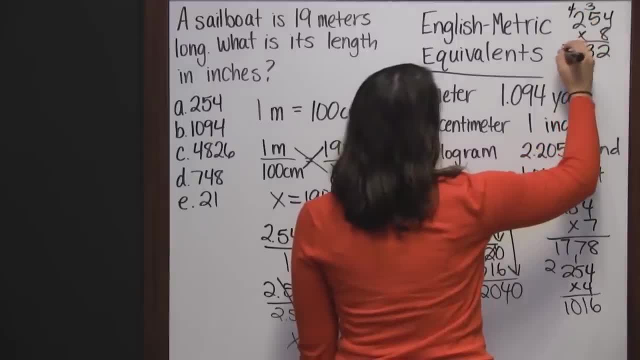 8 times 2 is 16.. 8 times 4 is 18.. 8 times 2 is 18.. 16 plus 4 is 20, so it's 8 times is correct and it's 2,032.. 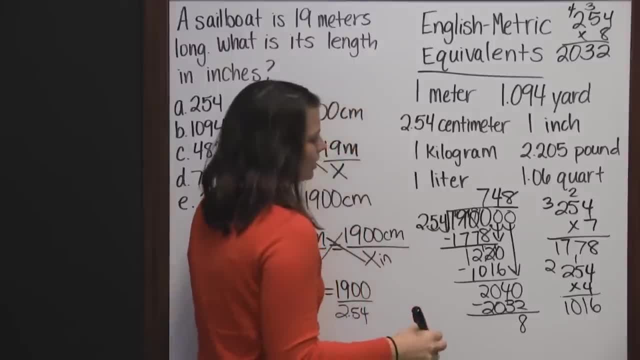 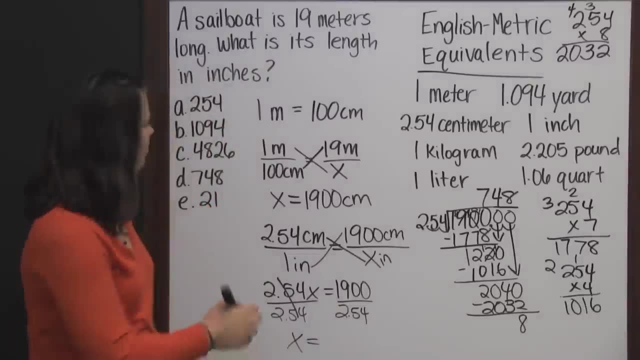 We subtract and we get 8, and that would be our remainder. It would be 8 out of 254, or we could keep going to find our decimal. But if we look at our answers, we don't need to keep going, because none of our answers have the decimal as part of it. 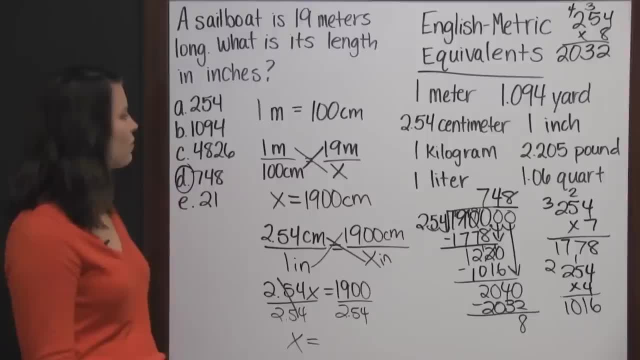 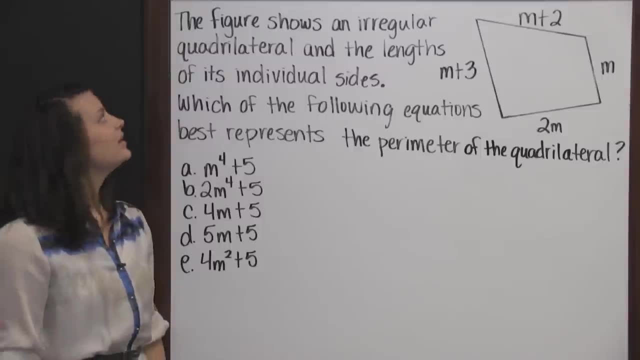 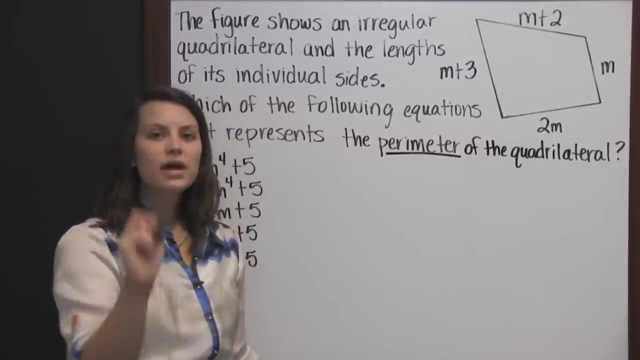 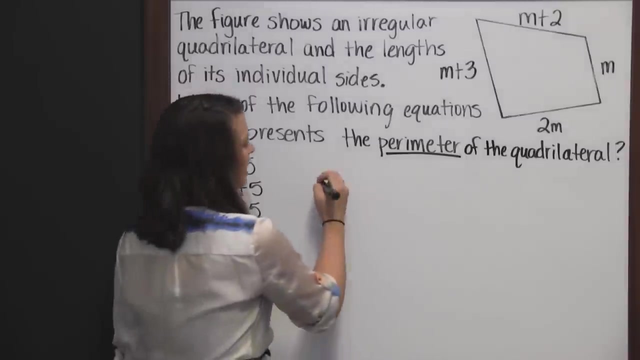 So our answer is D 748 inches. The figure shows an irregular quadrilateral and the length of its individual sides. Which of the following equations best represents the perimeter of the quadrilateral? The perimeter is the distance around a figure. To find the perimeter of any shape, you can simply add all of the sides. 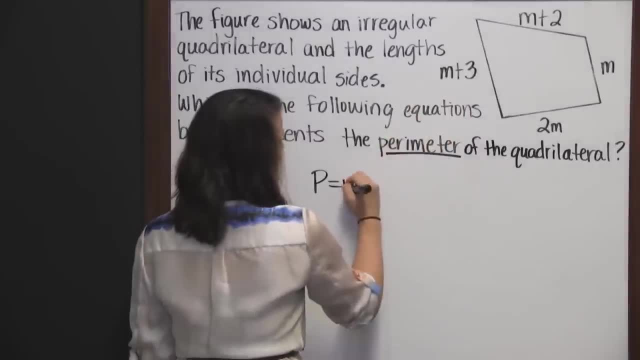 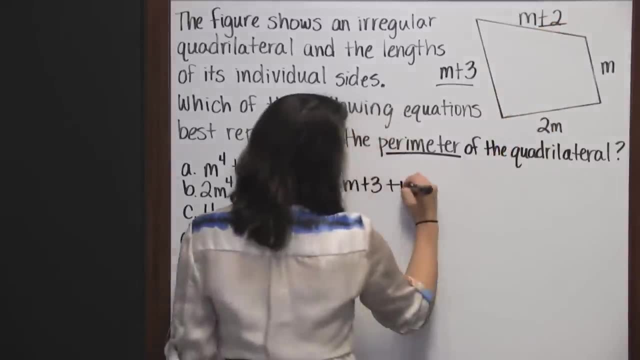 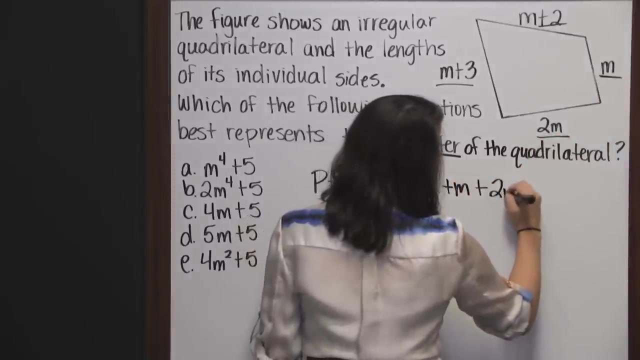 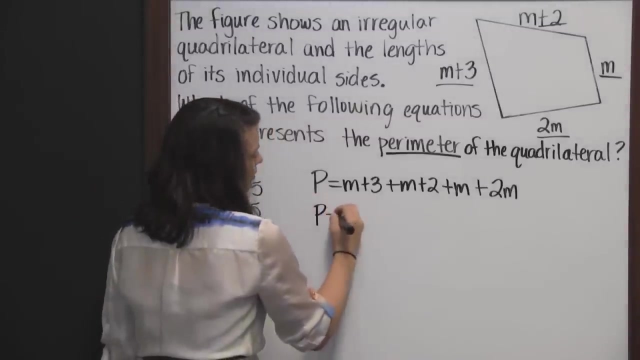 So the perimeter is M plus 3 plus M plus 2 plus M plus 2M. And now we just need to combine like terms. So the perimeter is M plus M plus M plus 2M. so that's 1,, 2, 3 M's plus 2 M's is a total of 5 M's plus 3 plus 2 is 5.. 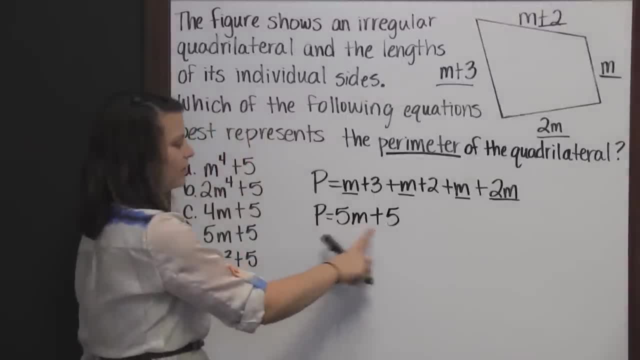 So the perimeter is 5 M's plus 2 M's, is a total of 5 M's plus 3 plus 2 is 5.. So we have a üzer- mögen, that is 5-ils, 5 M's plus 5-ils, and the border is a water- sintep. 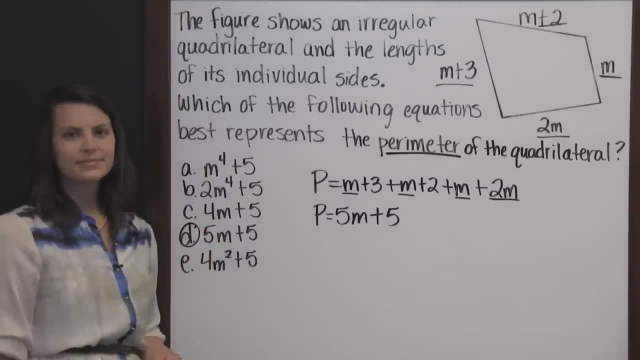 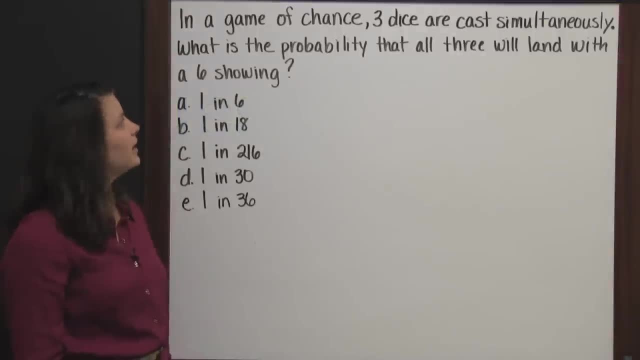 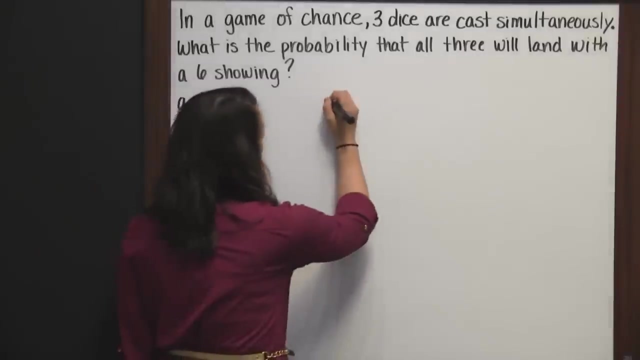 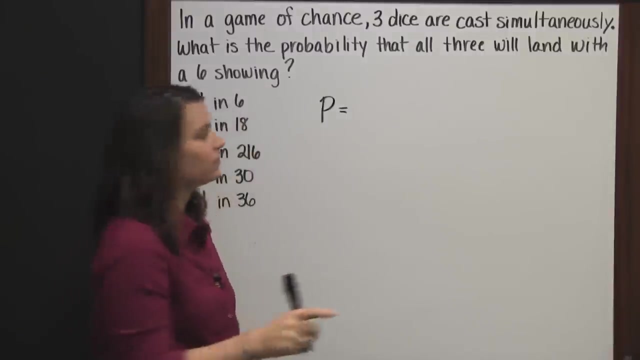 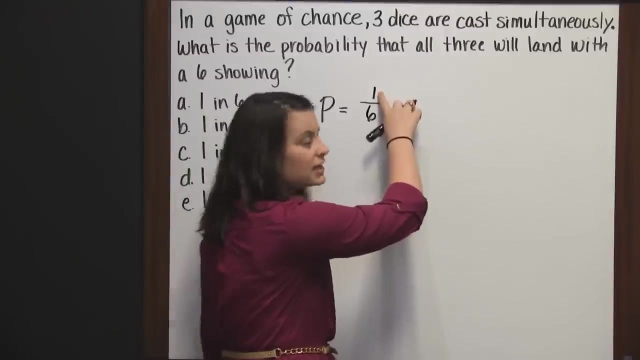 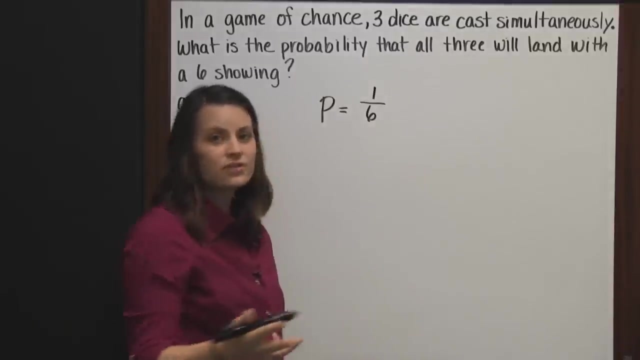 Answer: Damn, that is the answer. one dice landing with a 6 showing is 1 out of 6, since 1 of the numbers is a 6 out of a total of 6 numbers, and the other two dice have the same probability, so times 1, sixth. 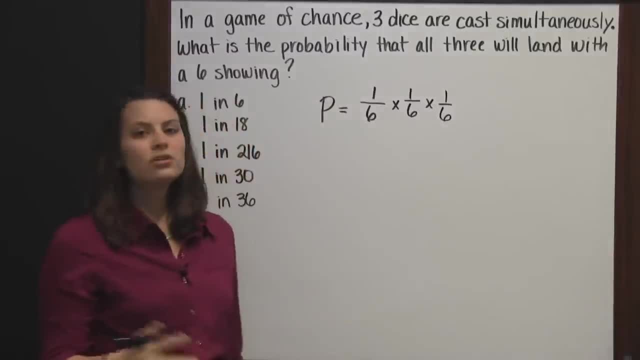 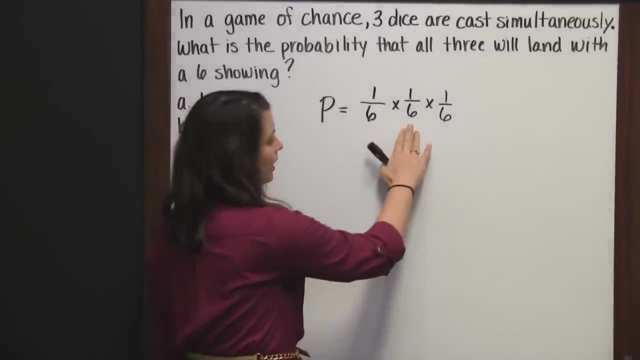 times 1. sixth, All of these events are independent of each other, meaning they don't affect each other, which is why we just multiply the three probabilities of the three dice together. So that means that the probability is 1 out of 6 times 6 is 36, times 6 is 216.. So 1. 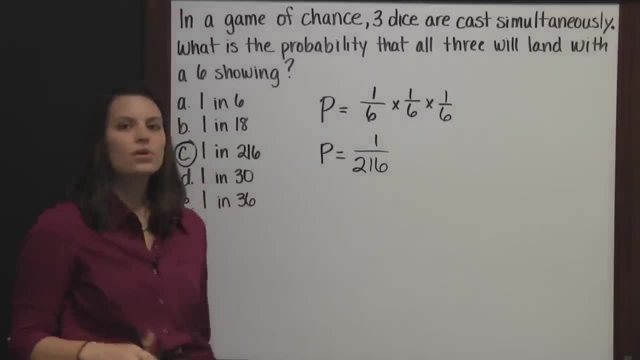 and 216, which, if you really think about it, makes a lot of sense. It's not very likely that when you roll three dice you're going to get three sixes. It's very unlikely. It doesn't happen very often, Maybe one time out of 216 times that you cast those dice. 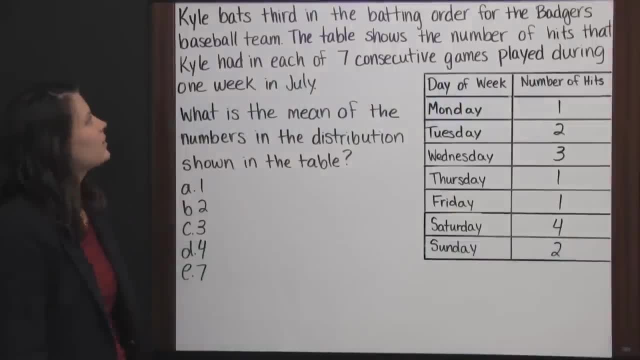 It doesn't really look very likely. Kyle bats third in the batting order for the Badgers baseball team. The table shows the number of hits that Kyle had in each of seven consecutive games played during one week in July. What is the mean of the numbers in the distribution shown in the table? Well, the 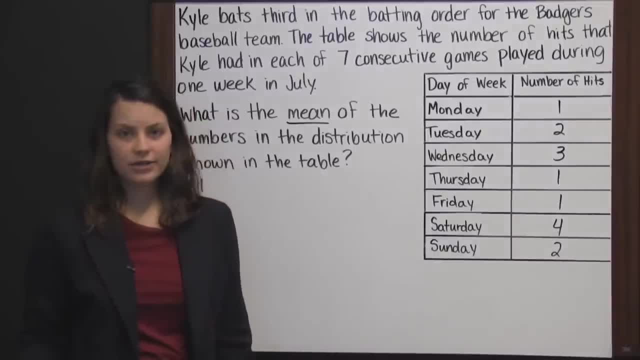 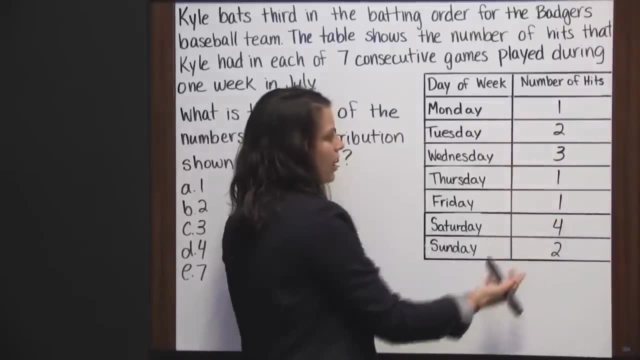 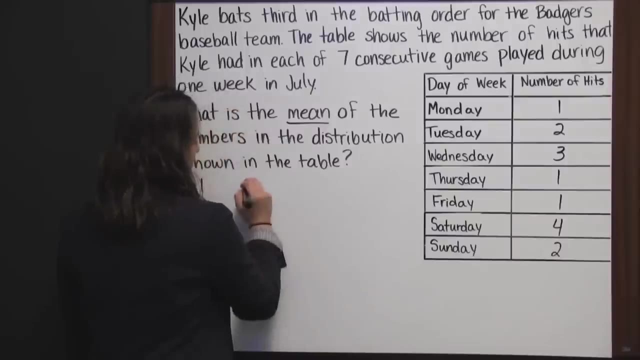 mean of a set of numbers is the average 23. To define the average or the mean, you must add all of the numbers together and then divide them by the number of numbers there are. So first we'll add all the numbers together: 1 plus 2 plus 3 plus 1 plus 1 plus 4 plus. 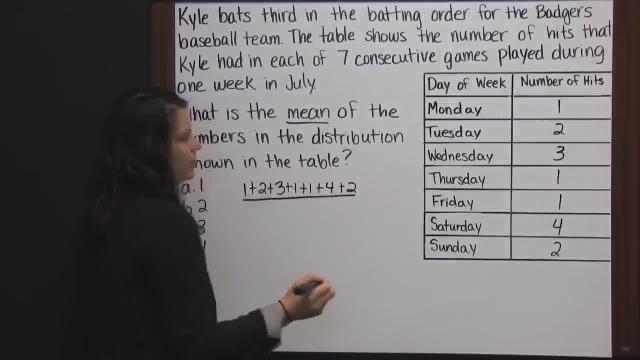 2.. Then we divide by the number of numbers there are, which is 1,, 2,, 3,, 4,, 5,, 6,, 7.. So we divide by 7. And again, this is how we find the mean. Add the numbers together and 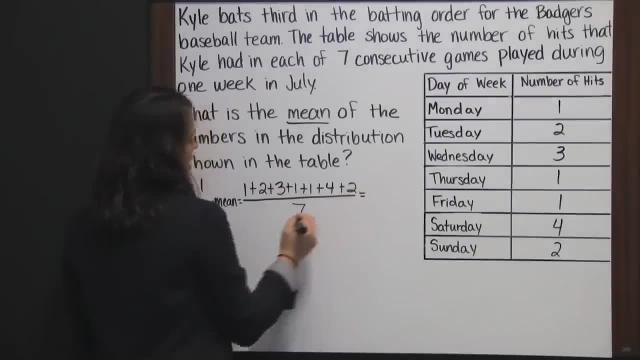 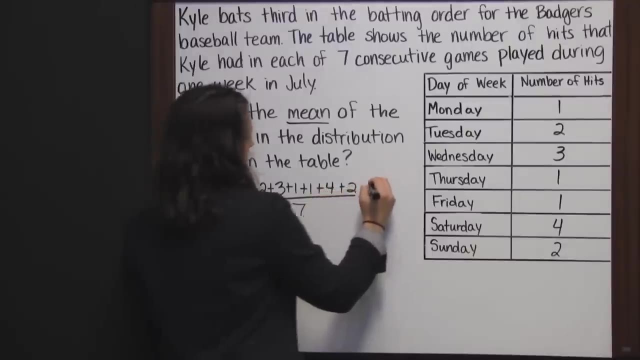 then divide by the number of numbers there are. So that is: 1 plus 2 is 3,, 3 plus 3 is 6, plus 1 is 7, plus 1 is 7.. Plus 1 is 8, plus 4 is 12, plus 2 is 14.. So 14 divided by 7. And 14 divided by 7 is 2.. 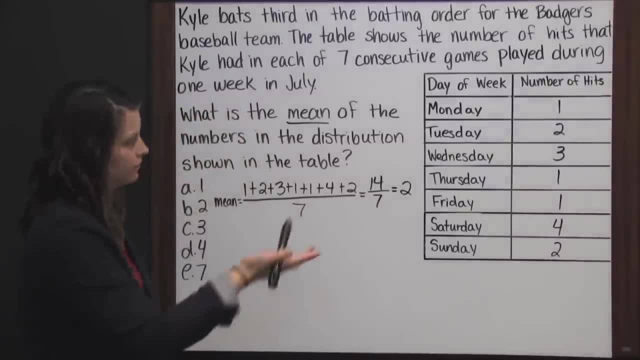 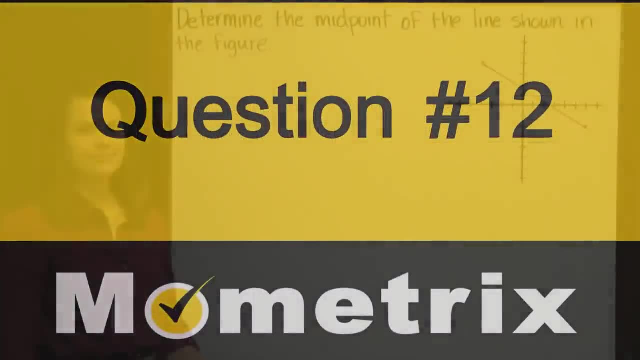 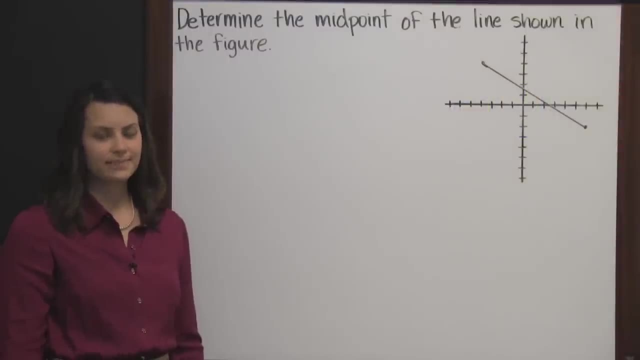 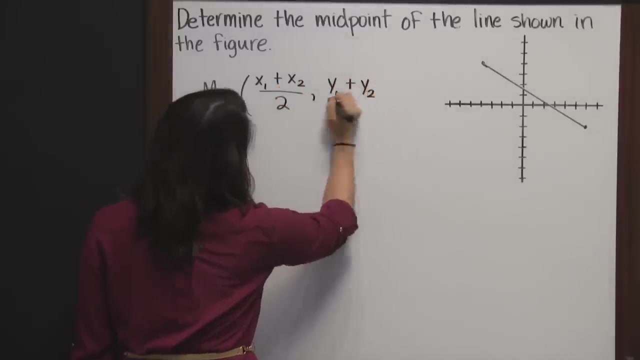 Therefore, the mean or the average of these numbers is 2.. Determine the midpoint of the line shown in the figure. We will use the midpoint formula to find the midpoint of this line. The midpoint formula is x1 plus x2 divided by 2, and then y1 plus y2 divided by 2.. 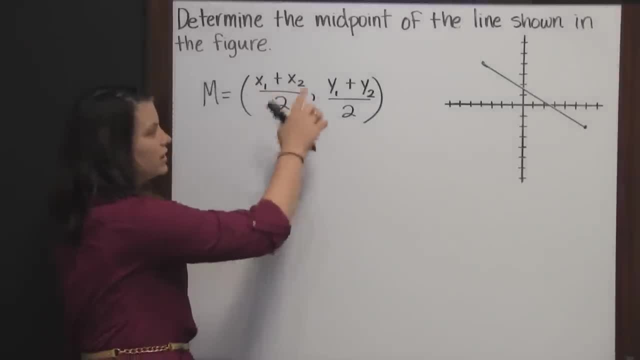 So what you're doing is you're adding your 2x coordinates together from the 2 endpoints and dividing that sum by 2. Basically finding the average of the x values, which would be the middle of the x values, And then doing: 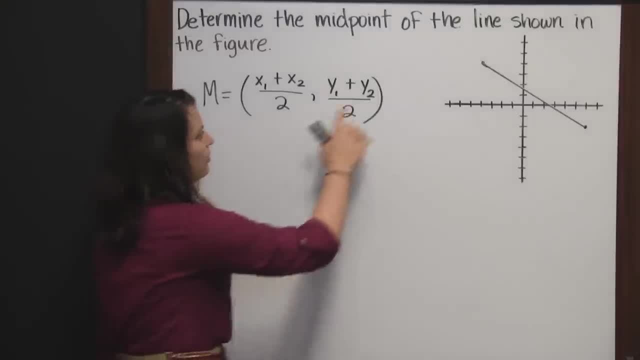 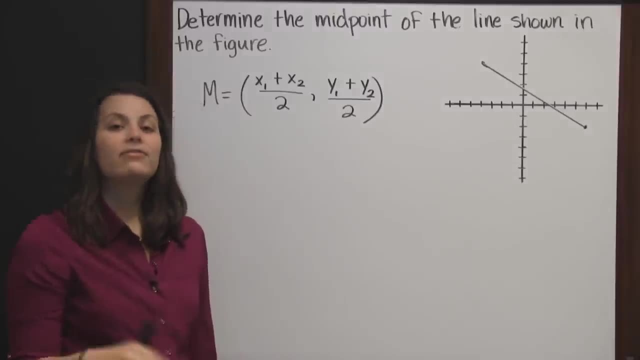 the same with your y coordinates of your 2 endpoints. You'll add those together and then divide that sum by 2. Again finding the average of those y coordinates or the middle of the y coordinates. So when you find the middle x coordinate and the middle y coordinate, you'll then have the coordinates of the midpoint. 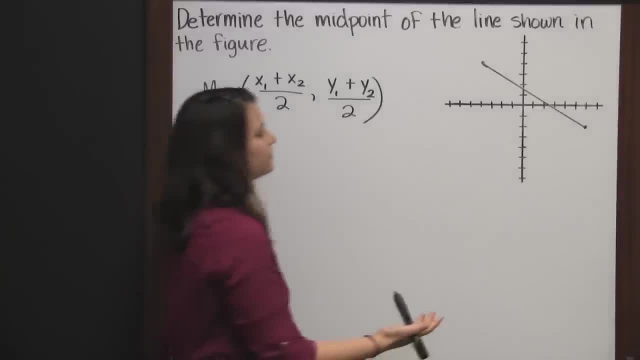 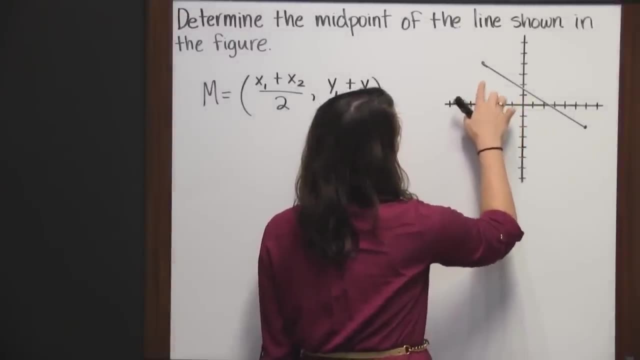 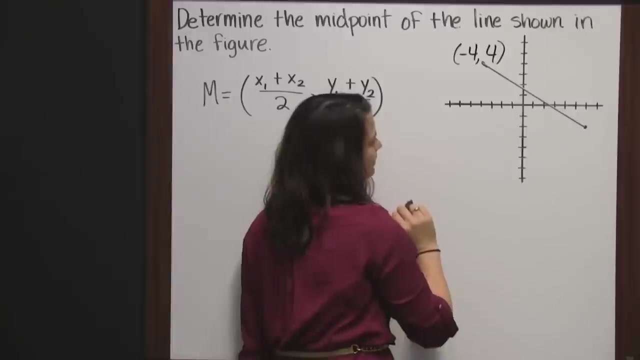 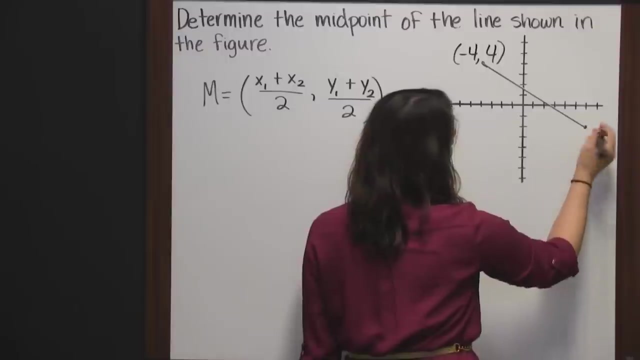 But first we need to know the coordinates of our endpoints. So this end point is at negative 1234, positive 1234,. so these coordinates are negative 4 for this endpoint And this end point is at 123456, negative 2.. 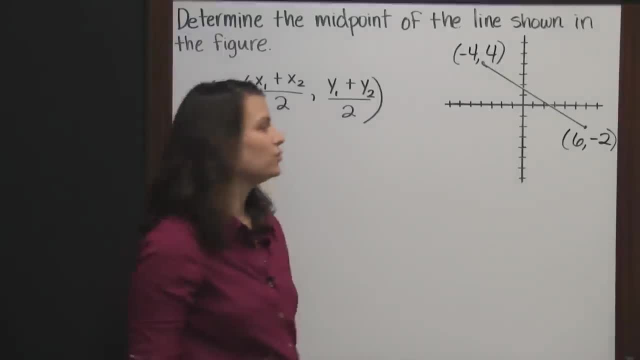 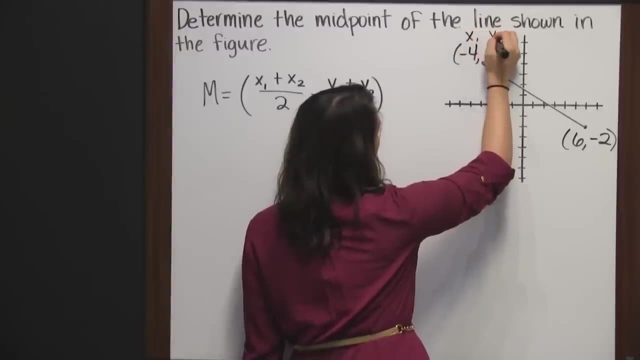 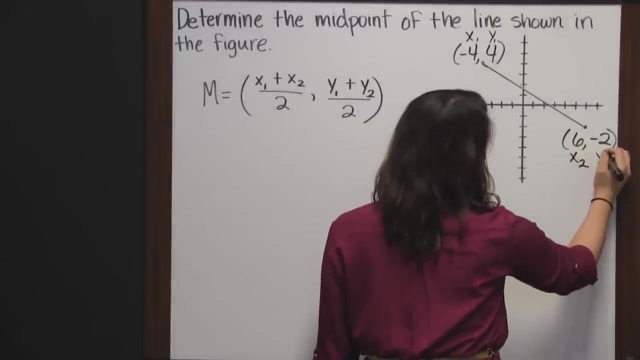 These are my x1, y1, x2, y2 coordinates, and it doesn't matter which one you label as your x1, y1, as long as you label them consistently. For instance, this could not be my x2, y1.. 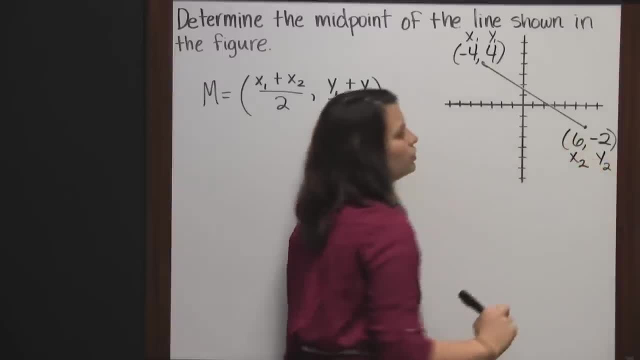 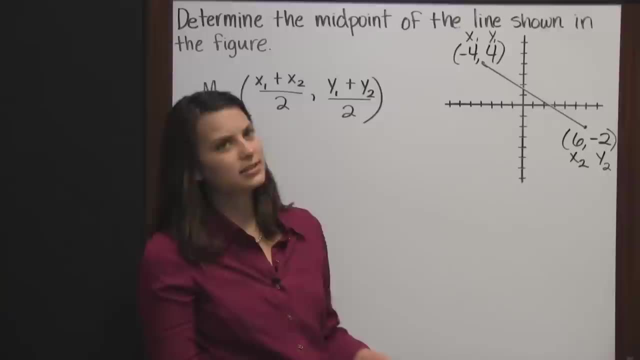 Since this is my x2 coordinate, that means this is my y2 coordinate, Those subscripts, the 1's and the 2's. all that means is: this is the first point, this is the second point, But it really doesn't matter which point is your first and which point is your second. 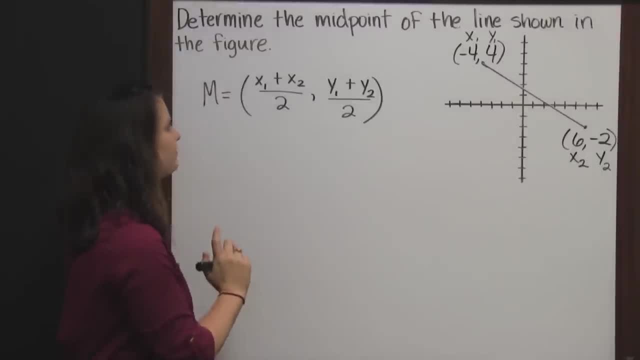 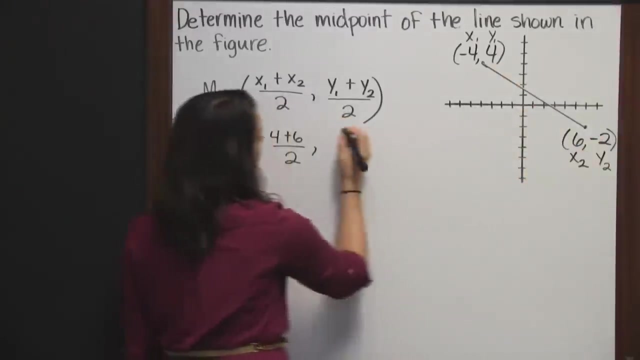 So I just usually label them from left to right, And now all we need to do is substitute and solve. So the midpoint is x1 plus x2, so negative 4 plus 6, divided by 2.. And then y1 plus y2,, 4 plus negative 2, divided by 2.. 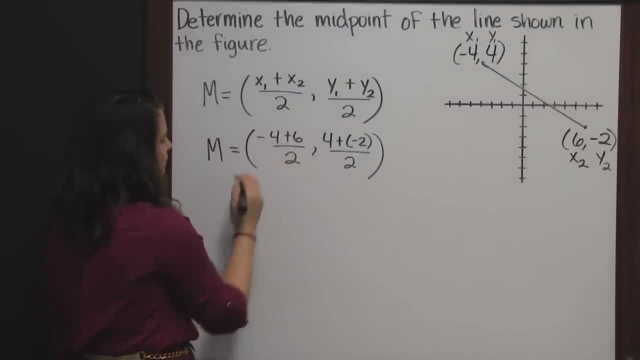 Now we need to simplify by adding negative: 4 plus 6 is 2, divided by 2.. 4 plus negative 2 is 2, divided by 2.. And finally, we divide: 2 divided by 2 is 1,, 2 divided by 2 is 1.. 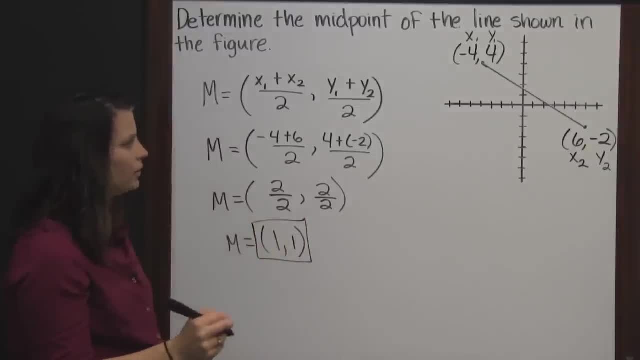 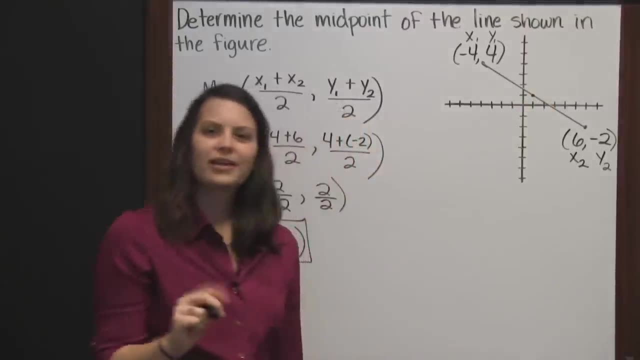 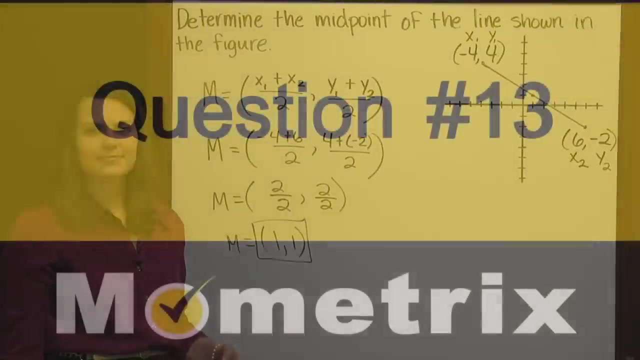 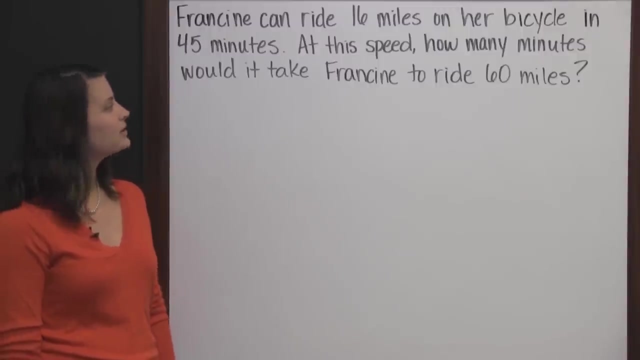 So the midpoint is 1, 1, which you can see on this graph over 1, up 1.. And you know that point does look like it's right in the middle of that line. So that's our midpoint. Francine can ride 16 miles on her bicycle in 45 minutes. 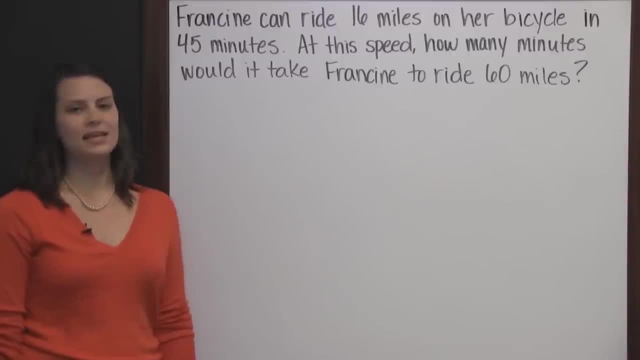 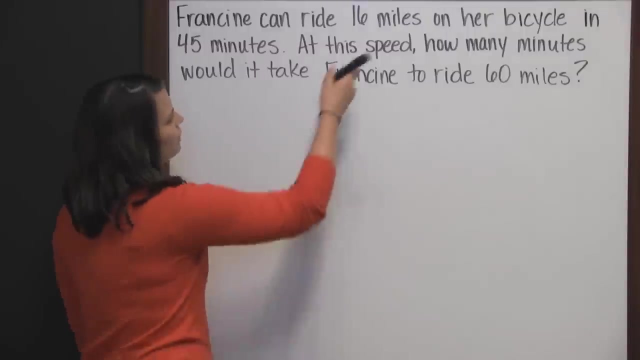 At this speed, how many minutes would it take Francine to ride 60 miles? This problem is a good one. Francine is a good candidate for using a proportion to solve. There's more than one way to solve it, but I like proportion, so I'm going to use a proportion. 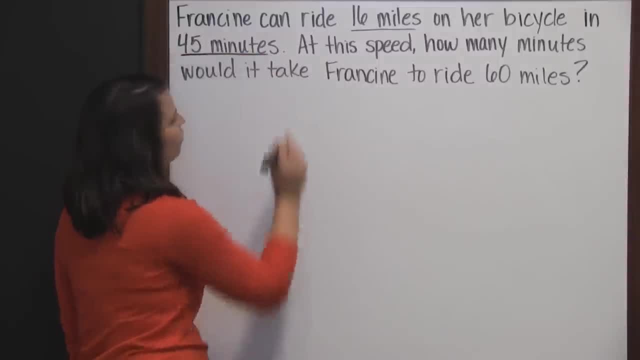 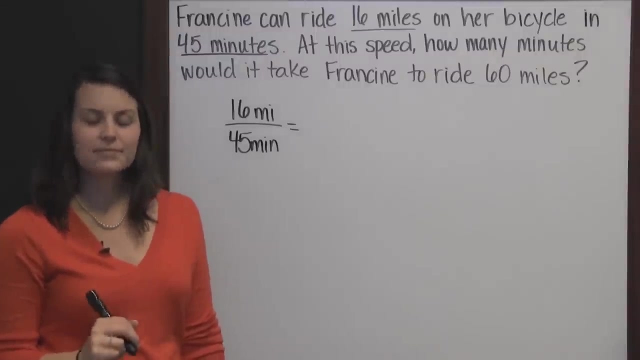 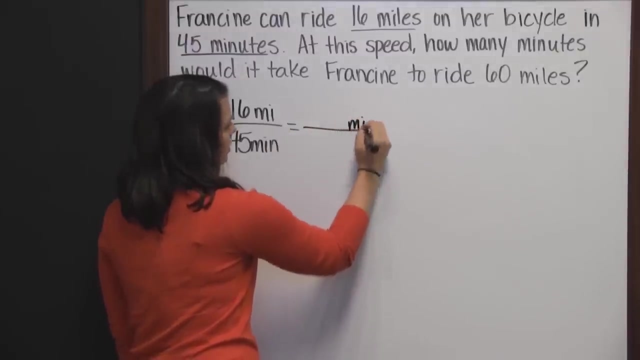 First, I know that Francine can go 16 miles in 45 minutes. That's going to be my first ratio, So I have 16 miles in 45 minutes And the key to setting up a successful proportion is to be consistent. So since our first ratio we have miles to minutes, then our second ratio will also. 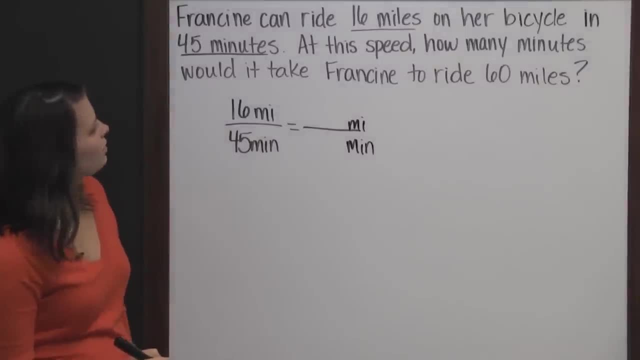 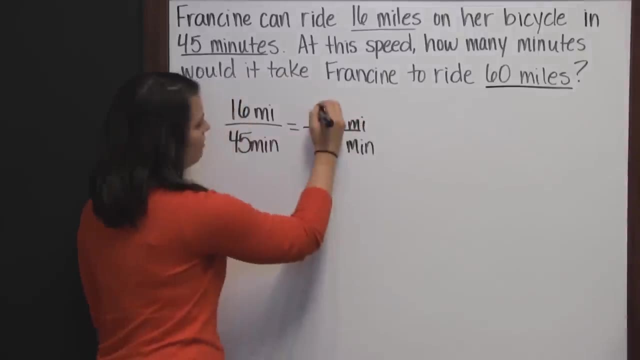 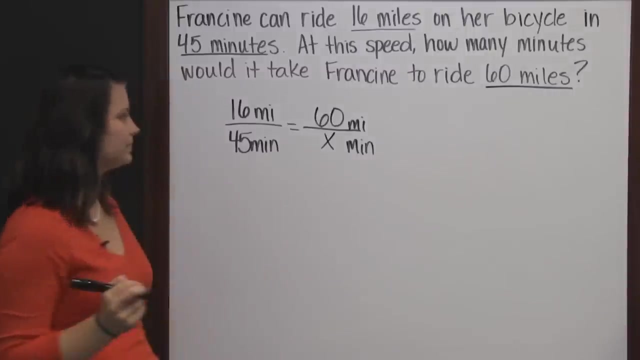 be miles to minutes. So they want to know how many minutes it would take Francine to ride 60 miles. So my miles is 60, and my minutes is what I'm trying to find. so that's where I'll put a variable. 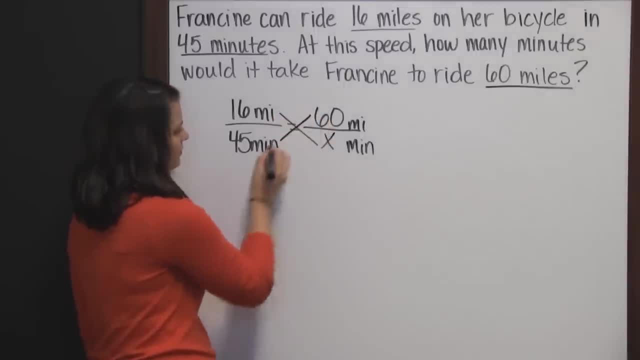 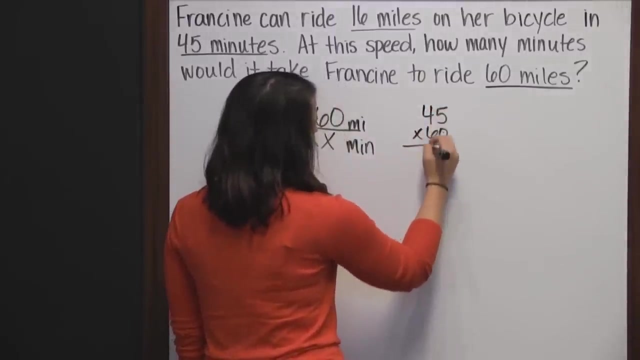 To solve a proportion we cross: multiply 16 times X is 16X, and that equals 60 times 45, 0.. 6 times 5 is 30,. carry the 3.. 6 times 4 is 24, plus 3 is 27,, so 2,700. 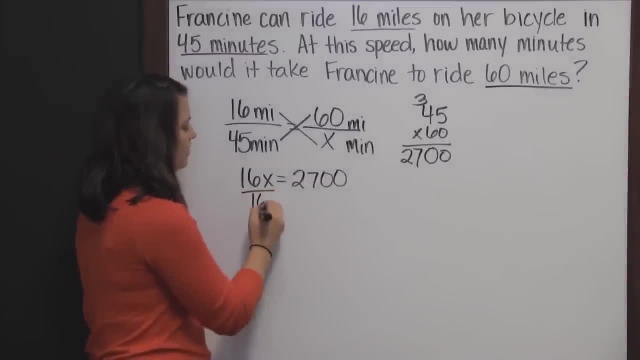 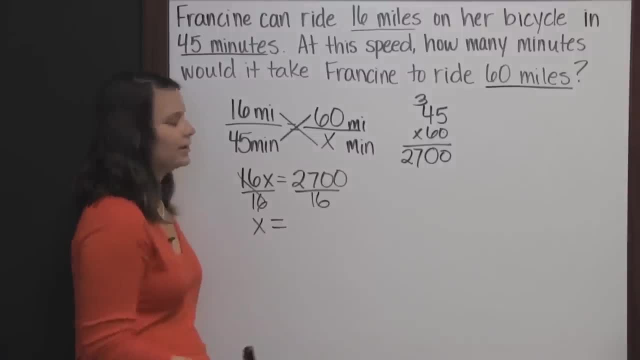 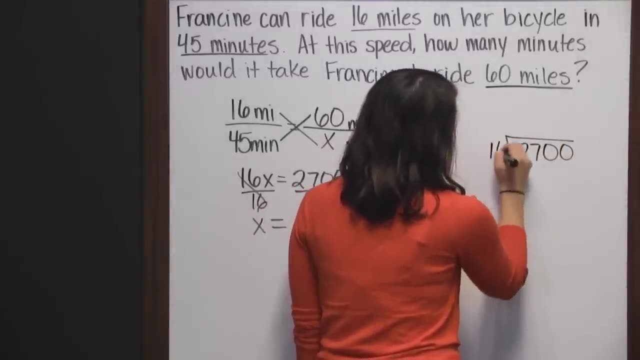 By solving for X by dividing both sides, By solving for X by dividing both sides. So X equals. and now I need to find out what 2,700 divided by 16 is. 16 goes into 2,700 one time. 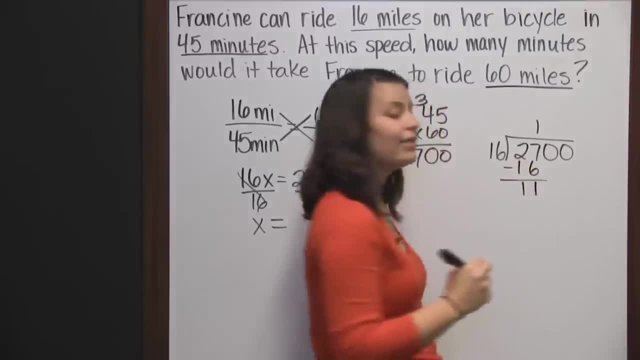 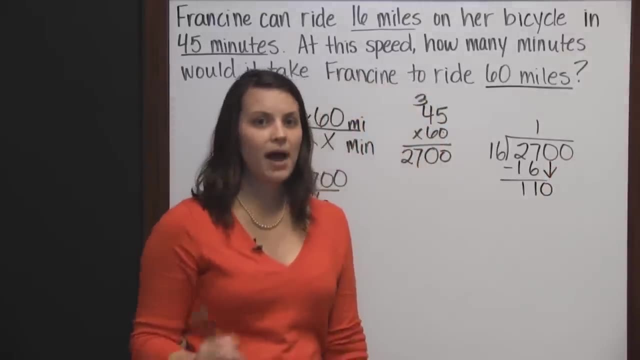 And that's 16, and we subtract and get 11. Then we bring down our 0.. We could use 15 as a compatible number to see if we can get the answer. To see how many times 15 would go into 110. 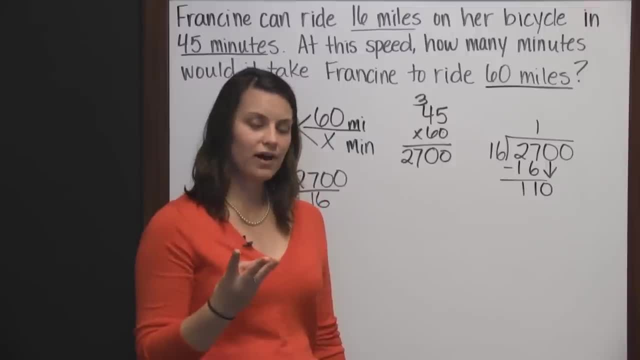 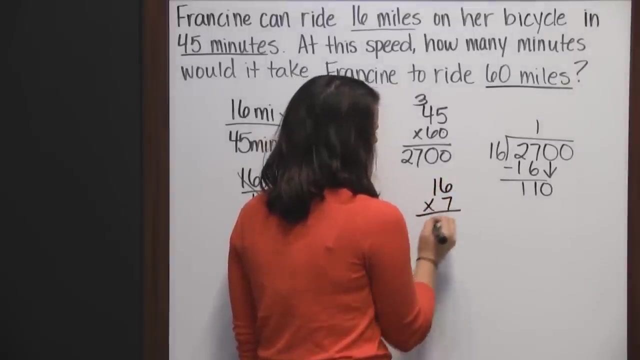 So we have 15,, 30,, 45,, 60,, 75,, 90,, 105.. So 7 times. So let's see if 16 will go into 110. seven times Seven times 6 is 42.. 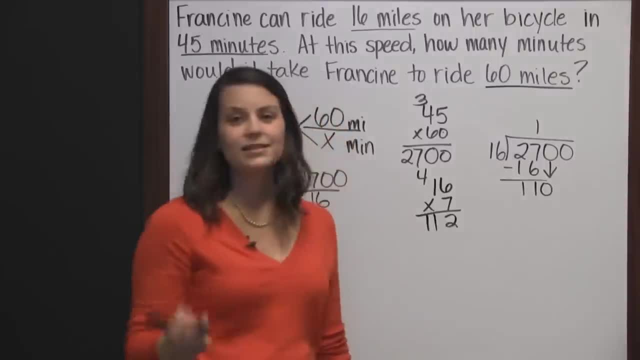 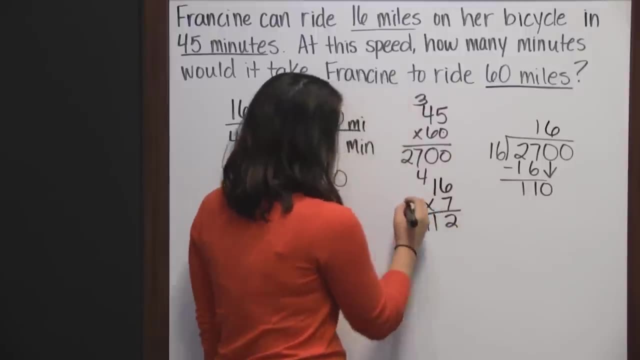 Seven times 1 is 7, plus 4 is 11.. Seven times 6 is 42.. Seven times 1 is 7, plus 4 is 11.. And that's a little too big, Which means I know 16 goes into 110 six times. 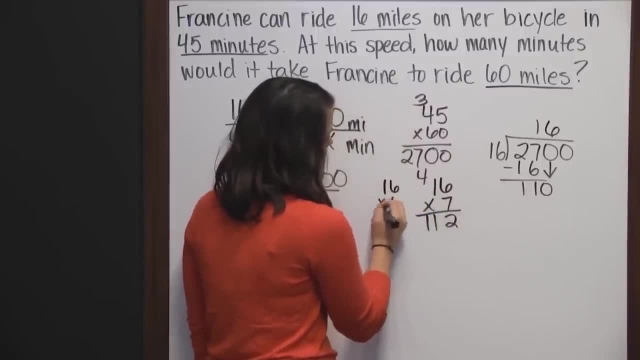 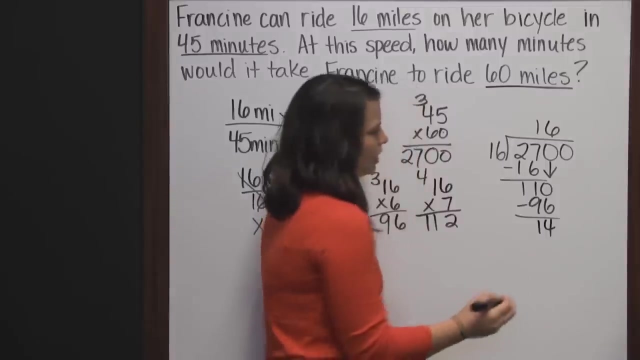 So 16 times 6.. Six times 6 is 36.. Six times 1 is 6, plus 3 is 9.. And that works. So we need to subtract and we get 14.. Then we bring down our next 0.. 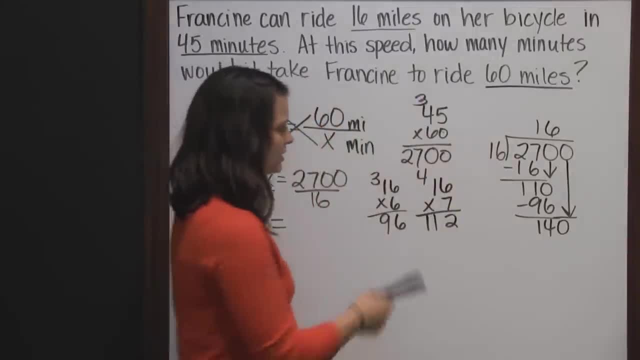 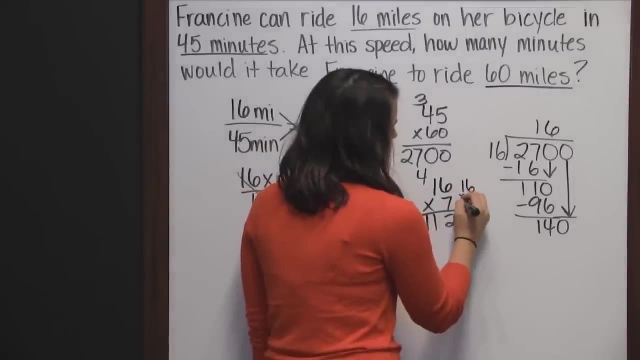 We have 140.. So I know 16 is going to go into 140 at least seven times, but it should go even more than that. So let's see what 16 times 8 is. Eight times 6 is 48.. 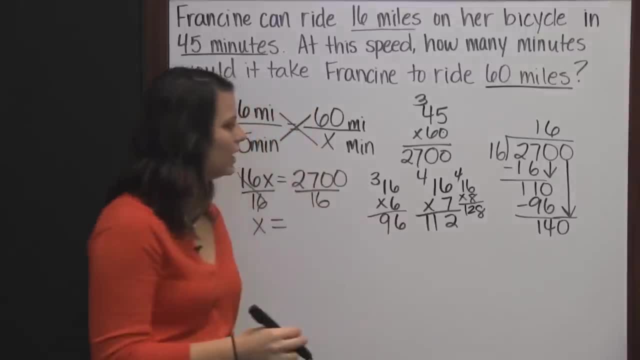 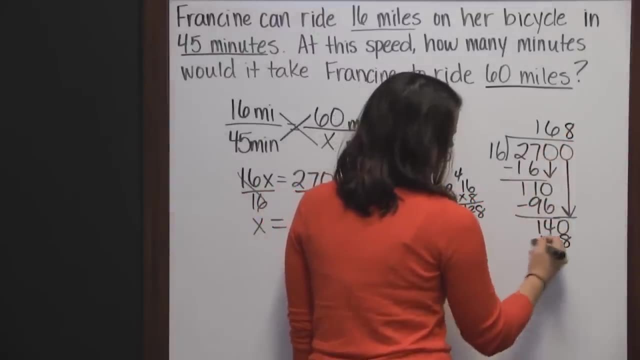 Eight times 1 is 8, plus 4 is 12. And that's all we're going to be able to do. So eight times and we get 128.. And when we subtract those numbers, we get 14.. Okay. 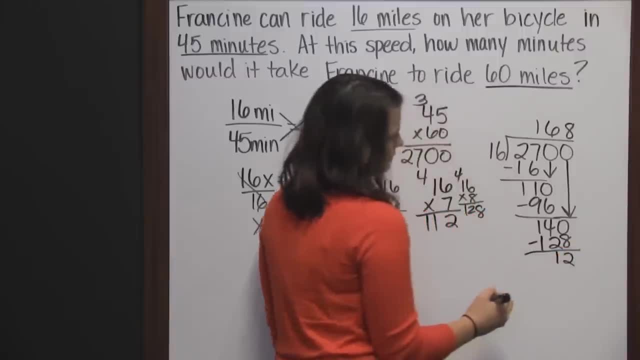 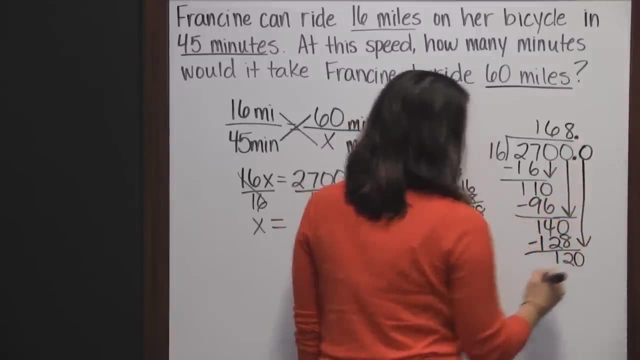 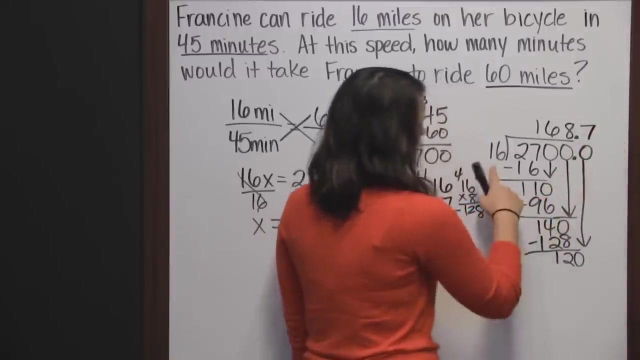 So we subtract those numbers, we get 12.. So that means we need to add a decimal and a 0, and bring it down. Sixteen goes into 120. seven times Sixteen times 7, we found earlier is 112.. 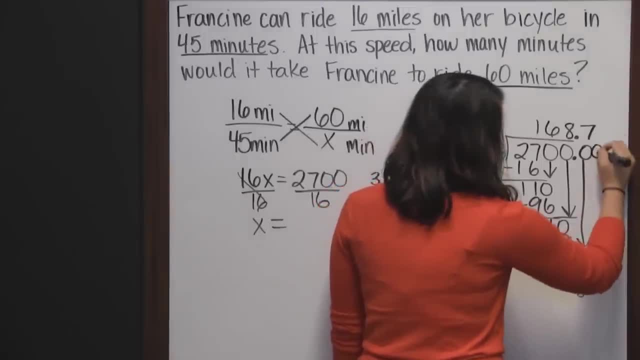 So we subtract and we get 8.. We add another 0, and bring it down. And we subtract those numbers, we get 12.. So that means we need to add a decimal and a 0, and bring it down. 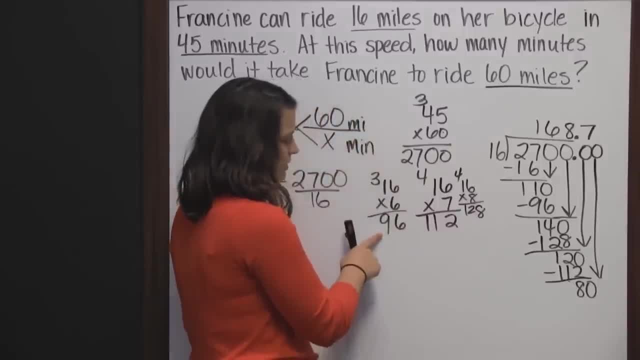 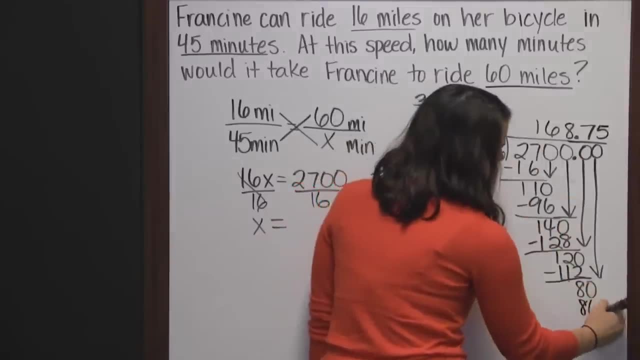 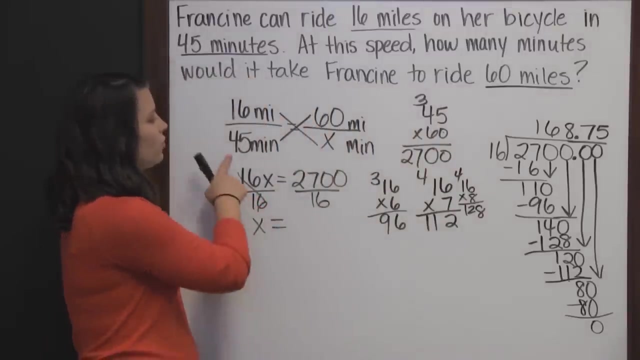 And 16 goes into 80, less than six times and actually exactly five times. Sixteen times 5 is 80. So we subtract and we get a remainder of 0. So that means if it took her 45 minutes to go 16 miles, it should take her 168 and 75. 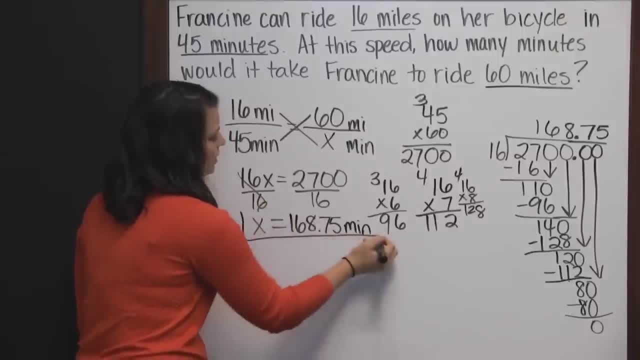 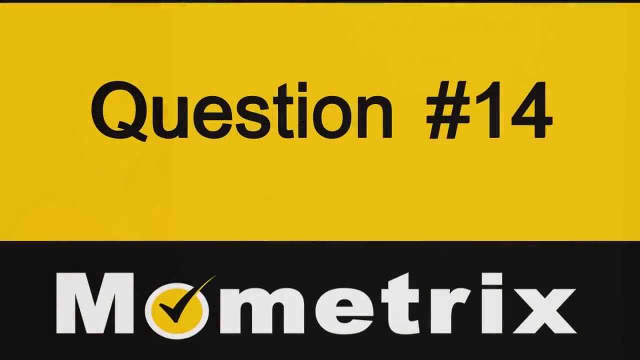 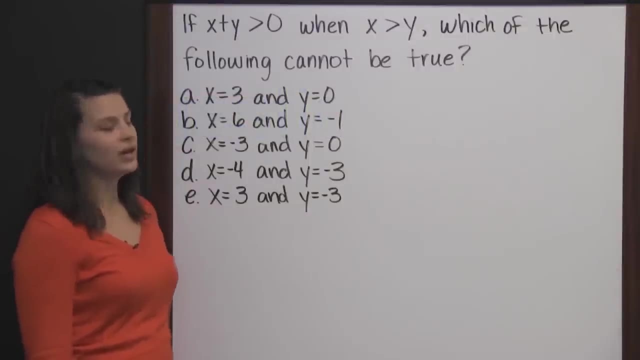 hundredths minutes to go, 60 miles, And this is the answer. This is the answer you would grid in: If x plus y is greater than 0, when x is greater than y, which of the following cannot be true? This word when is very important because it means we're only looking at the situations. 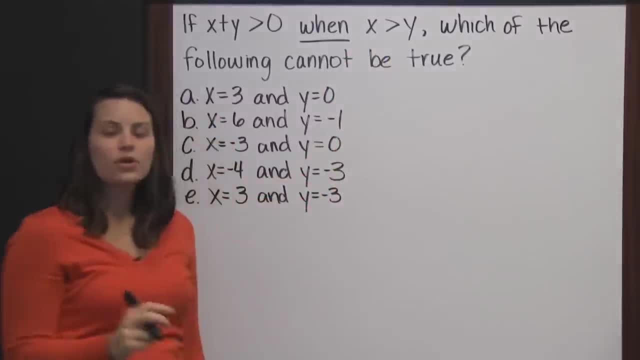 when x is greater than y. So, for example, if x is greater than y, when x is greater than y, which of the following cannot be true? So first we should go through our answers and eliminate the ones that don't satisfy. 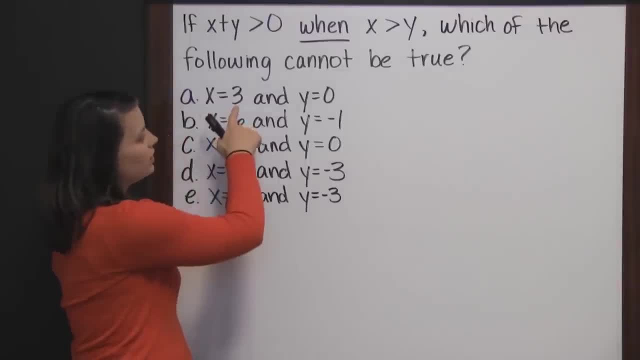 this inequality: Is 3 greater than 0?? Yes, so it stays. 6 is greater than negative 1,, so it stays Negative. 3 is not greater than 0, which means c must be eliminated as a triangle. So we subtract and we get a remainder of 0. 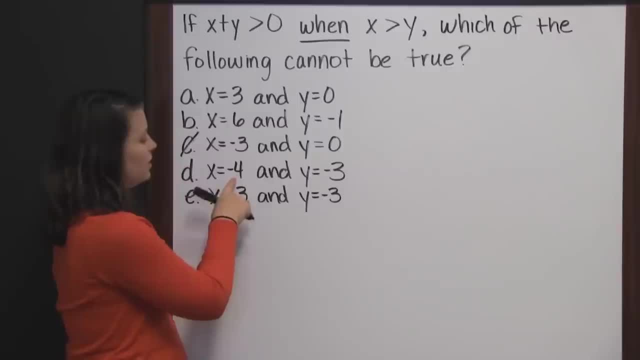 So that means if x is greater than y, which of the following cannot be true? Negative 4 is greater than 0, which means c must be eliminated as a triangle. So we subtract and we get a remainder of 0, which means c is greater than 0. 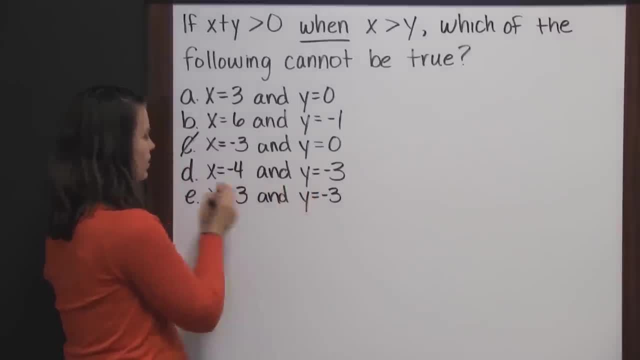 Negative 4 is not greater than negative 3, so it must also be eliminated as a choice. Negative 4 is not greater than negative 3.. 3 is greater than negative 3.. So the three answers left are the only ones that satisfy this inequality. 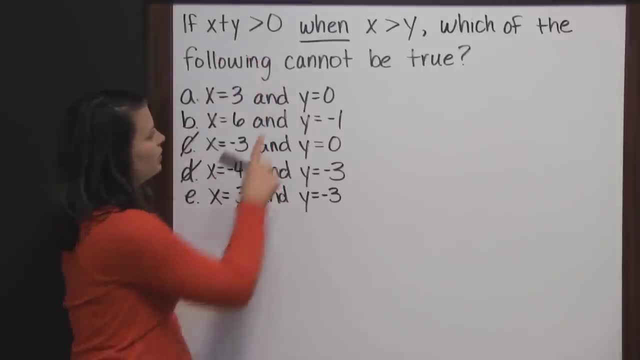 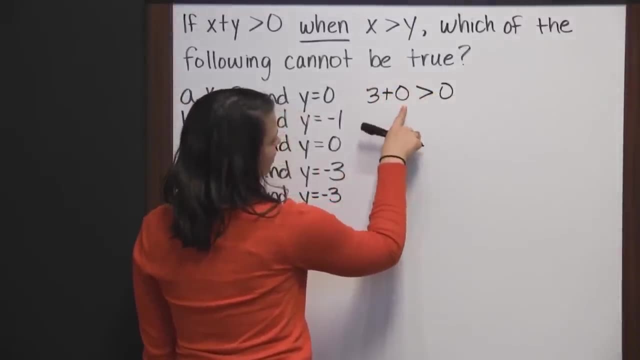 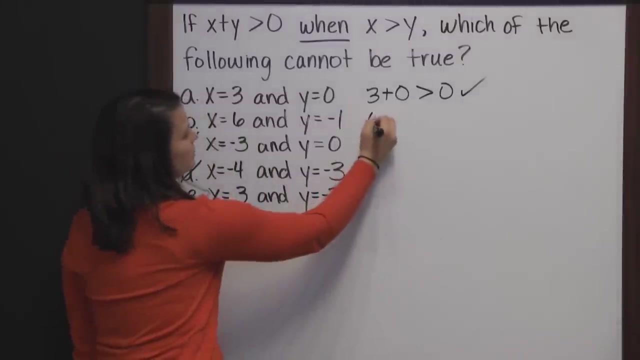 So now we need to check to see if they satisfy the first. So we'll take a. 3 plus 0 is greater than 1.. Oh, I know, greater than 0.. 3 plus 0 is 3, and that is greater than 0, so it works. b: 6 plus negative. 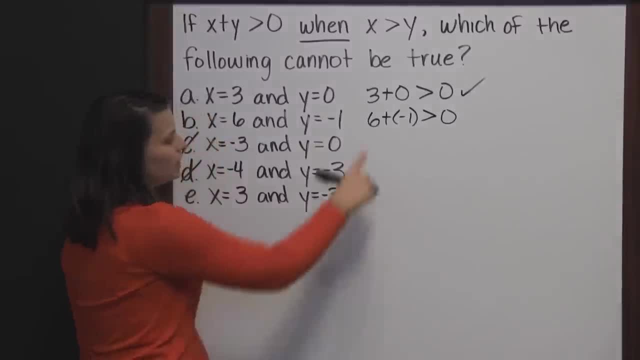 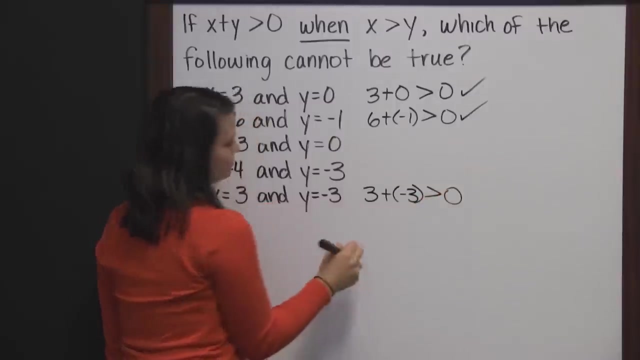 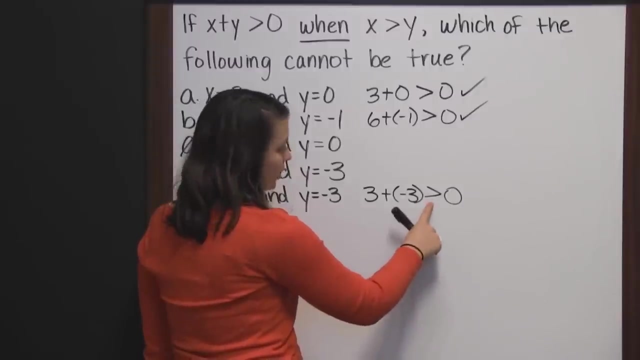 1 is greater than 0.. 6 plus negative 1 is 5, and 5 is greater than 0.. And finally, e 3 plus negative 3 is greater than 0.. 3 plus negative 3 is 0,, but 0 is not greater than. 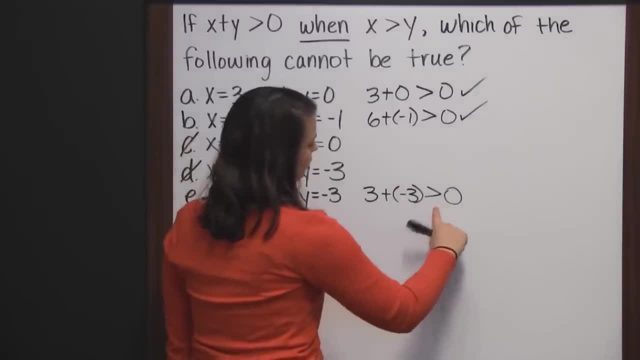 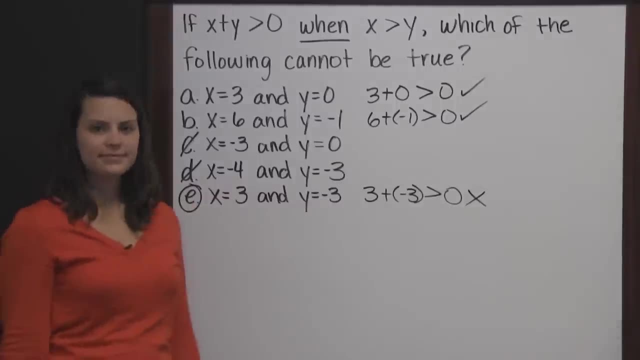 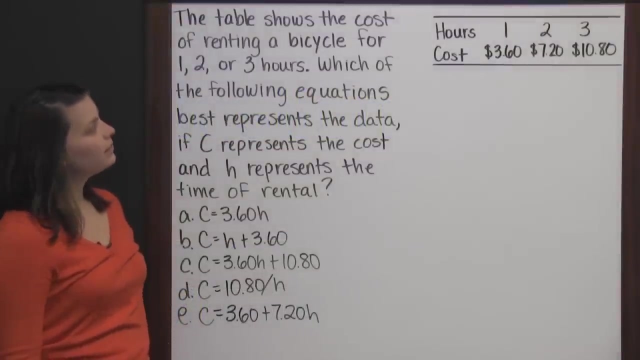 0.. 0 is simply equal to 0,, so this one is not true. So we found our answer e. The table shows the cost of renting a bicycle for one, two or three hours. Which of the following equations best represents the data? if c represents the cost and h represents 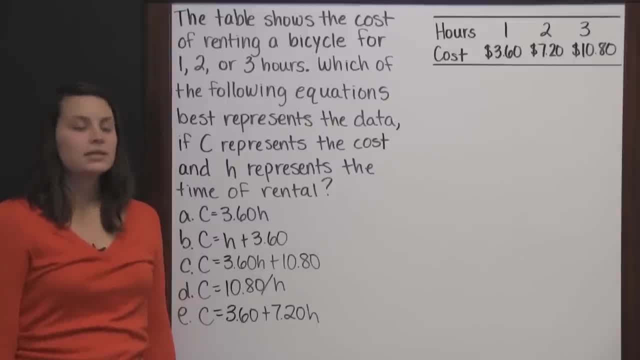 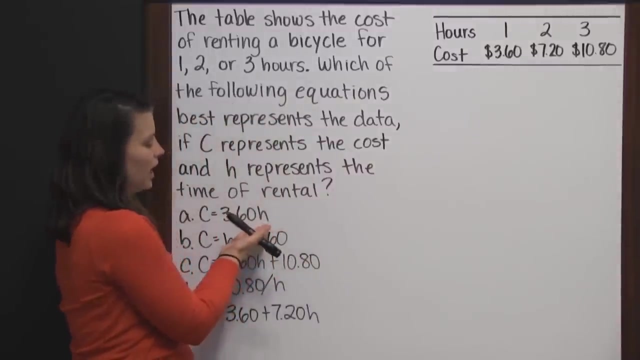 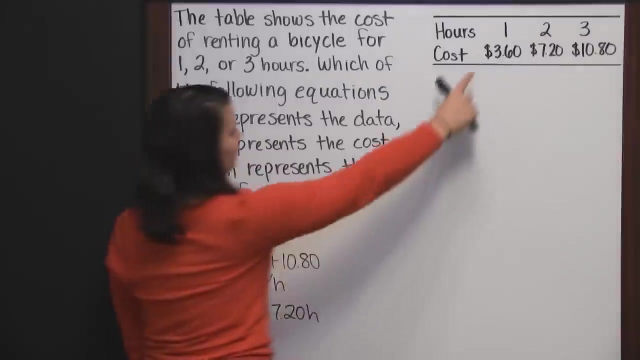 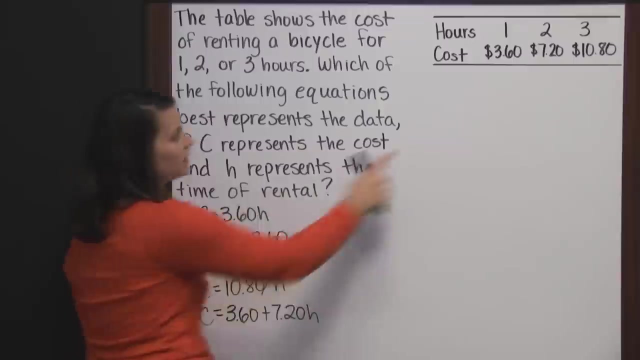 the time of rental. Since this is a multiple choice question, you could always substitute these values, Or substitute these values- values for hours- into your equation and see if you get the cost. For instance, you could replace H with 1 and you have 360 or $3.60 times 1,, which is 360, which is the cost for. 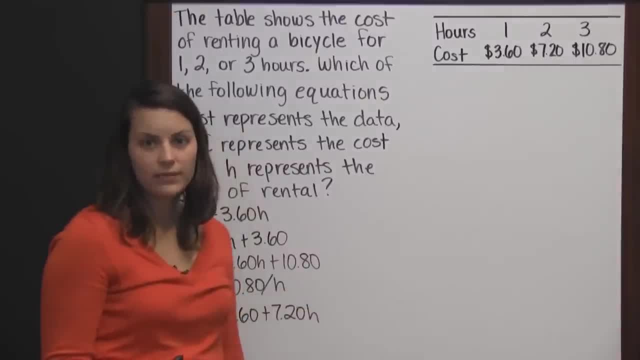 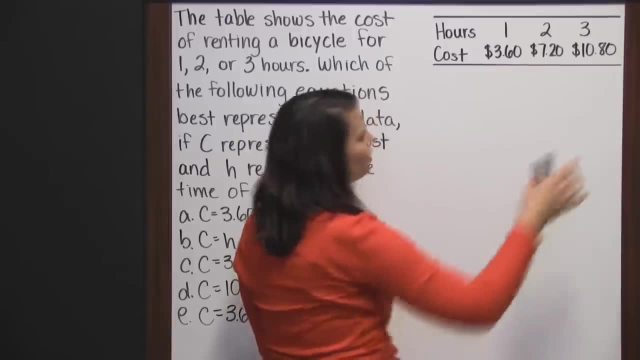 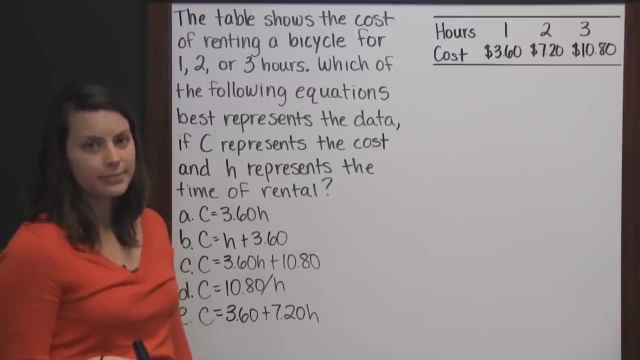 one hour, And then do the same with 2 and with 3.. Because sometimes an equation will work for one set of data but not for the other two, So you should test it on all of them. However, I'll show you how to solve this problem if it weren't multiple choice. 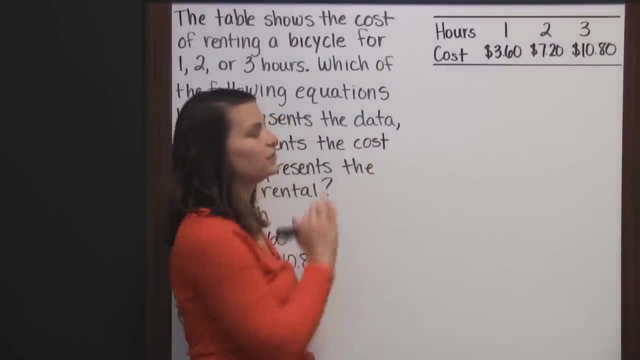 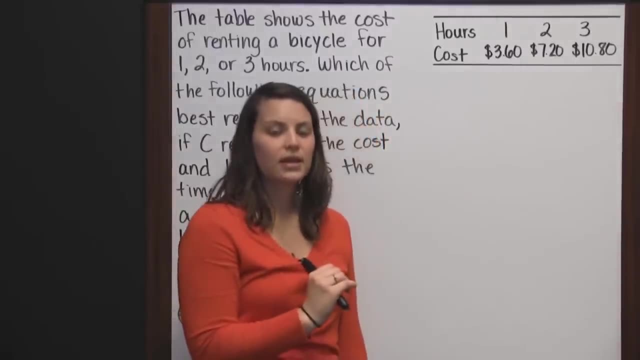 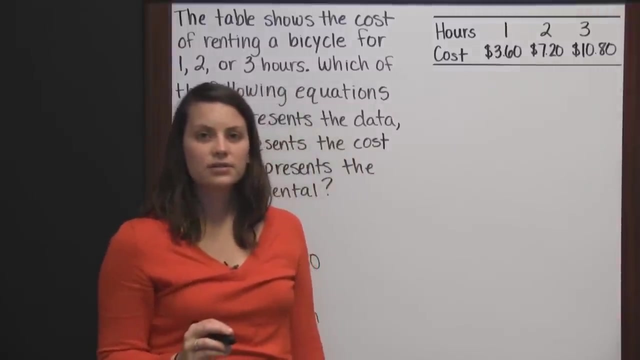 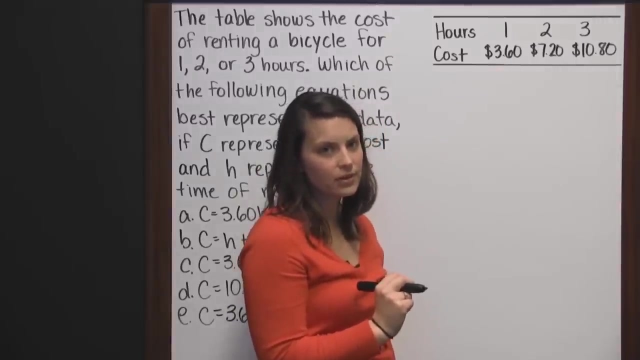 So we're going to write our own function rule using the data. First, looking at hours and cost, your cost is dependent on the number of hours that you spend on your equation, In other words, you rent the bike. Cost, then, is the dependent variable, And I want to focus. 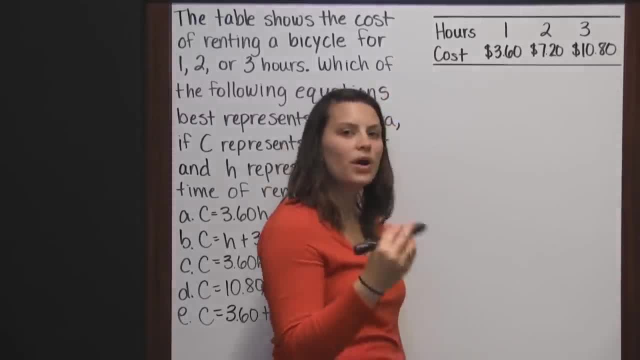 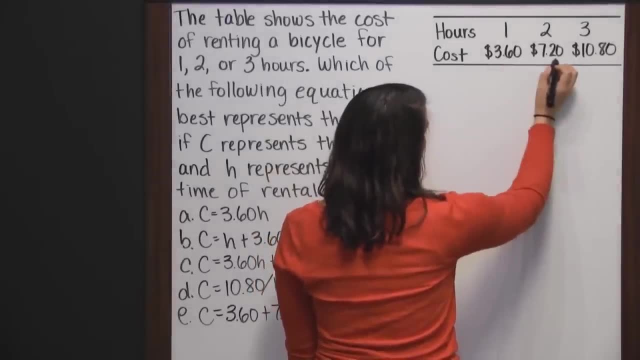 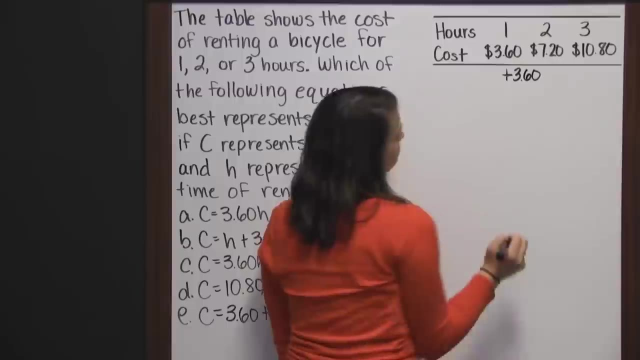 on my dependent variable and see what kind of changes are happening. So, from $3.60 to $7.20, I'm adding $3.60.. From $7.01 to $7.20, I'm adding $3.60.. From $7.01 to $7.02, I'm adding $3.16.. And then 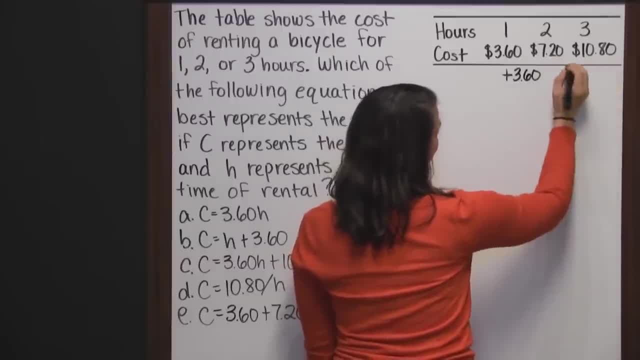 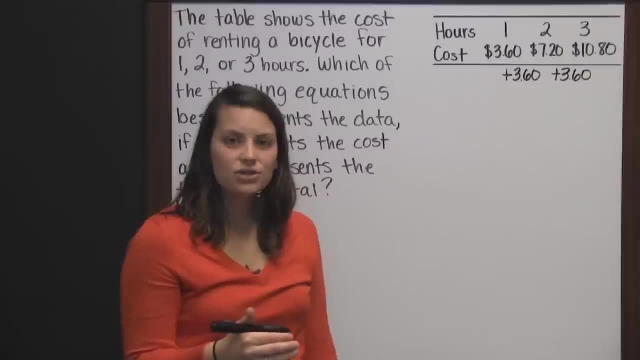 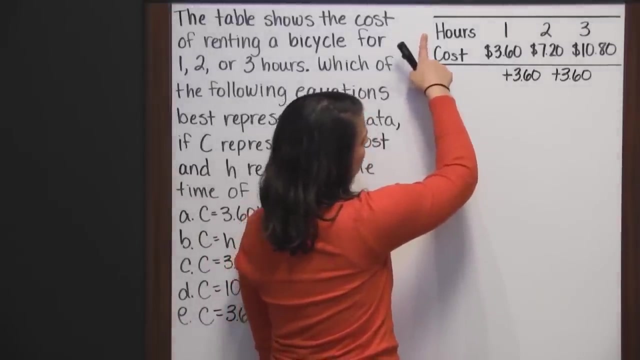 I'm adding $3.20 to $10.80.. I'm again adding $3.60.. So I can see that the change in Y is constant or the change in the cost in the dependent variable is constant. I want to now compare and see what's happening with my independent variable, my time So from. 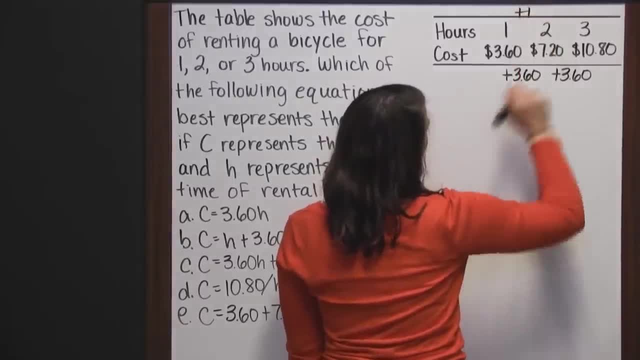 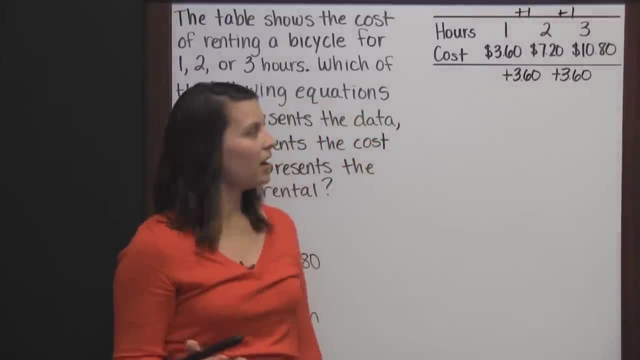 1 to 2, I increase by 1.. From 2 to 3, I also increase by 1.. So there's a constant change in my independent my time as well. This tells me that there's a linear relationship here. So to write my function: 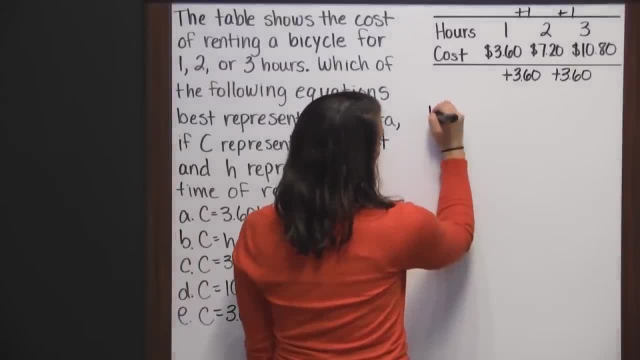 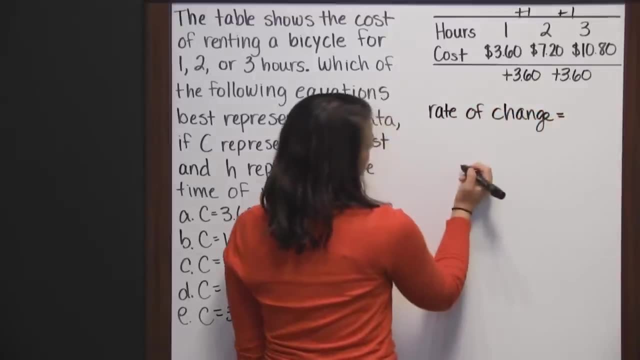 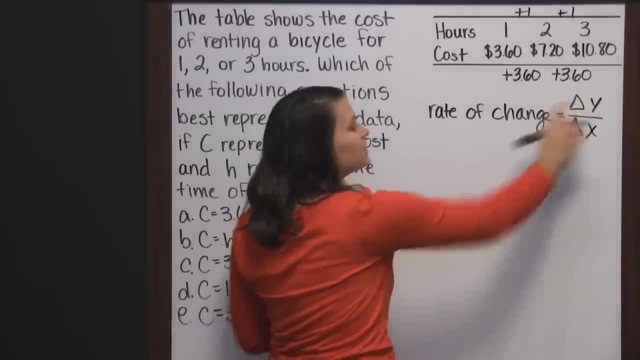 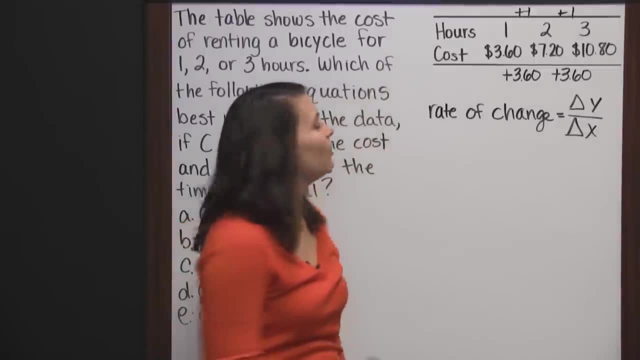 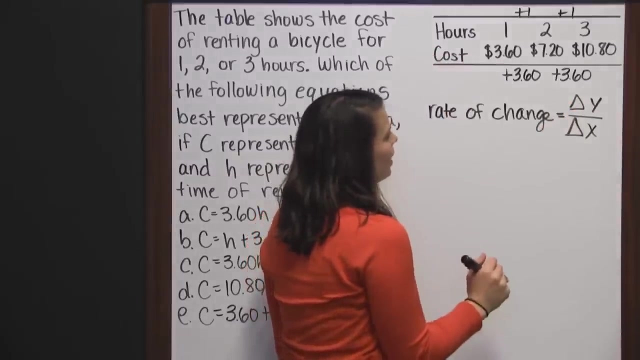 change in X and the Y, that's the dependent variable, whereas X is the independent variable And we've already established that our cost is dependent. Therefore, our cost is our Y And we've already found the change in Y: It's $3.60.. 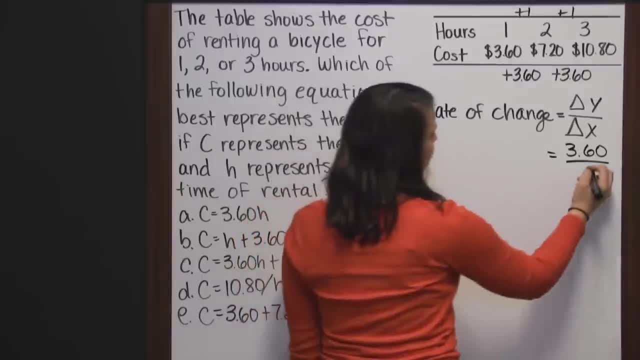 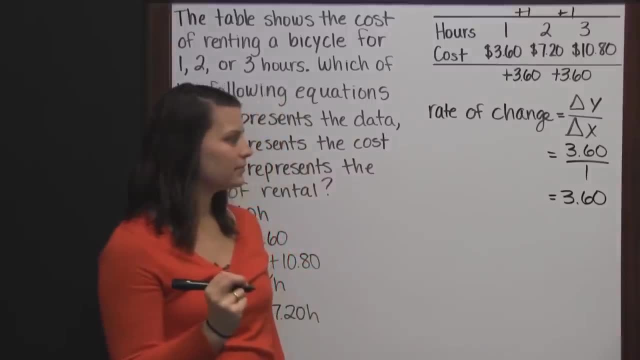 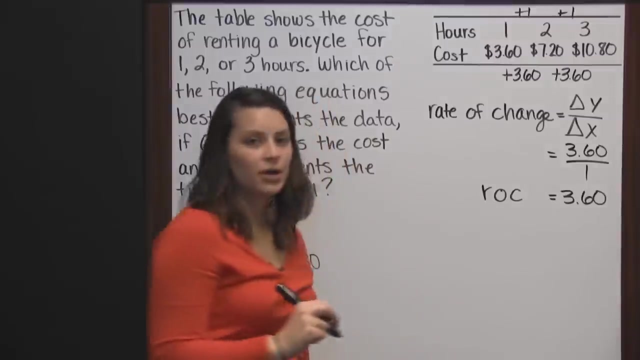 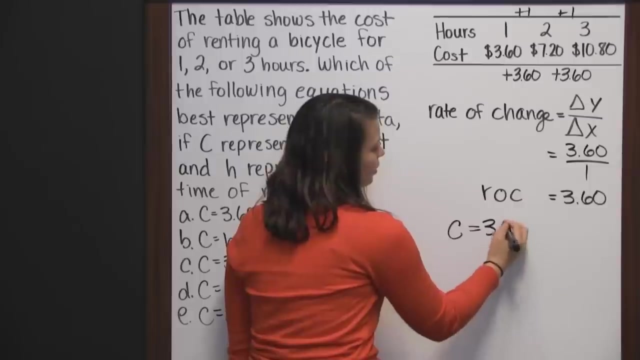 divided by the change in x, 1.. So our rate of change is simply $3.60. And that rate of change is what you're multiplying the independent variable by to get the dependent variable. So I've now found that the cost is equal to $3.60 times my independent variable of h. 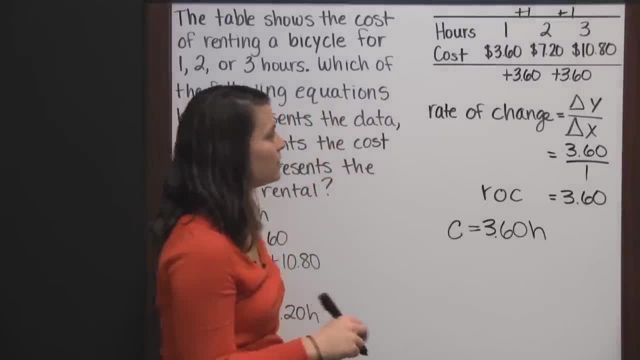 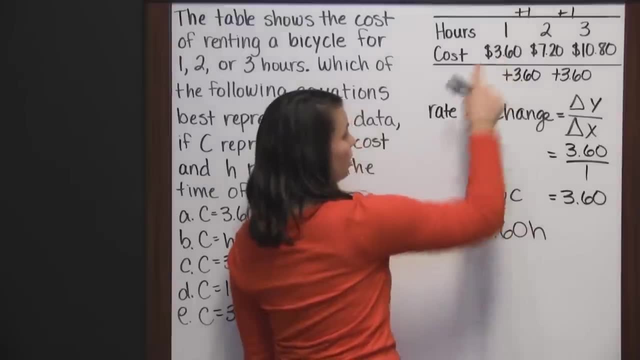 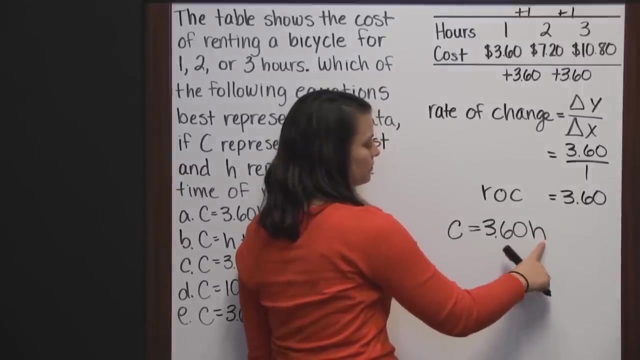 And then we can check and see if it works. So let's replace h with 1.. $3.60 times 1 is $3.60.. Try it with 2. $3.60.. $3.60 times 2 is $7.20.. 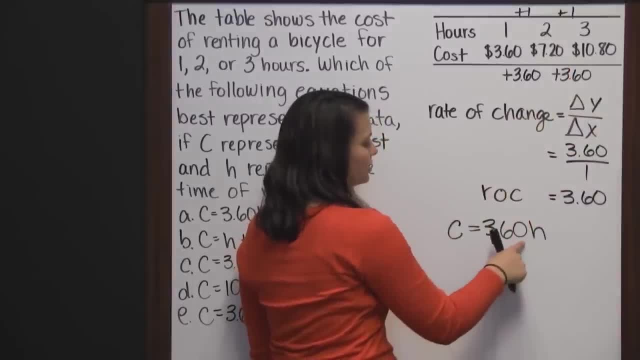 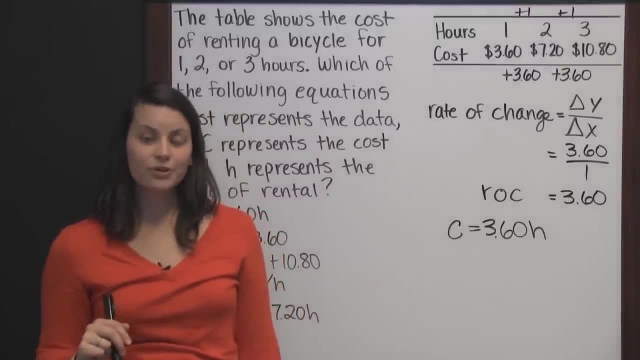 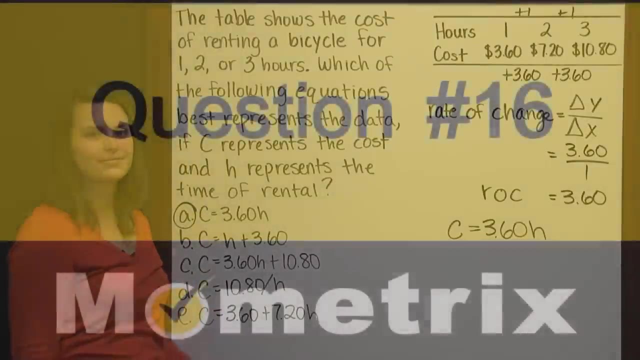 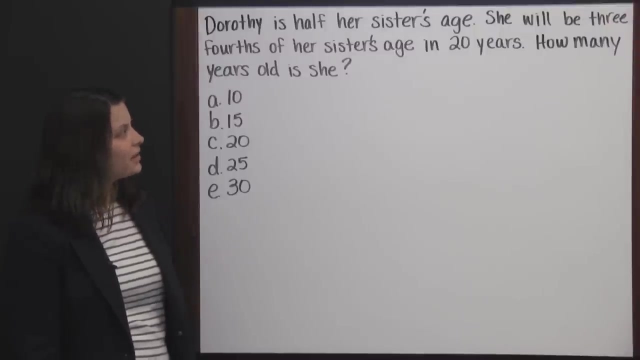 Finally, 3.. $3.60 times 3 is $10.80.. So that verifies that our function rule works for this situation and is correct. So answer A Okay. Dorothy is half her sister's age. She will be three-fourths of her sister's age in 20 years. 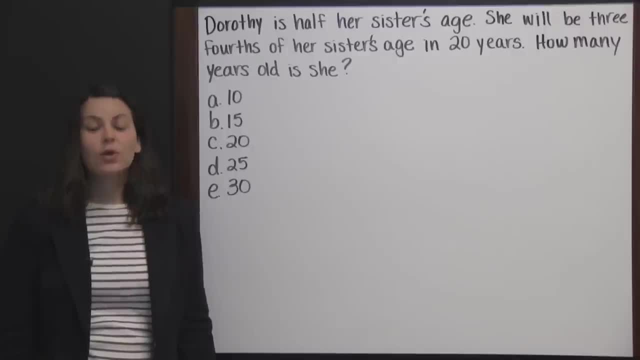 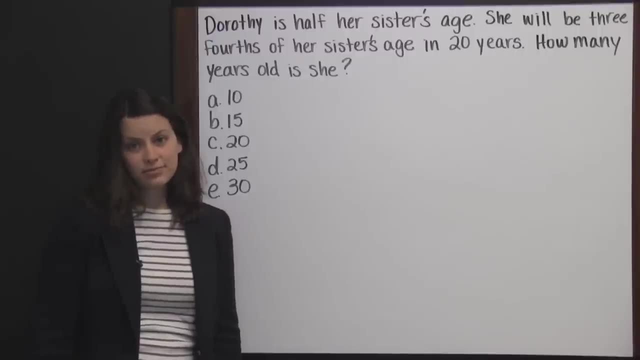 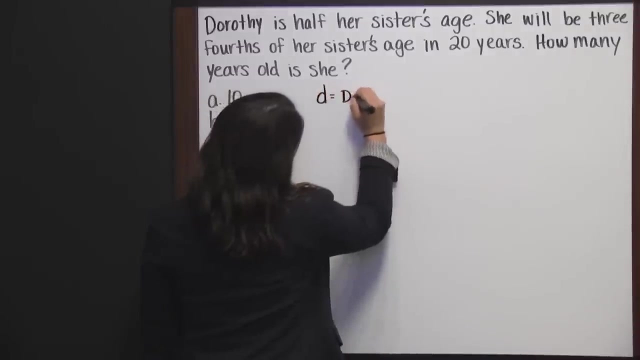 How many years old is she? We have two unknowns here: We don't know Dorothy's age and we don't know her sister's age, So I'm going to make up two variables for this. I'm going to use D for Dorothy's current age. 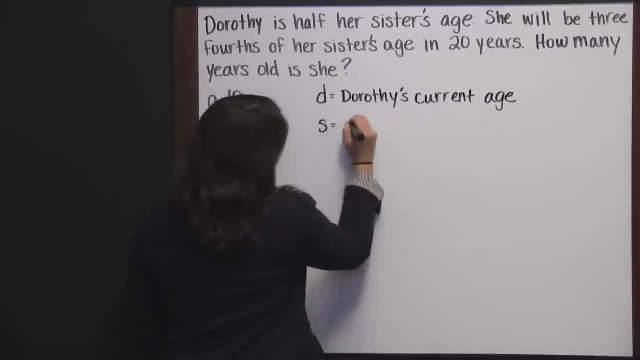 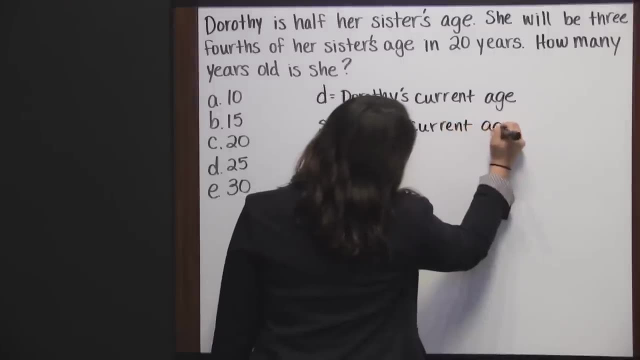 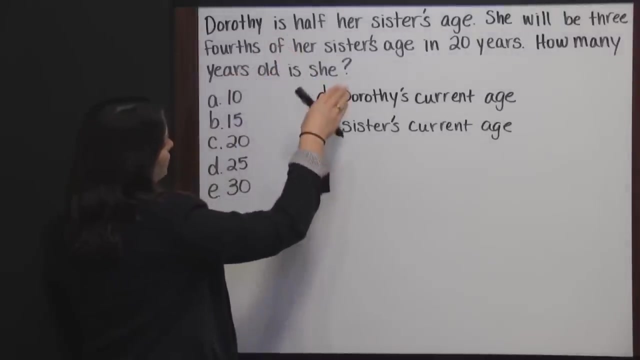 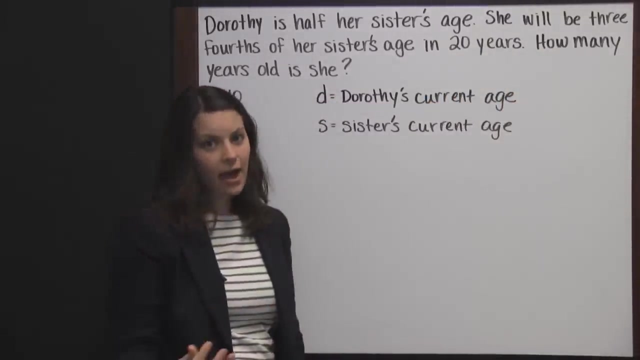 And I'll use S for the sister's current age. And I say current because they're talking about their ages now and then also their ages in 20 years. But what we want to know is how many years old she is now. So we're going to deal with their current ages. 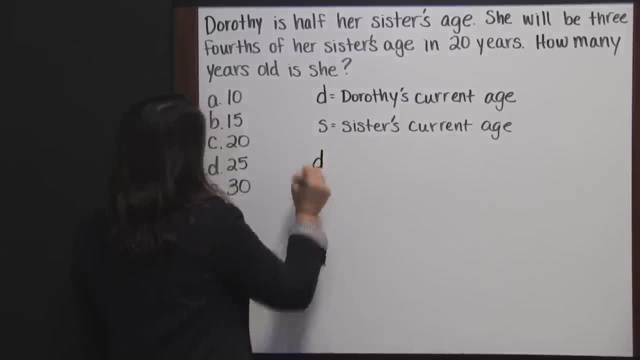 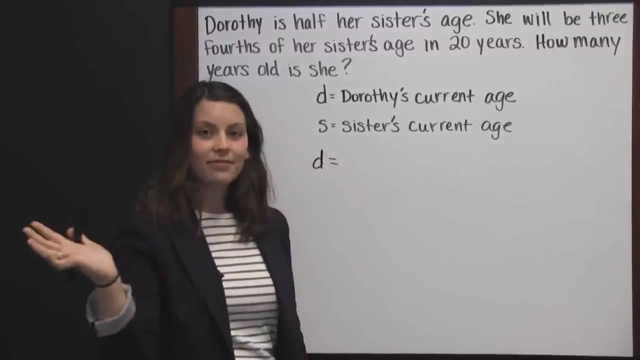 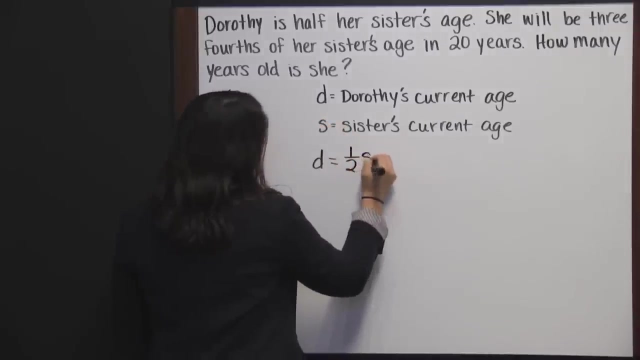 So first we have we have that Dorothy is and is in math means equals. It's one of my favorite words. I love the equals sign. So Dorothy is Dorothy equals half her sister's age, so half S. So it's. 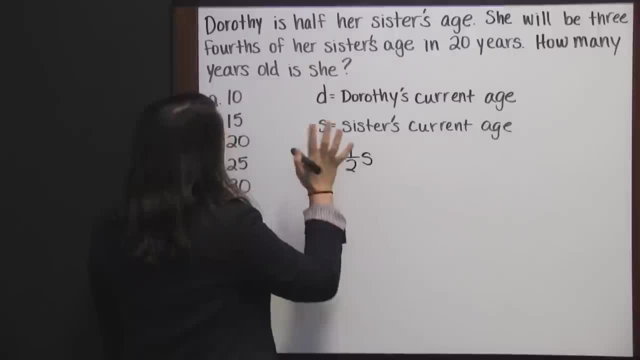 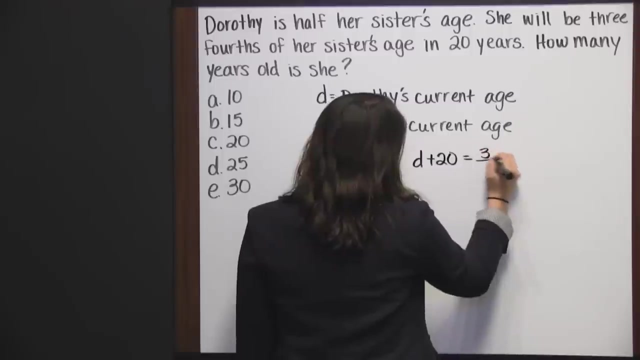 kind of like translating. You're translating from words into mathematical equations. The next sentence says: she will be. so Dorothy will be three-fourths of her sister's age in twenty years. So Dorothy, in twenty years, will be three-fourths of her sister's age. 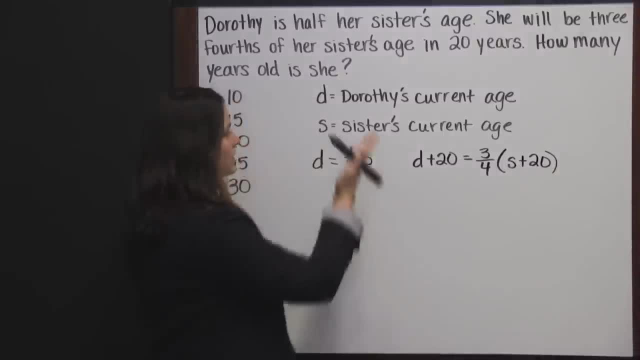 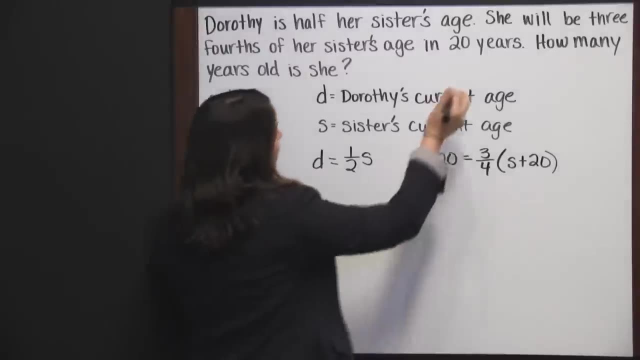 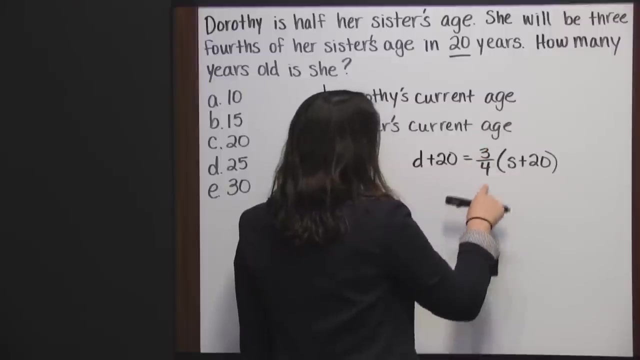 in twenty years. Remember that D and S were Dorothy and her sister's current ages. So when they talk about in twenty years, that means we have to add twenty to their current age. So Dorothy's age in twenty years. so plus twenty will be, or equals three-fourths. 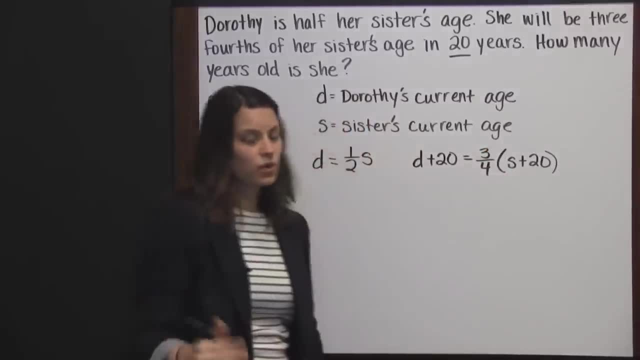 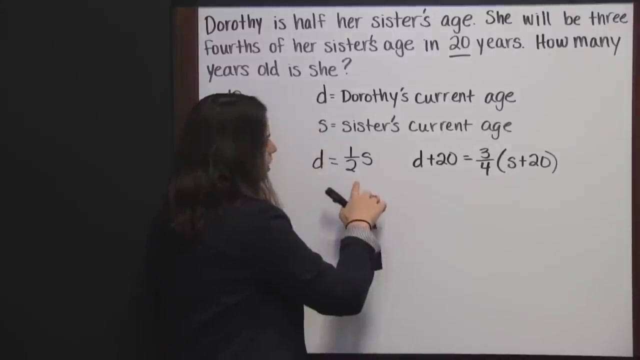 of her sister's age, also in twenty years. So we want to solve for Dorothy's age, obviously, and we can do this in lots of different ways. But the first thing I want to do is I want to notice is that, since I know that D is one-half S, I can replace D in this equation with one-half. 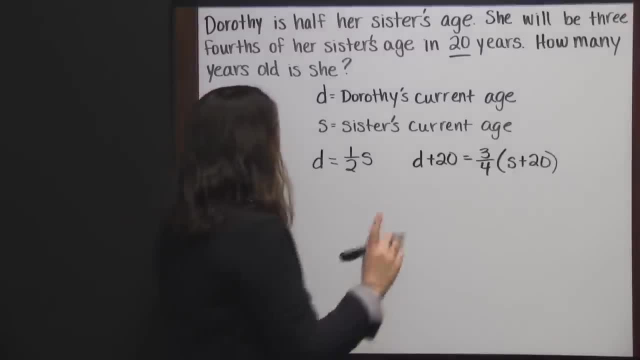 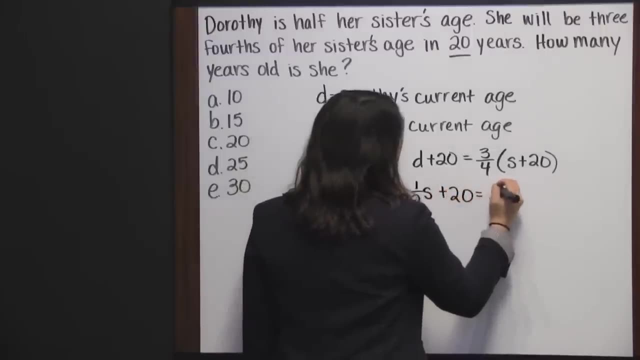 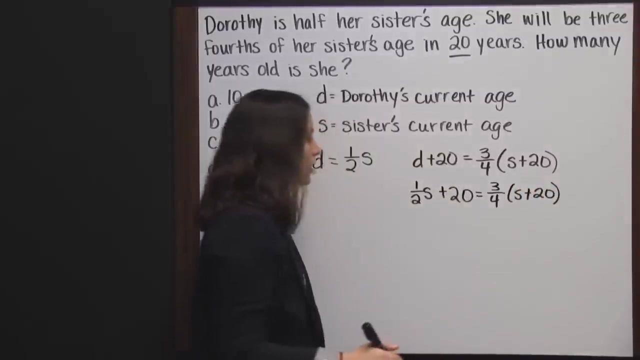 S, And that's called substitution. So that's the method I'm going to use. I'm going to replace D with one-half. S plus twenty equals three-fourths times the quantity S plus twenty. Well, from here, lots of options for solving. The first thing I think about is really, I just want to get. 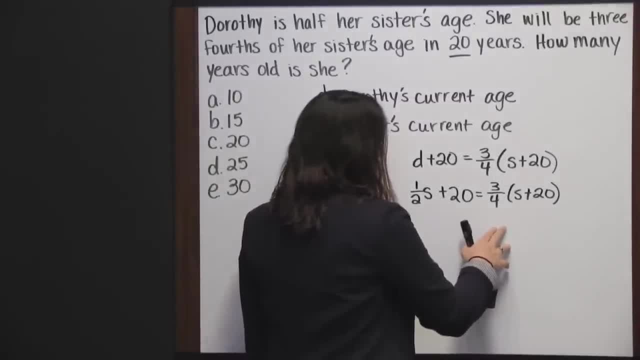 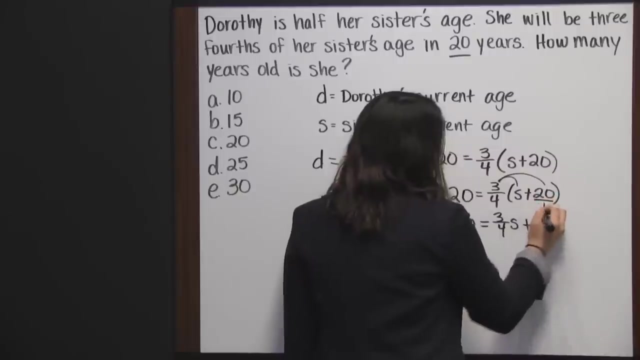 rid of this fraction, this 3 fourths. I think I'll start by distributing the 3 fourths to what's inside my parentheses. I have: 1 half s plus 20 is equal to 3 fourths s plus, and then, with the 3 fourths and the 20,, I can put 20 over 1, and I can simplify multiplying. 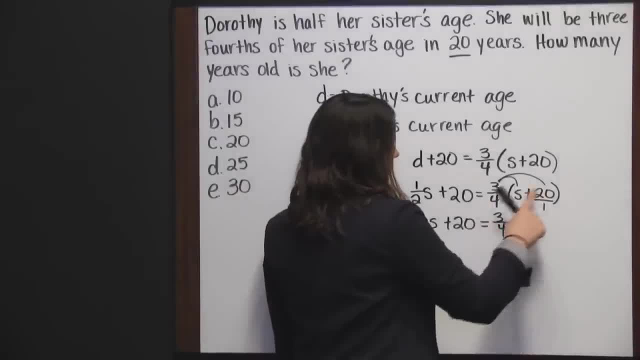 these numbers by cross-canceling 4 and 20.. I'm simply multiplying two fractions together, so I can use this shortcut. I'm going to divide both 4 and 20 by 4.. 4 divided by 4 is 1, and. 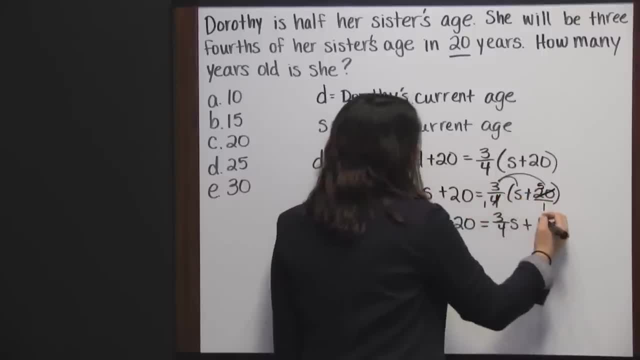 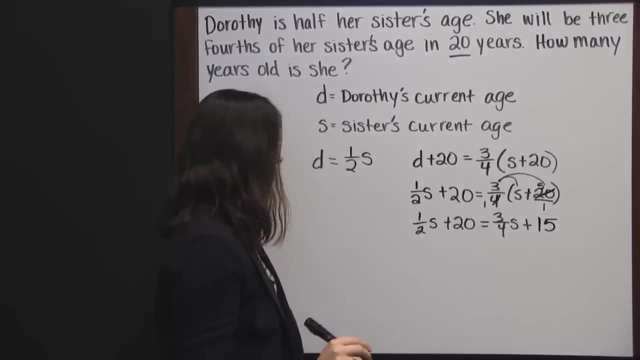 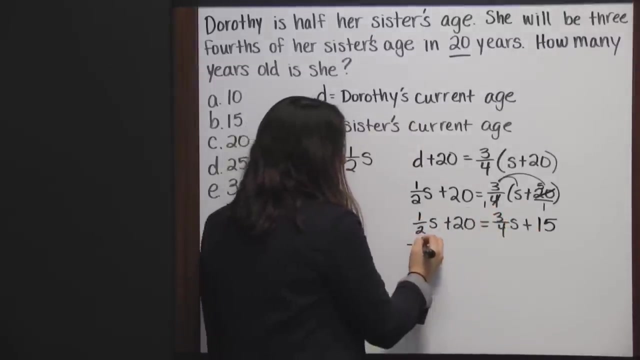 20 divided by 4 is 5, so 3 times 5 is 15.. Three-fourths of 20 is 15.. That makes sense. We need to get all of our variables on the same side. To do that, I'm going to subtract 1 half s from both sides, 1 half s minus 1. 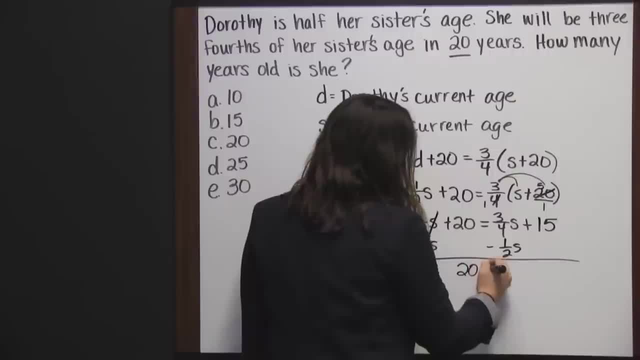 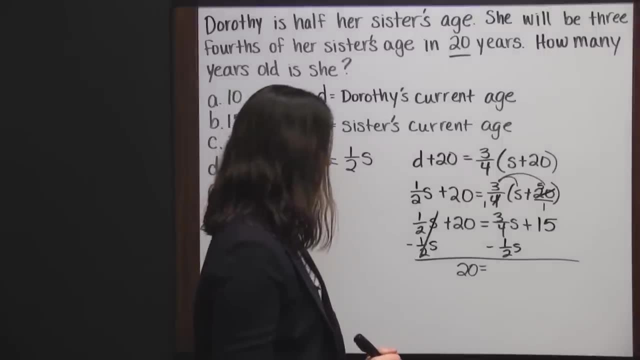 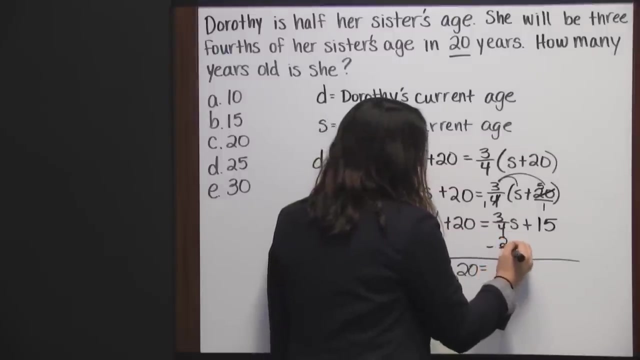 half s is 0.. I'm going to bring down 20, and that equals: Now, to subtract fractions, I have to have common denominators, So one-half is also two-fourths. so I'm going to change one-half to two-fourths. 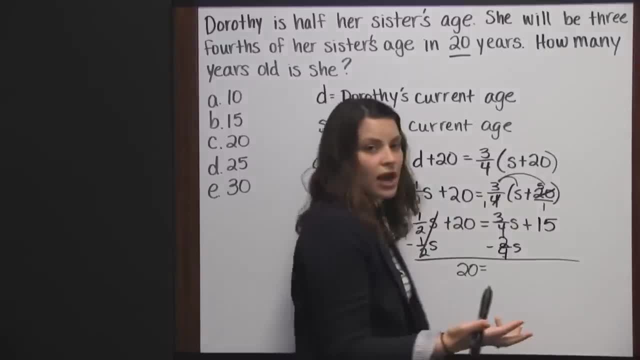 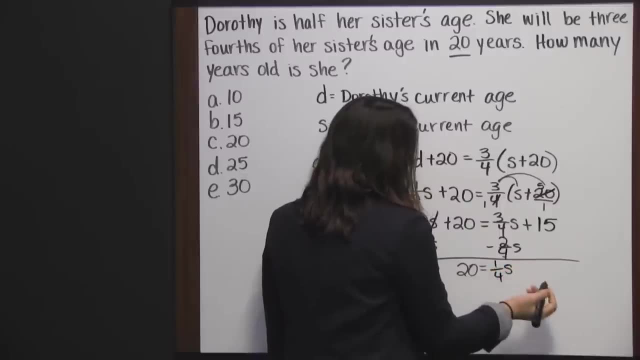 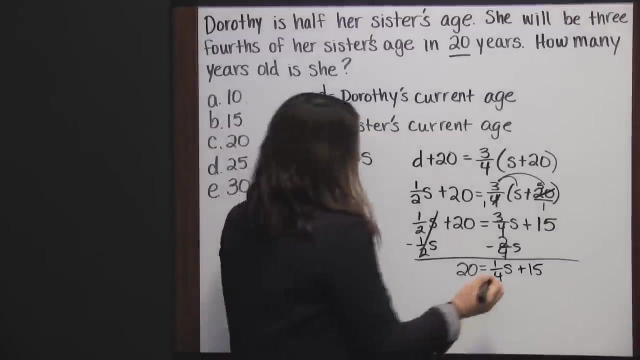 so that I can subtract these. And then, when I subtract, you just subtract the numerators: Three minus two is one and your denominators stay the same: one-fourth s plus 15.. Next I need to subtract 15 from both sides. 20 minus 15 is five, and five is a fourth of. 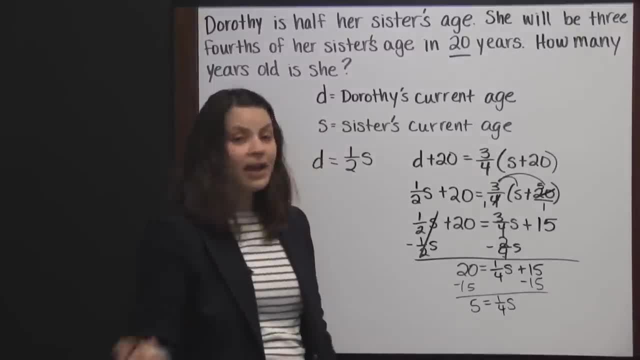 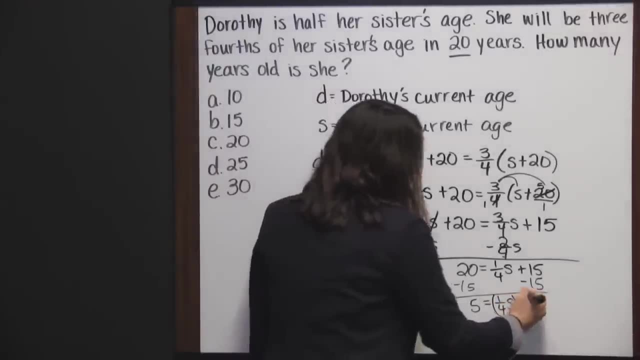 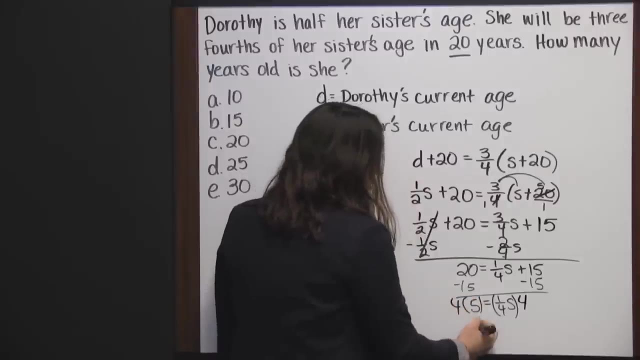 the sister's age. So finally, I need to multiply both sides by the multiplicative inverse of a fourth, which is four over one or just four. So multiply both sides by four. Four times five is 20, and 20 is her sister's age. A fourth of four is one, so we're left. 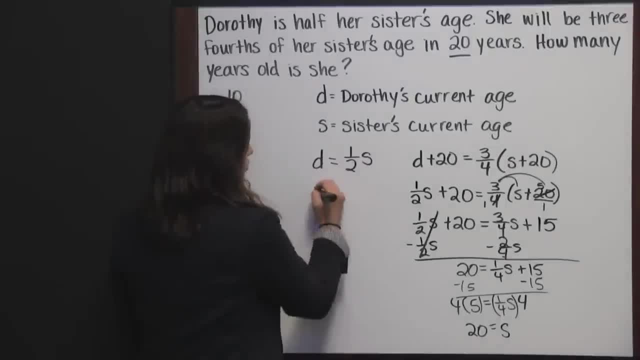 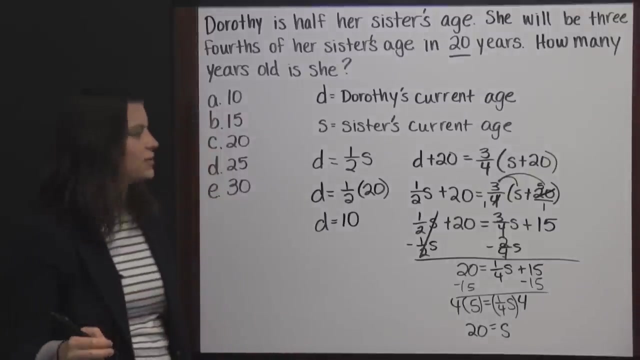 with s the sister's age. Well, remember that Dorothy is half of her sister's age. so since we now know her sister's age is 20, we know that Dorothy is half of that and half of 20 is 10.. So that means Dorothy is 10 years old. 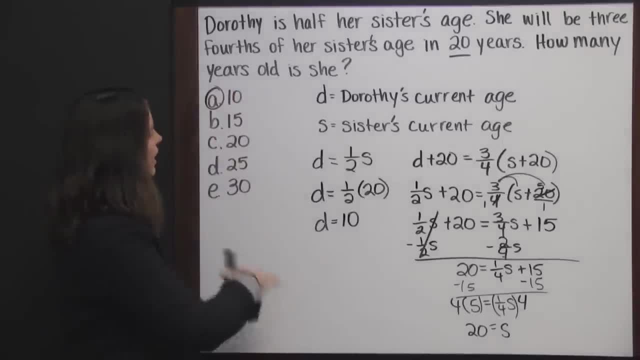 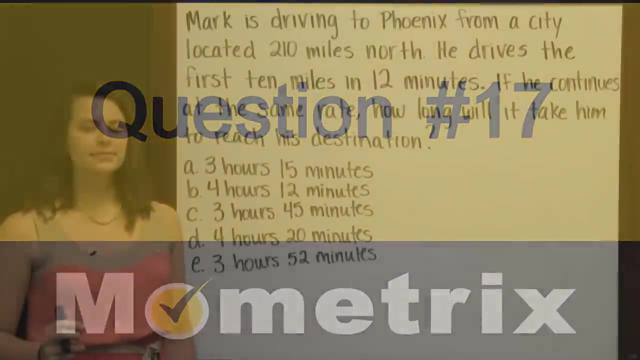 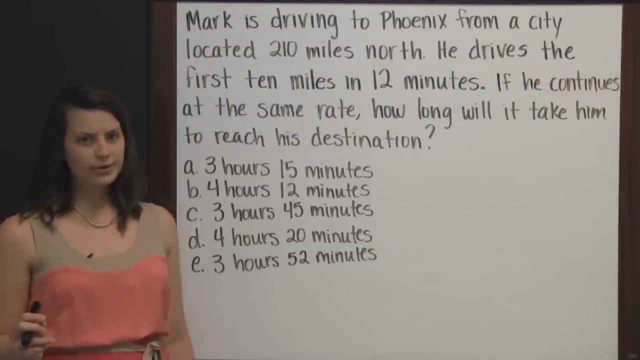 You could have solved this also by just kind of playing with the numbers, playing with the answers and seeing which ones would work with the information you were given. but I always love to solve a good algebra problem. Mark is driving to Phoenix from a city located 210 miles north. He drives the first 10 miles. 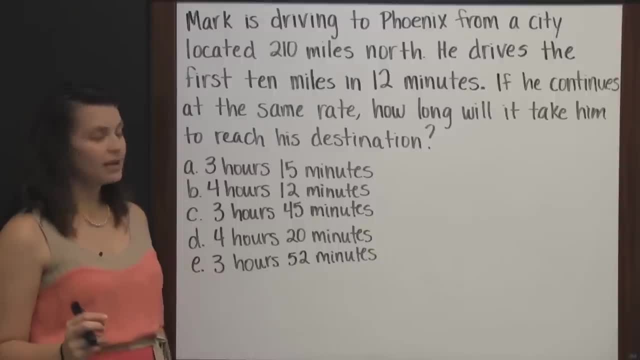 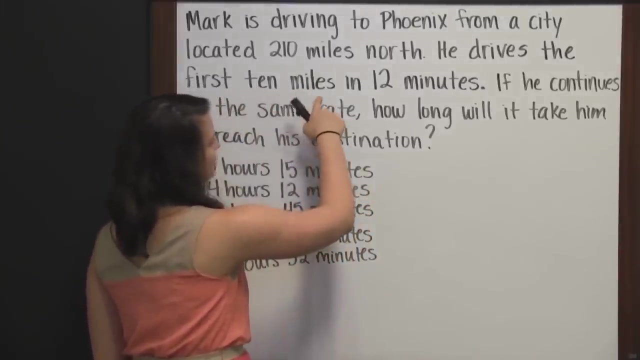 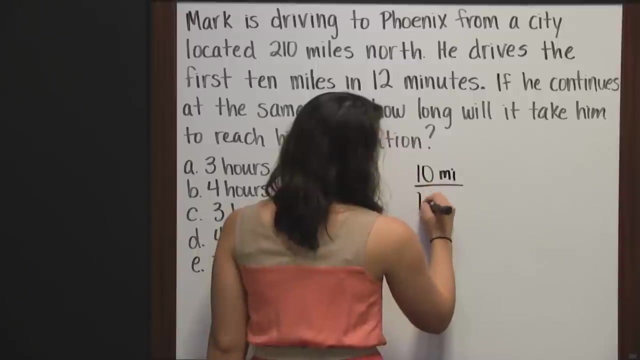 in 12 minutes. If he continues at the same rate, how long will it take him to reach his destination? We can use a proportion to solve this problem. We know that the first 10 miles took him 12 minutes, so that's one ratio: 10 miles took. 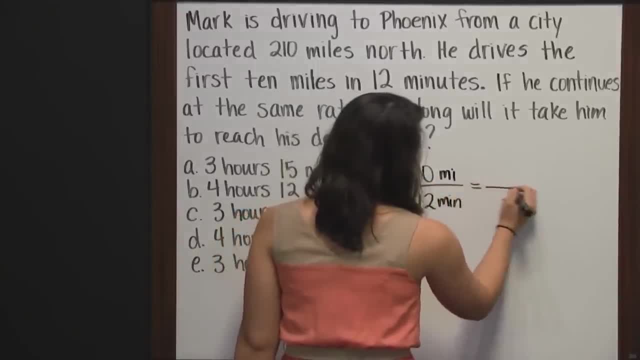 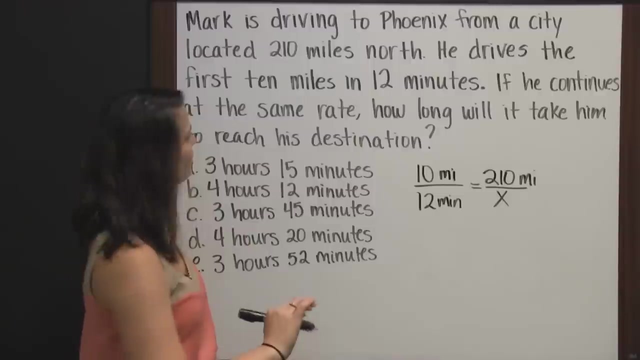 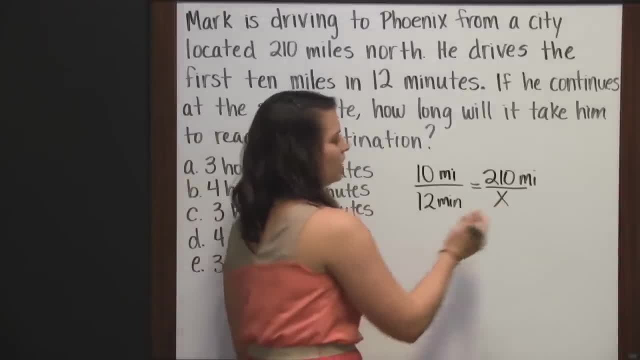 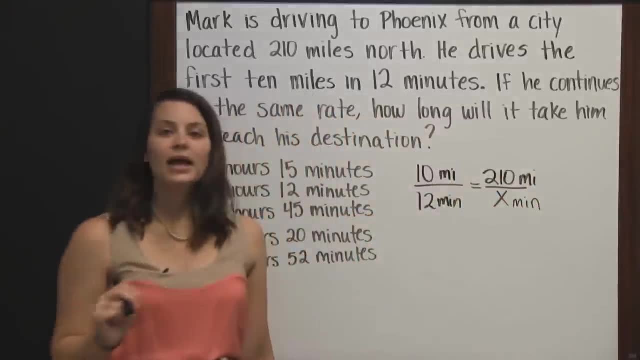 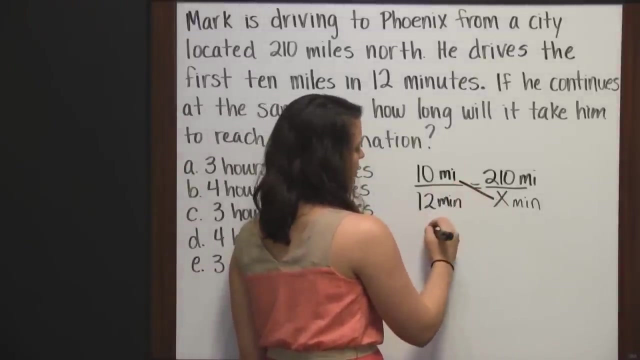 to solve and find how long it's going to take him in minutes, Miles to minutes, miles to minutes. And to solve a proportion we cross multiply And to solve a proportion we cross multiply. So 10 times X is 10X equals 12 times 210.. 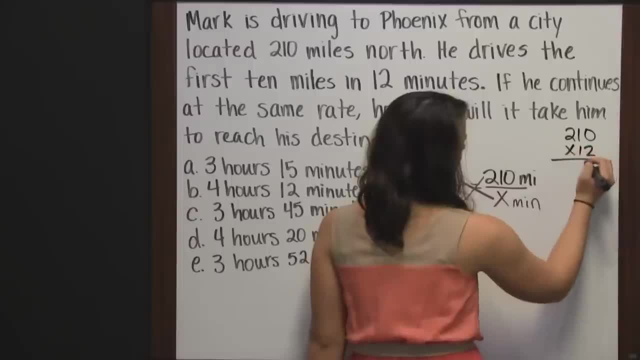 So I'm going to multiply that right over here: 2 times 0 is 0.. 2 times 1 is 2.. 2 times 2 is 4.. 0 placeholder- 1 times 0 is 0.. 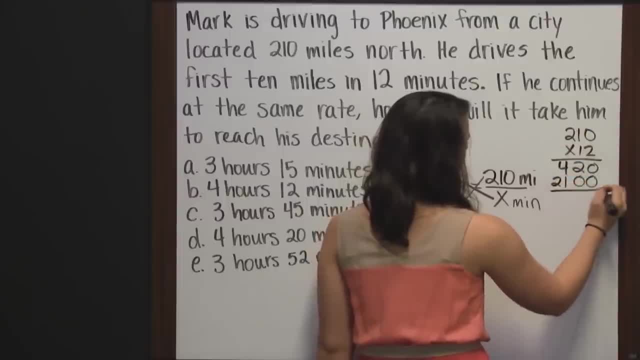 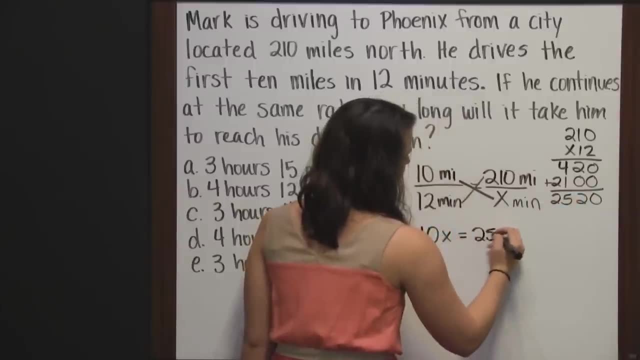 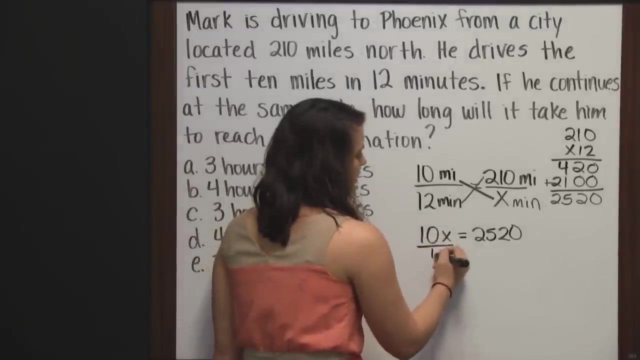 1 times 1 is 1.. 1 times 2 is 2.. And we add these together: 0,, 2,, 5, 2,, so 2,520.. And then to solve for X, we need to divide both sides by 10.. 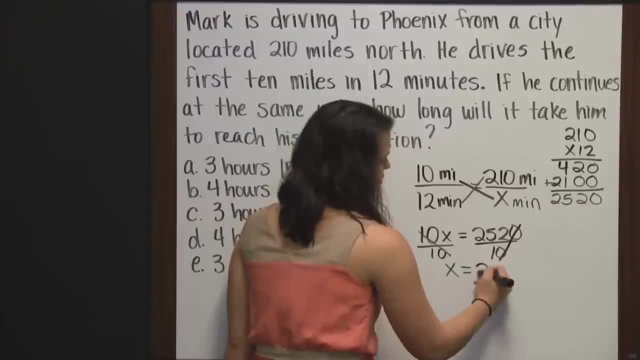 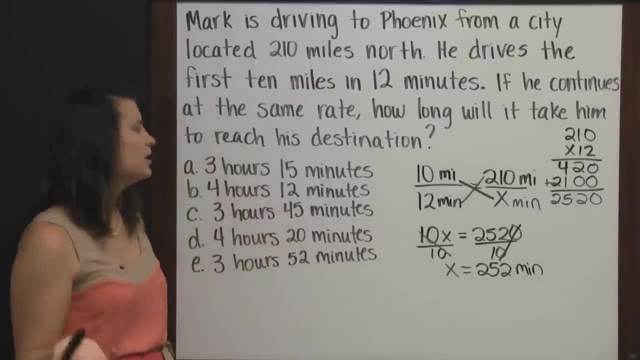 So X equals- I'm going to just cancel a 0 here. 252.. 252- what Well, 252 miles, 252 miles, 252 miles, 252 minutes. But, as you can see, our answers aren't in minutes. 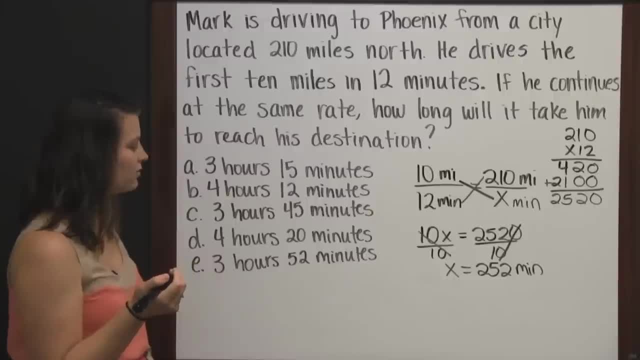 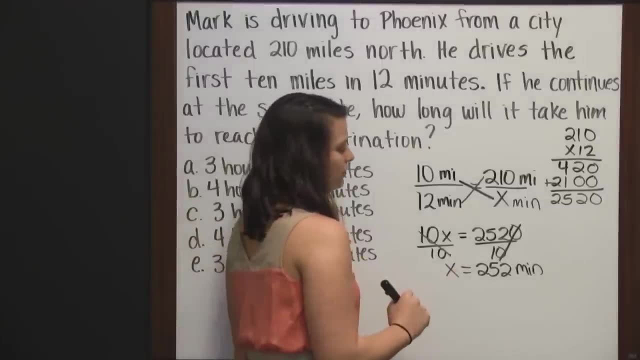 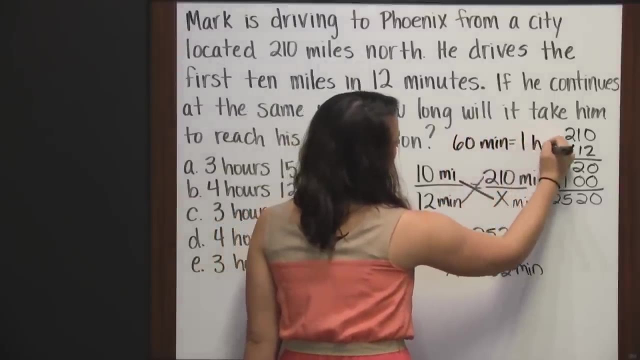 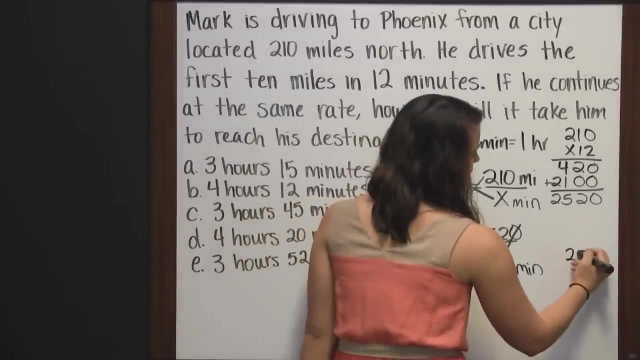 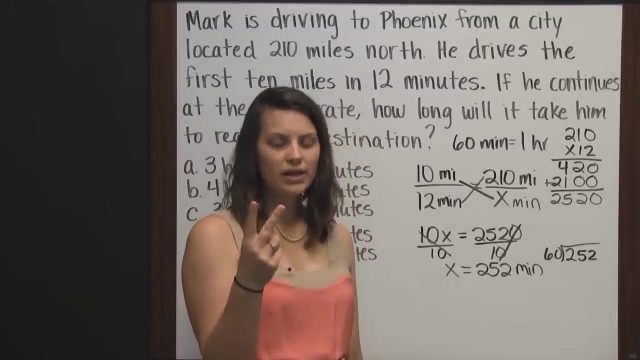 They're in hours and minutes, So we need to figure out just how many hours and then leftover minutes there are in 252 minutes. And since there are 60 minutes in one hour, I need to divide 252 by 60.. So 252 divided by 60, so 60 does not go into 25, 60 goes into 252, 60,, 120,, 180,, 240. 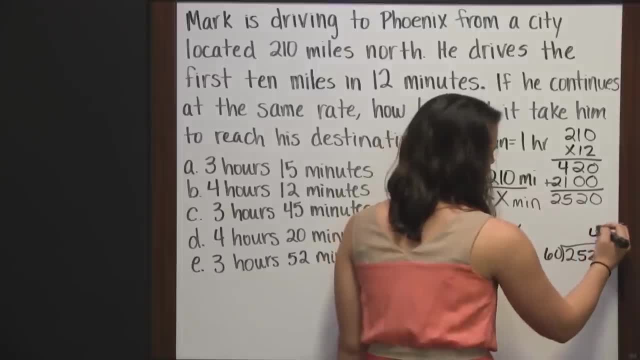 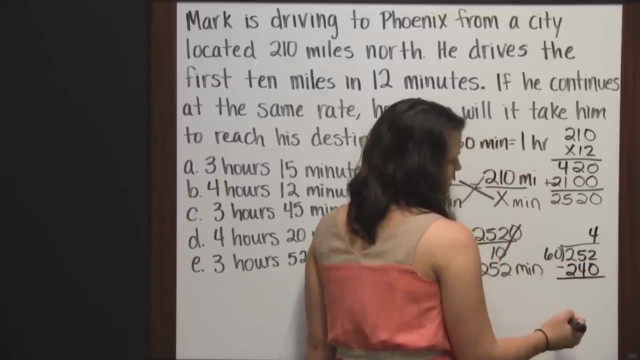 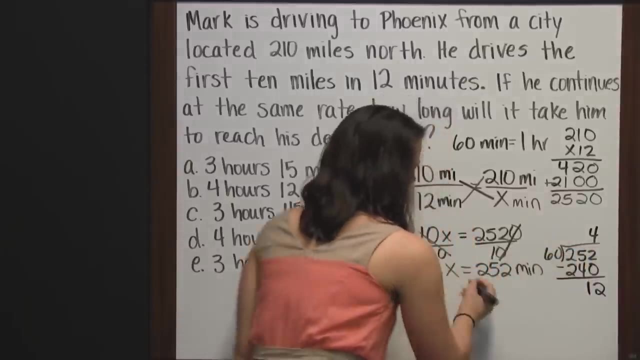 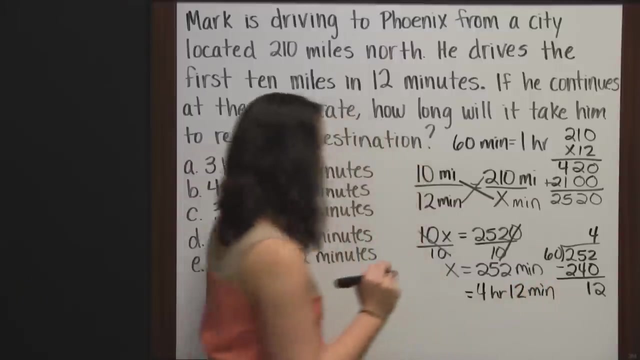 So 4 times, because 4 times 6 is 24, and 4 times 6d is 240.. We subtract and we get 12 that's left over. So that means 252 minutes is 4 hours and 12 minutes left over. 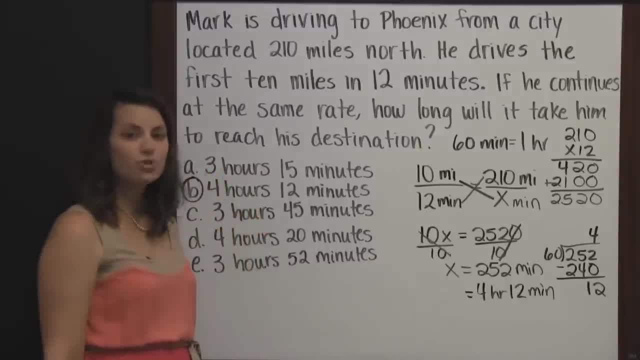 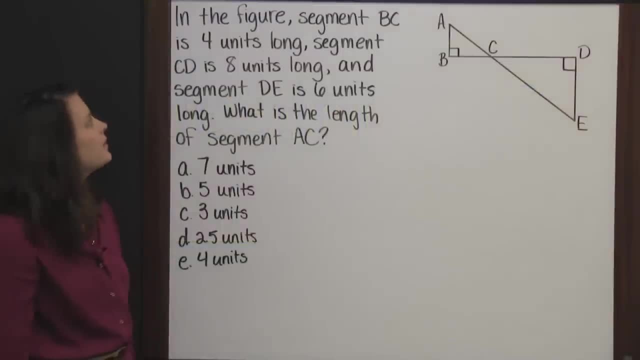 So that is answer choice B: 4 hours and 12 minutes. In the figure, segment BC is 4 units long, segment CD is 8 units long and segment DE is 6 units long. What is the length of segment AC? 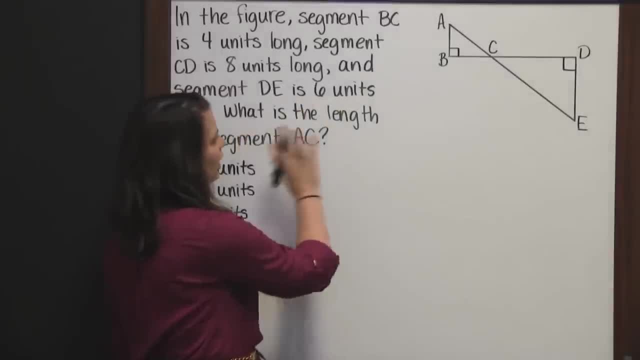 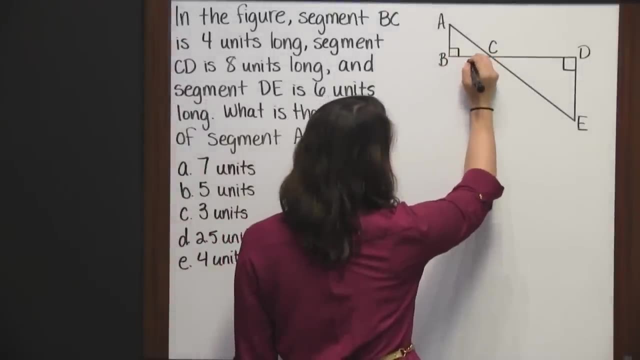 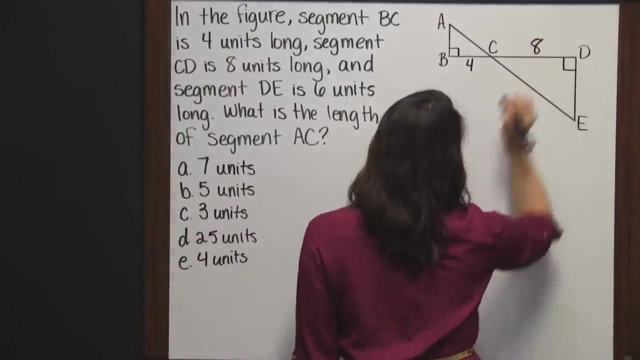 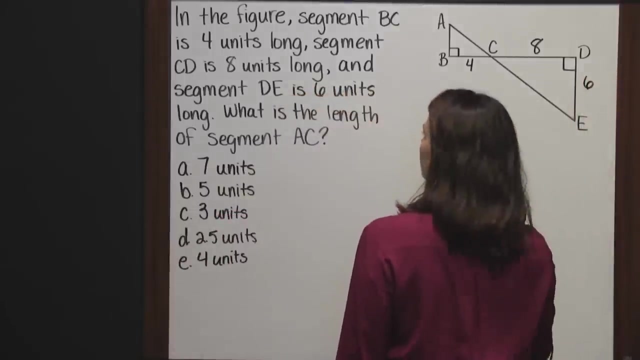 The first thing I'd like to do is take this information and actually put it on my picture. So segment BC is 4 units long. here's segment BC. it's 4.. Segment CD is 8 units long. CD is 8, and segment DE is 6 units long. DE is 6 units long. 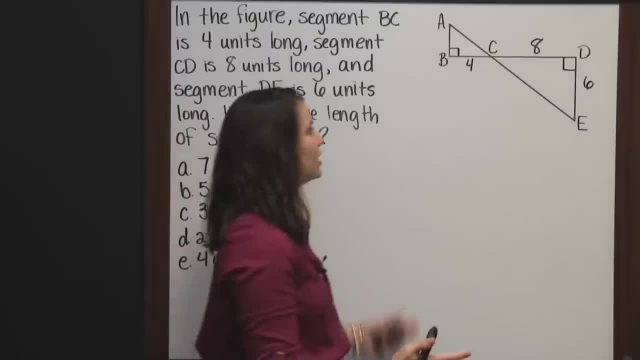 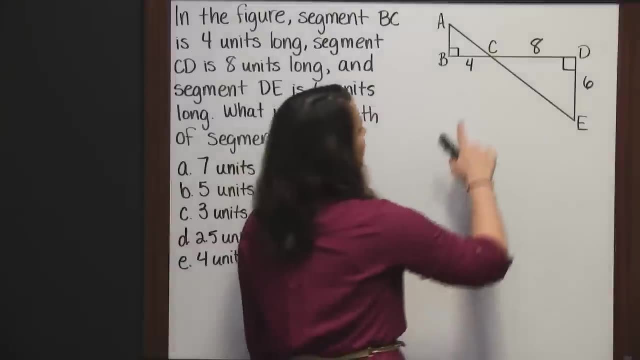 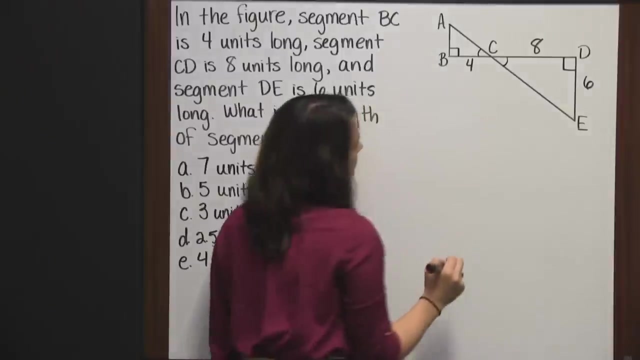 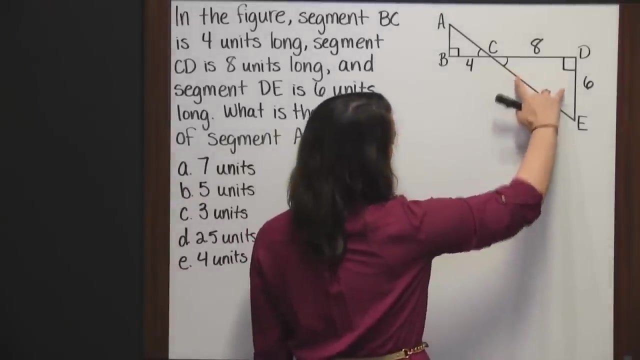 These triangles are not congruent and that's obvious. if you're looking at them, You can see this triangle is smaller than the other one. However, these right angles are congruent. These vertical angles are congruent, Since two angles of this triangle are congruent to two angles of the other triangle. 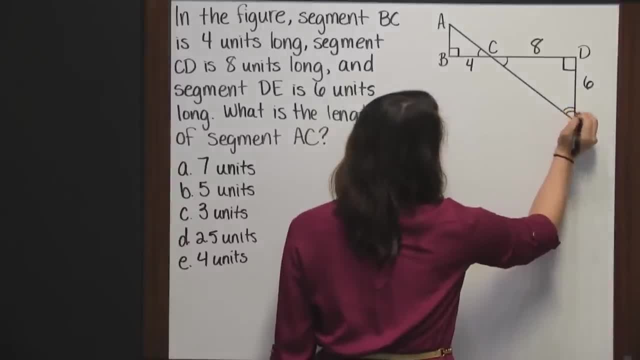 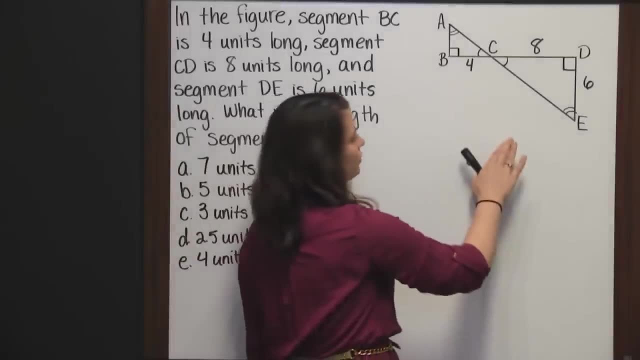 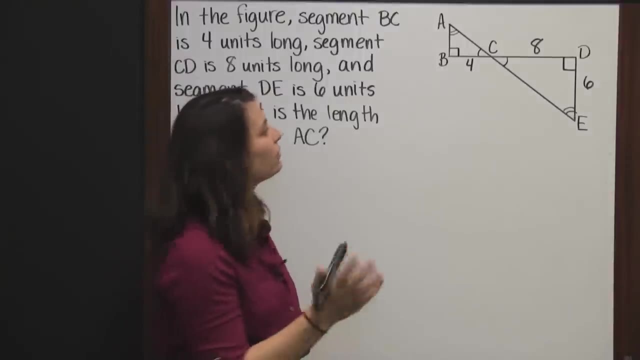 that means that the third angles, angle E and angle A, are congruent to each other. Therefore, these two triangles are similar to each other because all three of them are congruent. All three of their corresponding angles are congruent to each other. 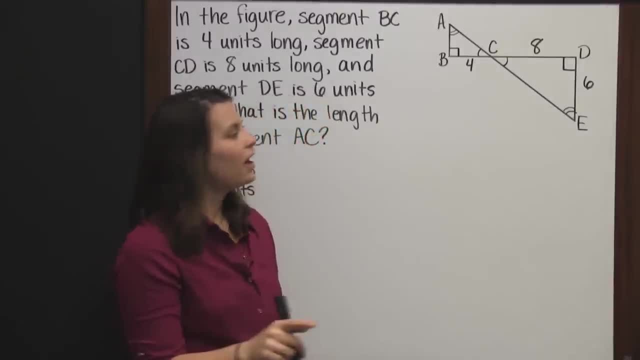 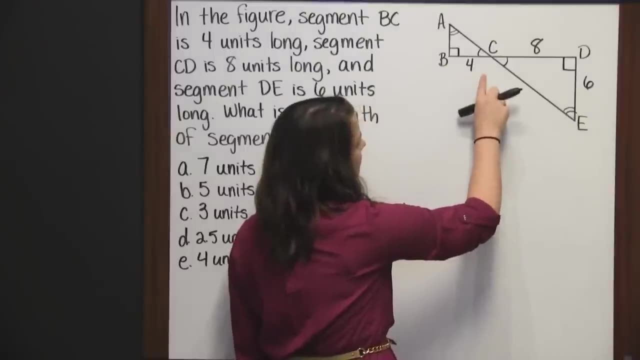 Since these triangles are similar, that means that their corresponding sides are proportional. You see that segment BC is half of segment CD. 4 is half of 8.. If we can find the length of segment CE, then we know the length of segment AC is 1.. 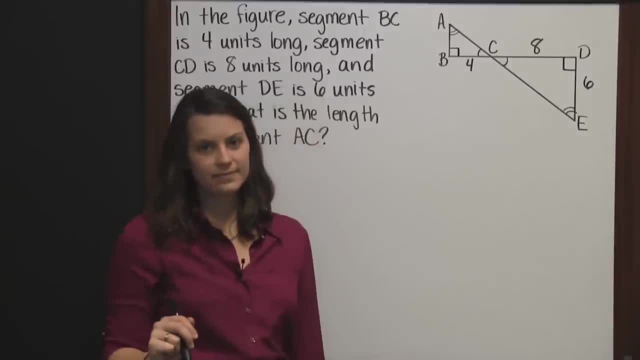 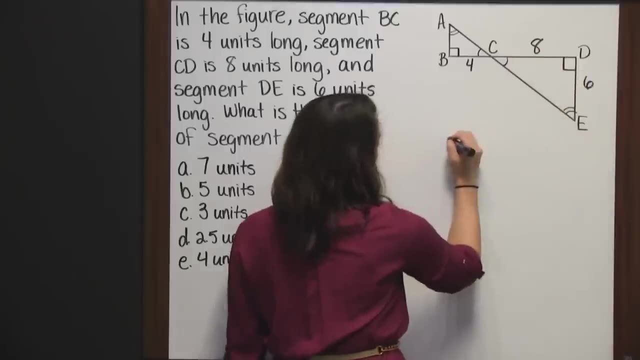 The length of segment AC is half of that. We're going to find the length of segment CE using the Pythagorean Theorem: a squared plus b squared equals c squared. We have our two legs: 8 squared plus 6 squared equals c squared. 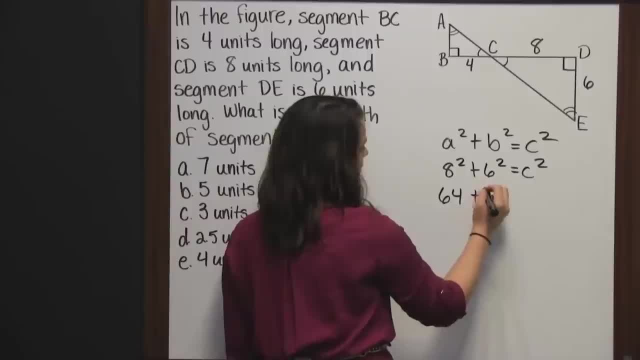 8 squared is 64, plus 6 squared is 36, equals c squared. 64 plus 36 is 100, equals c squared. Then to solve for c we need a square root both sides. The square root of 100 is 10, and the square root of c squared is c. 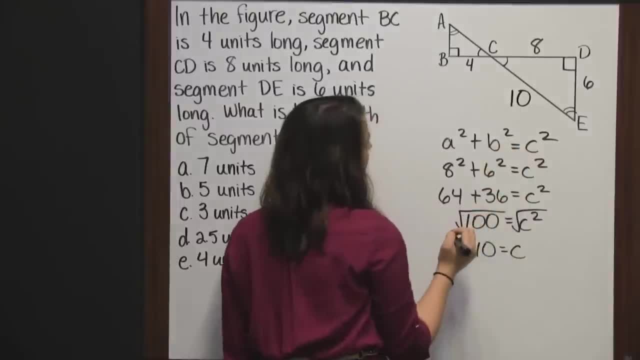 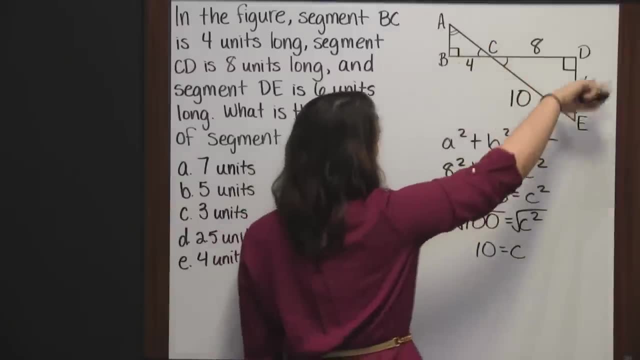 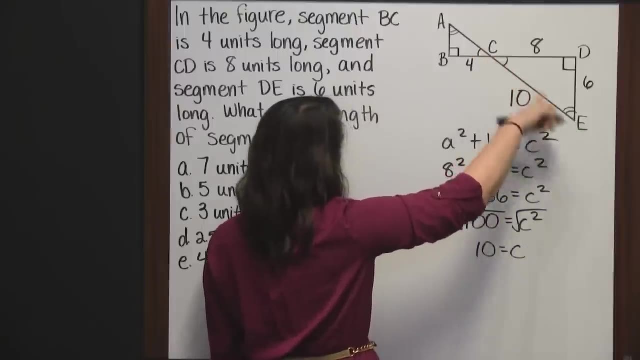 So the length of segment CE is 10.. And again, the lengths of the sides of triangle ABC are half the corresponding sides of triangle CDE. So since the length of segment CE is 10, that means that the length of segment AC is half of that, or 5.. 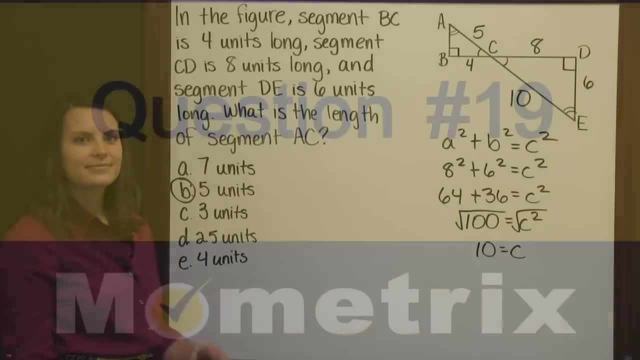 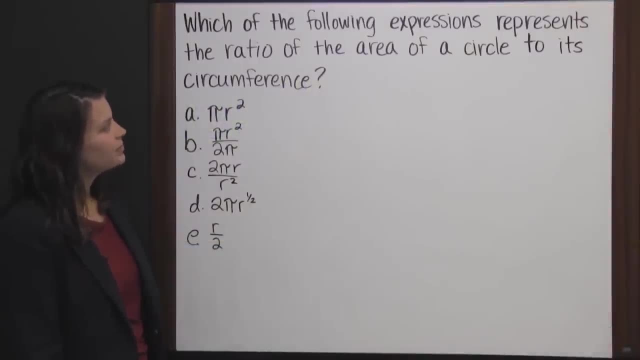 So answer b: Which of the following expressions represents the ratio of the area of a circle to its circumference? We've got some pretty key words here. The first one I see is ratio. A ratio is a comparison of two numbers like a fraction. 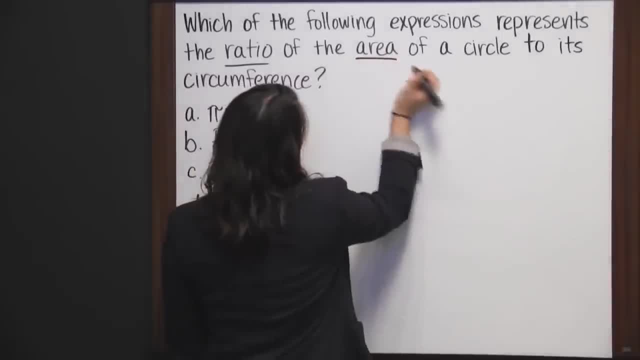 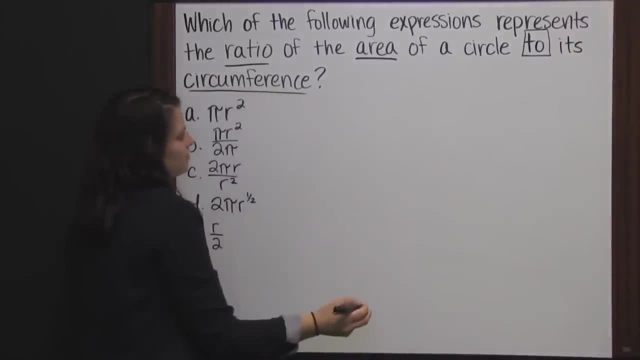 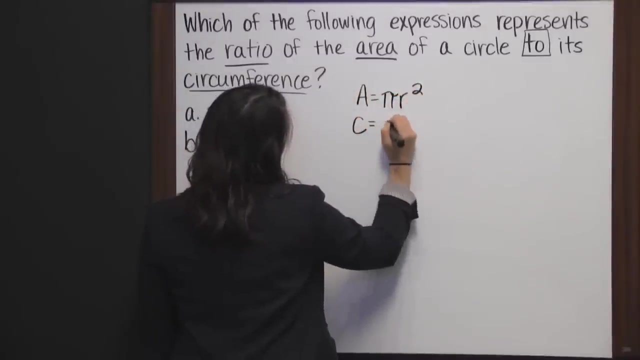 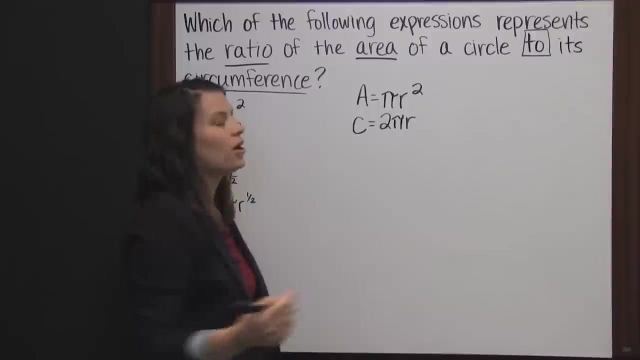 And what we're comparing is the area of a circle to its circumference. Well, the area of a circle is pi times radius squared, while the circumference of a circle is 2 times pi times radius. So the area is going to be our numerator. 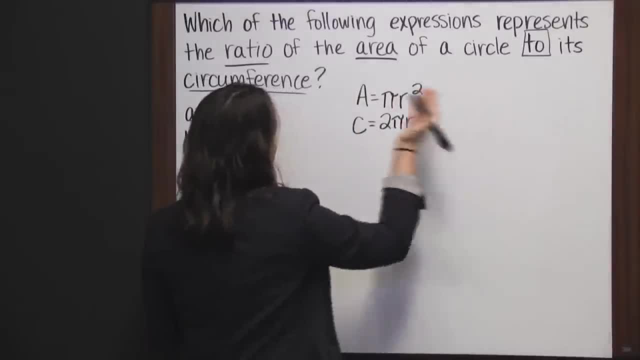 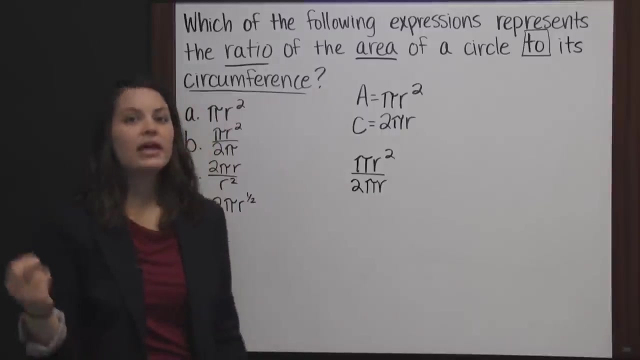 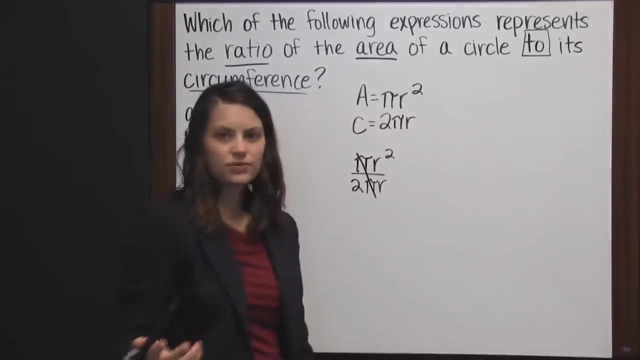 Since it was listed first, area to circumference means that the area should be in the numerator divided by this: 2 is your division bar the circumference, 2 times pi, times radius. And then we need to simplify. First I see that pi divided by pi cancels. 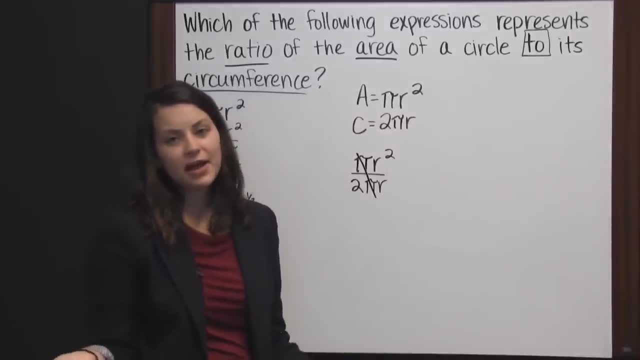 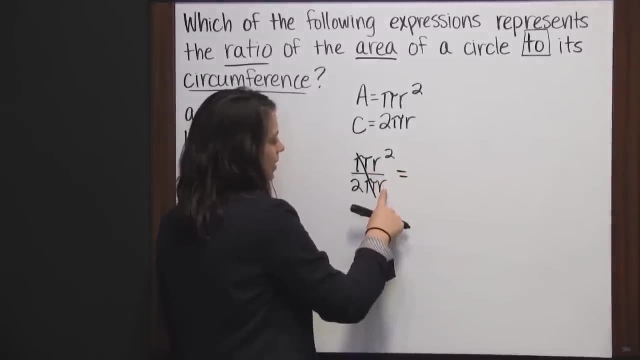 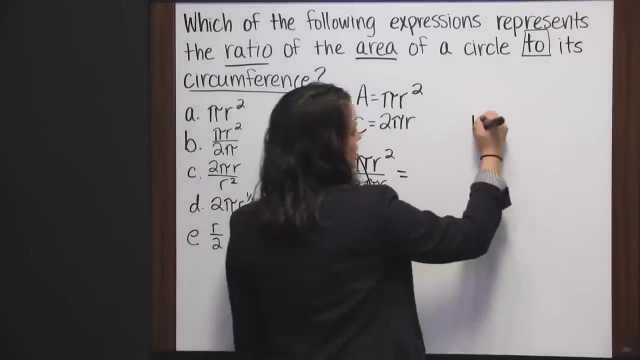 Pi divided by pi is 1.. Anything divided by itself is 1.. So we can cancel it. And then I can simplify: r squared divided by r. When you divide, you subtract the exponents, Or another way to think about it. is r squared is r times r. 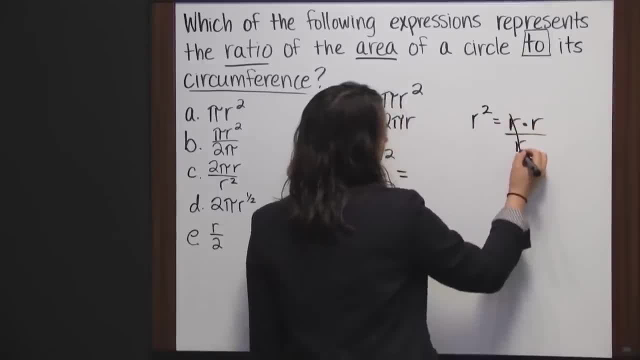 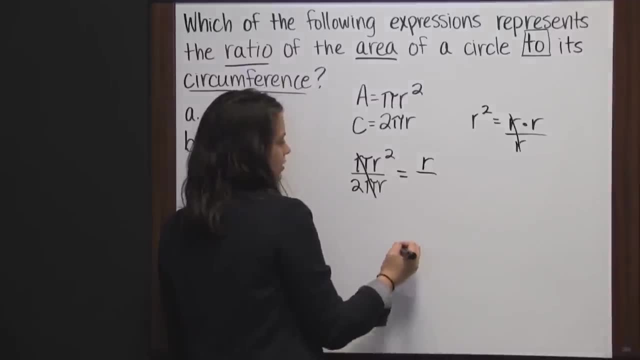 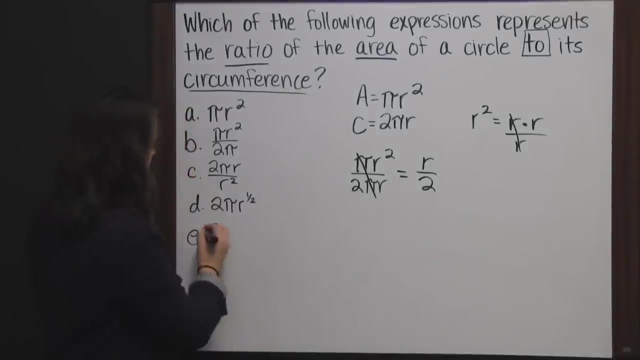 And I'm dividing that by r, And then you have something divided by itself is 1, or it cancels. So I'm left with just r in the numerator divided by 2 in the denominator, since those r's cancel. So we just have r divided by 2,. 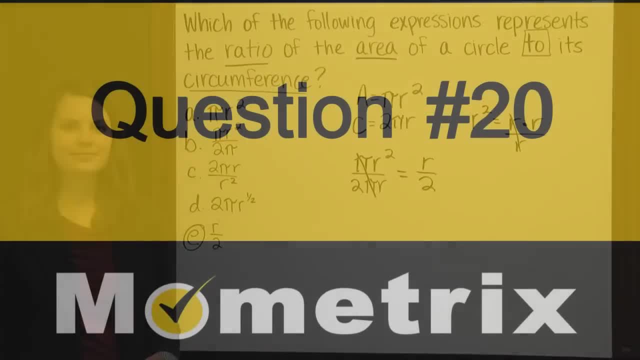 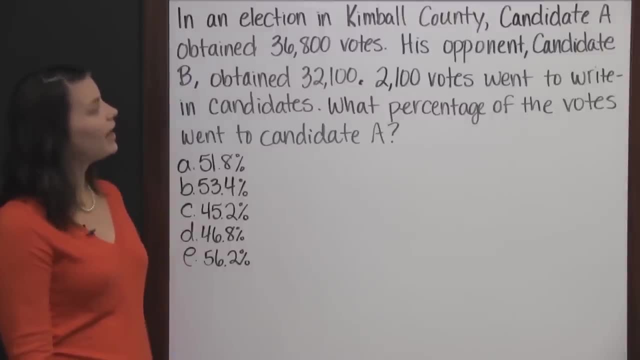 which is answer E. In an election in Kimball County, candidate A obtained 36,800 votes. His opponent, candidate B, obtained 32,100 votes. 2,100 votes went to write-in candidates. What percentage of the votes went to candidate A? 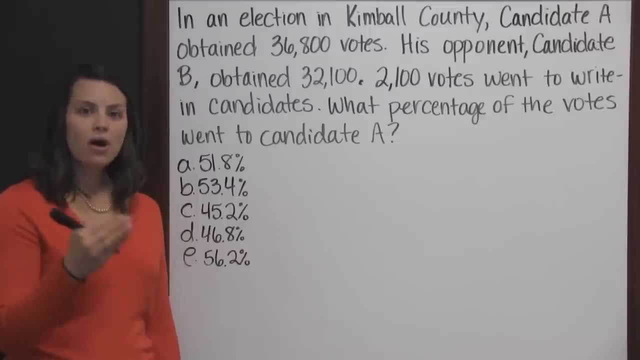 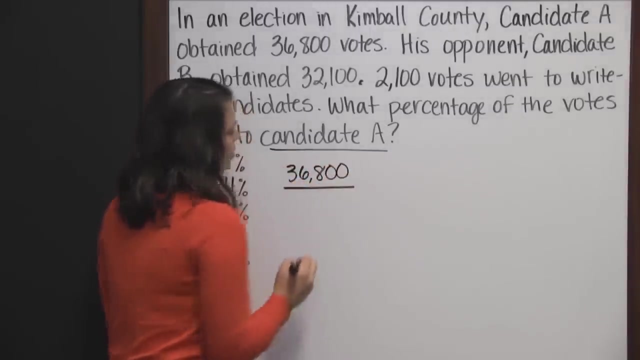 To find a percent, we need the part over the whole And we know the part. The part is the number of votes candidate A received, Which is 36,800.. What I need to know is the whole or the total number of votes. 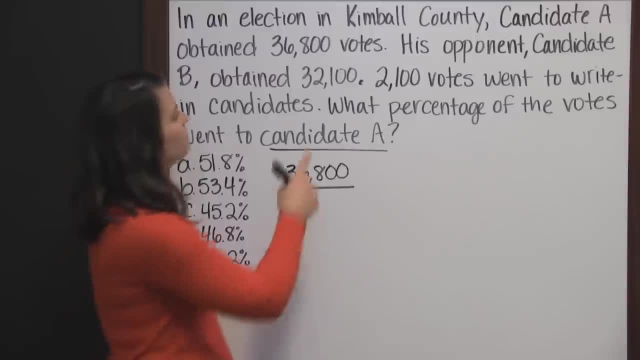 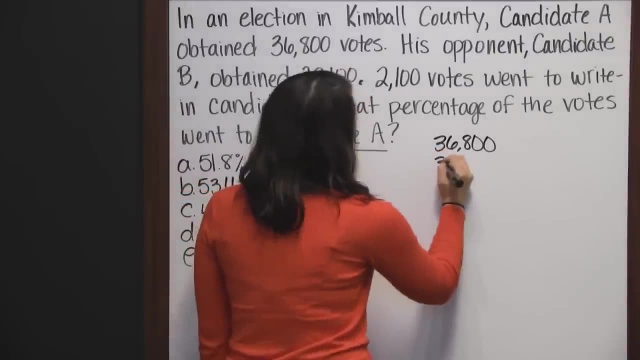 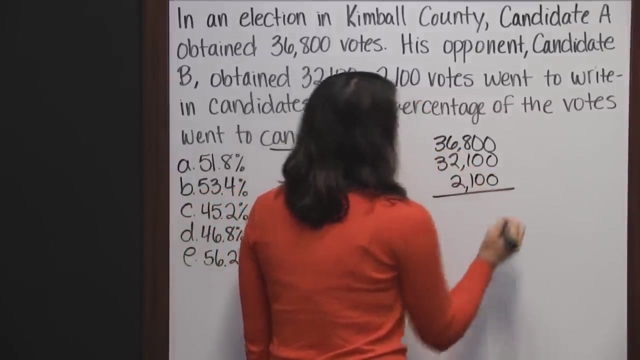 To find the total number of votes, we need to add up 36,800,, 32,100, and 2,100.. So that we can find the total. So we're adding, Those are 0.. And again we get 0. 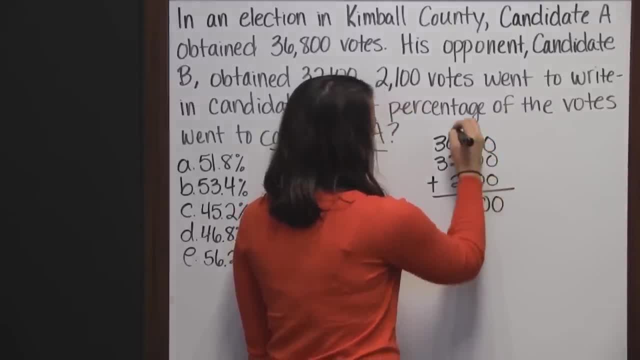 Then we have 8,, 9,, 10.. So that's a 0. Carry the 1.. We have 6,, 7,, 8,, 9,, 10,, 11.. Carry the 1.. And we have 3,, 6, 7.. 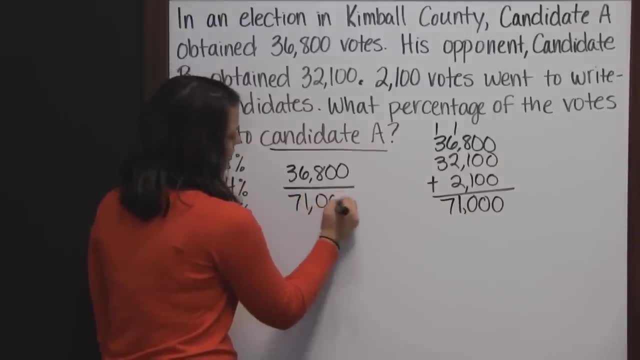 So that means there were a total of 71,000 votes. Now, to find our percent, we need to divide. That'll give us our decimal, which will then change into a percent. But before I divide, I'm going to first simplify this fraction. 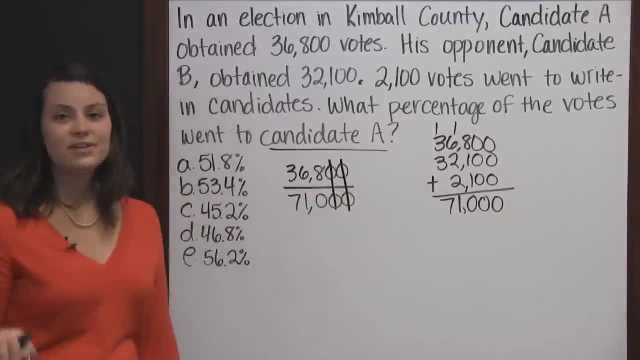 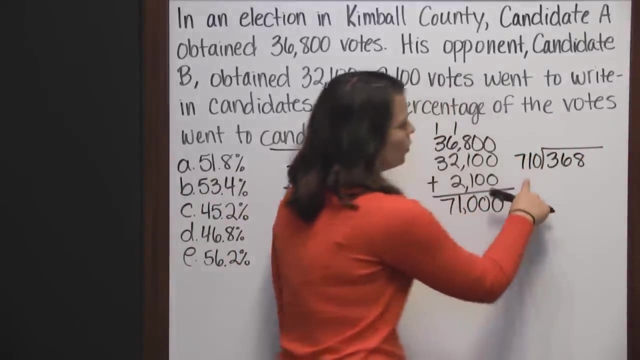 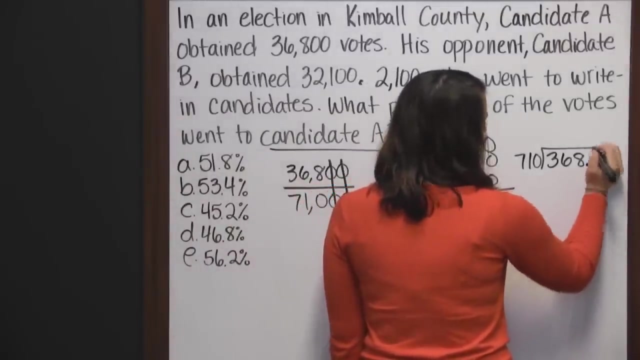 by canceling two zeros, And now my division will be a lot easier. So we need to divide 368 by 710.. Well, 710 doesn't go into 368 at all, which means I'm going to have to add a decimal and a 0.. 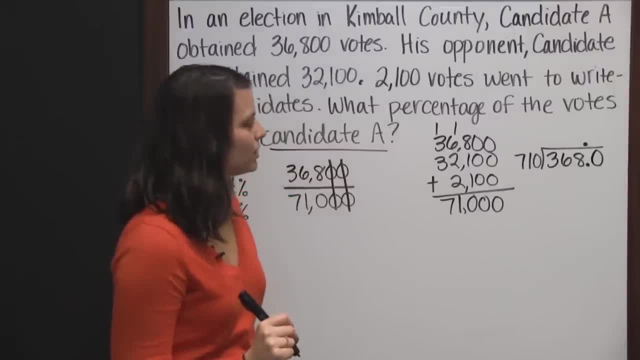 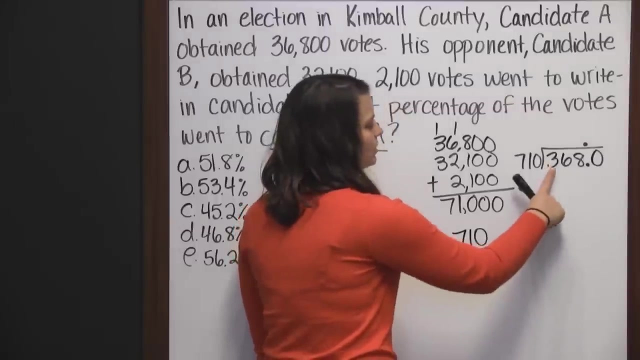 And now I can divide 710 into 3,680. So I can use compatible numbers here And 710 is very close to 700.. 700 times 5 would be 3,500.. So I'm thinking 710 is going to go about 5 times into 3,680. 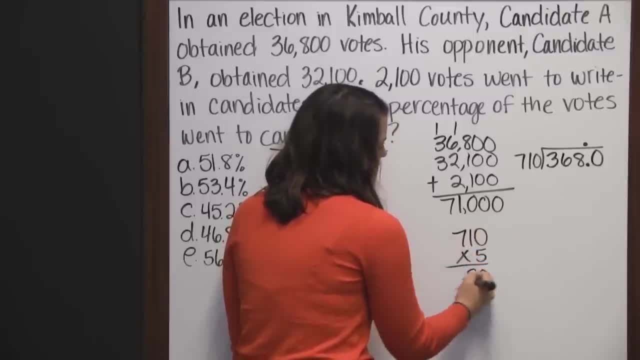 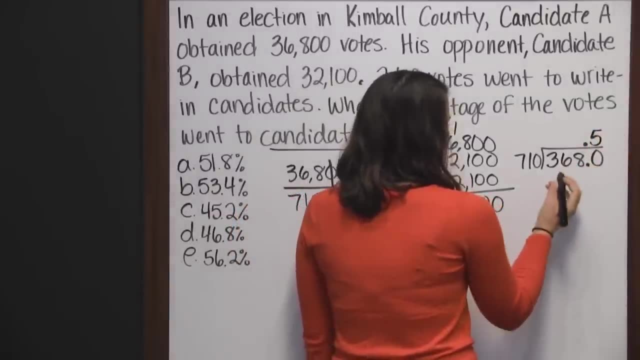 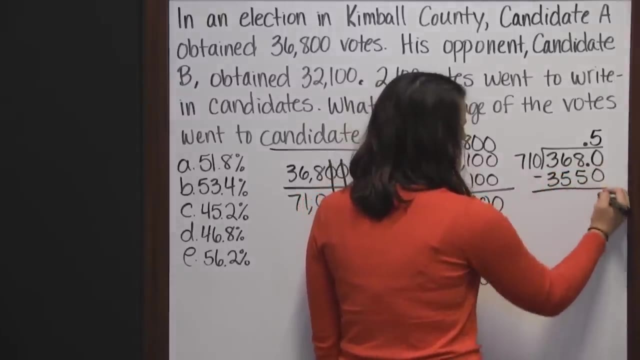 So let me multiply this. We get 0, and that's 5, and that's 35. So 3,550.. Yep, looks good, So that's 5.. We have 3,550.. Now we need to subtract. 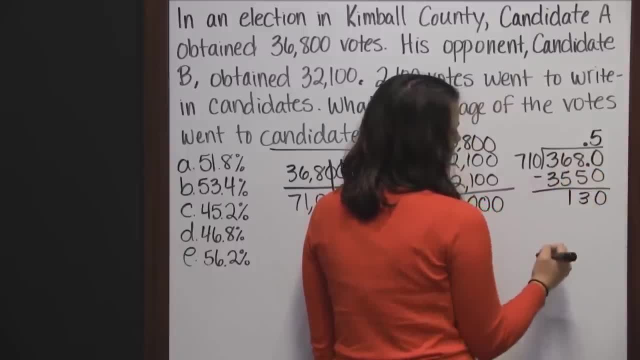 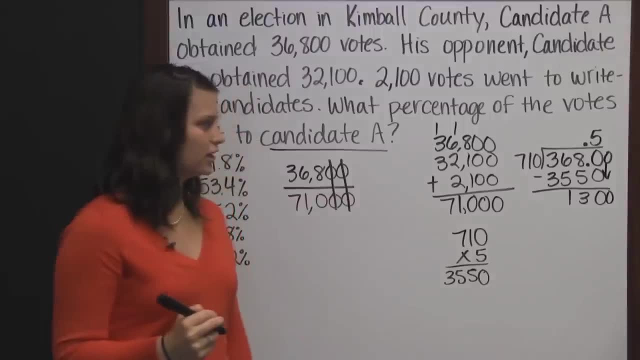 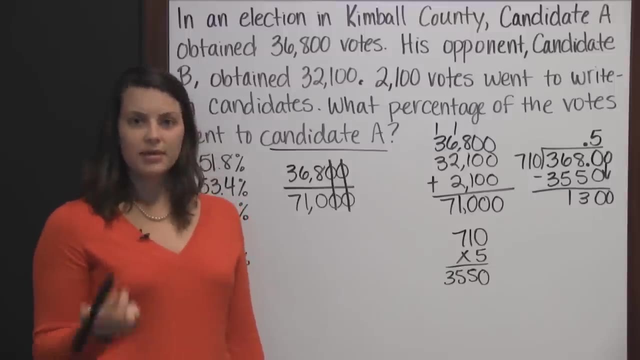 and that's 0, 1,, so 130.. Then we need to add a 0 and bring it down 1,300.. So 710.. And it's only going to go into 1,300 one time, because 700 plus 700 would be 1,400,. 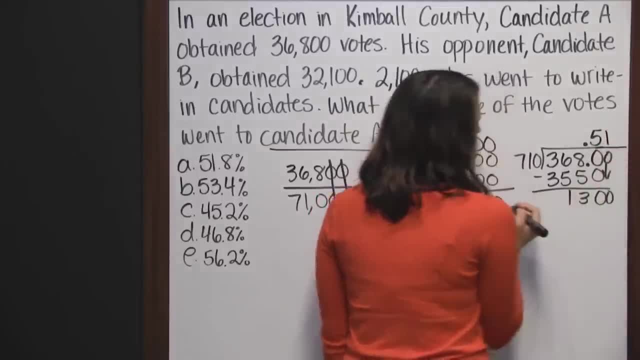 and that's too much. So it's just one time. 710 times 1 is 710.. Then we need to subtract, So I'm going to borrow from the 1.. That's a 0.. That's 13.. Borrow from the 13.. 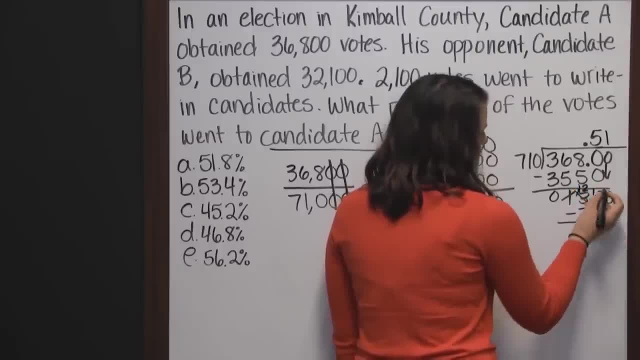 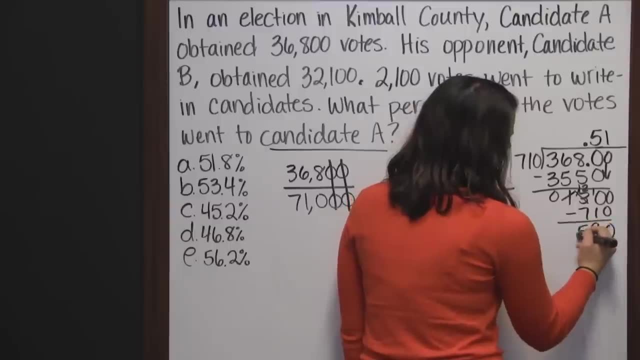 That's 12,, which makes that 10.. And we'll borrow. Well, we don't need to borrow, That's 0.. So 10 minus 1 is 9.. And 12 minus 7 is 5.. 590,, which makes sense. 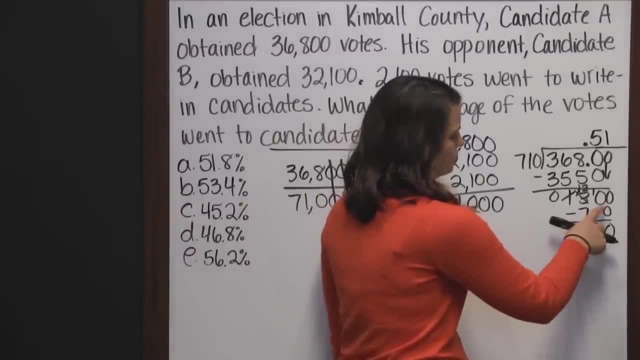 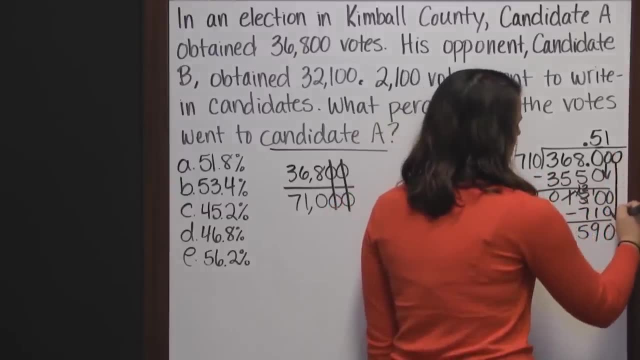 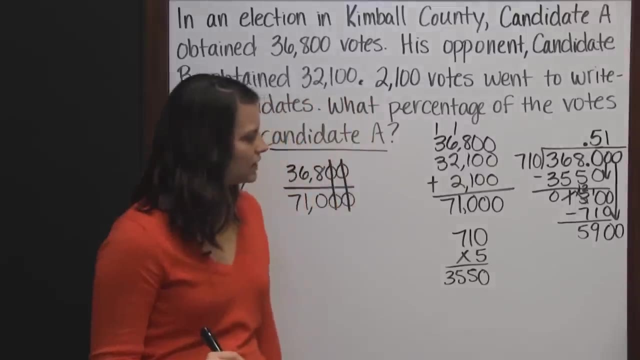 If you add 90 back to 710, you get 800.. And if you add 500 to 800, you get the 1,300.. So we need to add another 0 and bring it down. So now we need to know how many times 710 goes into 5,900. 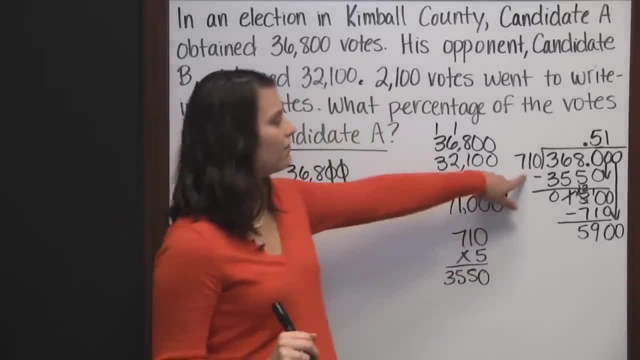 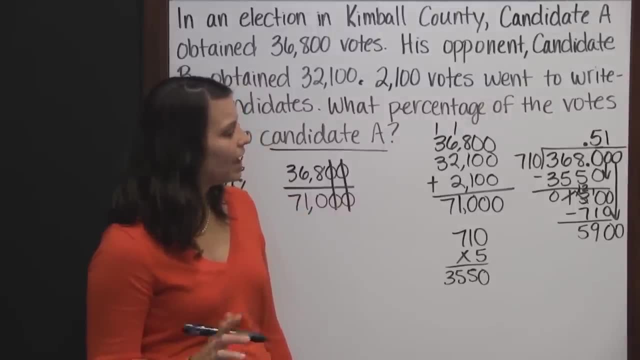 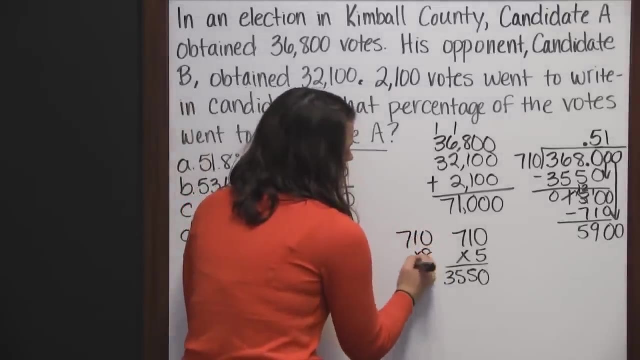 So I'm again going to use that compatible number of 700.. So let's see, 700 times 8 would be 5,600.. So I'm thinking it goes in there about 8 times. So that's 0, and that's 8,. 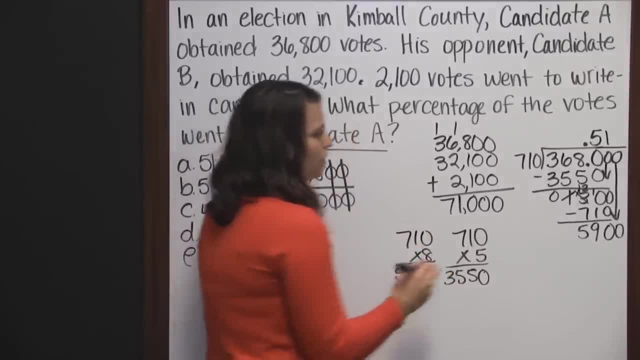 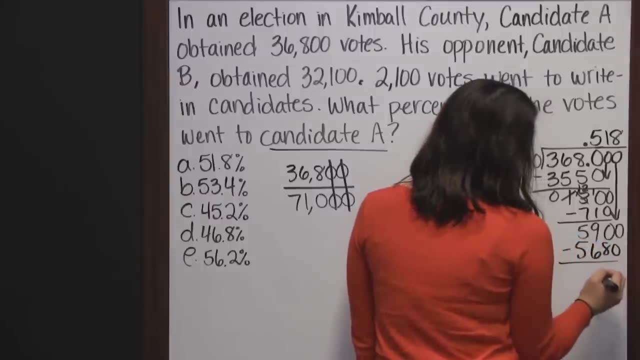 and that's 56.. So, yes, that's very close. So that's 8.. And we have 5680.. We can subtract and that's 0.. Borrow from the 9. That's an 8., So that's 10.. 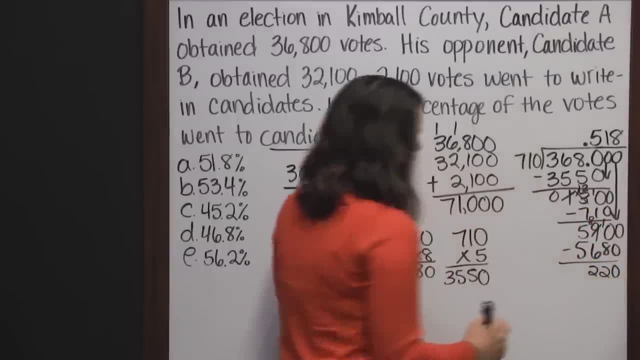 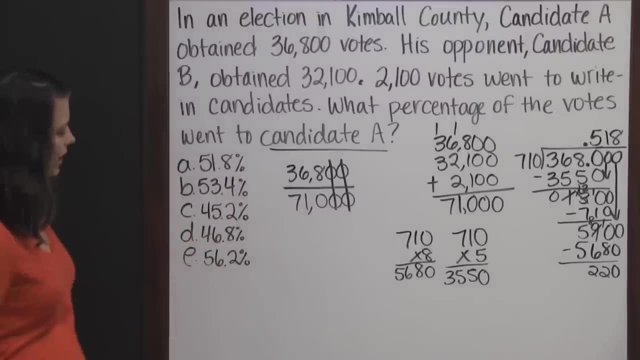 10 minus 8 is 2.. 8 minus 6 is 2.. So we get 220.. And we could keep going, but really that's all I need to know, because as I look at my answers, it's very clear. 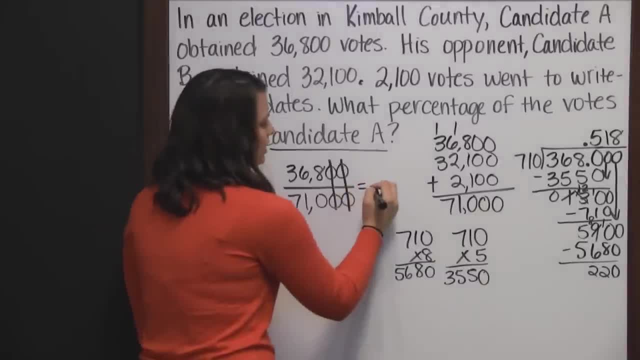 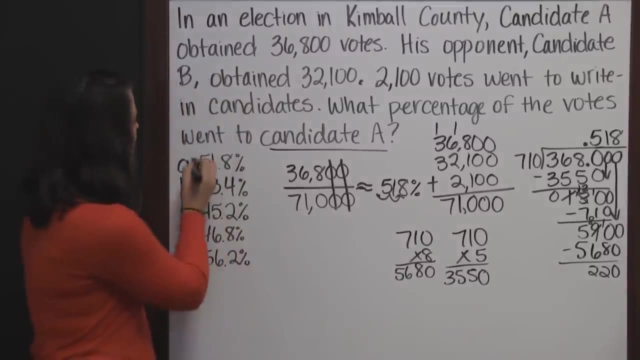 which one of these is my answer. This is well, it's about 518 thousandths. and then when we change it into our percent, we move our decimal two places to the right. we get 51 and 8 tenths percent. 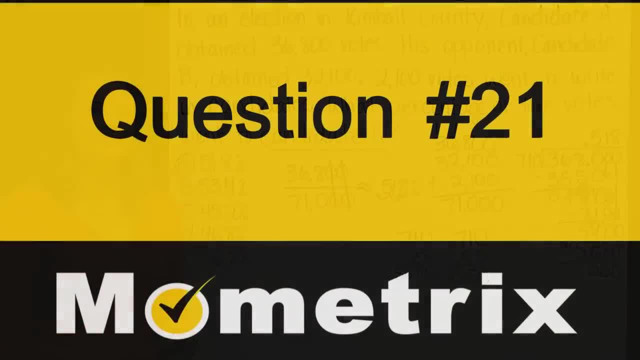 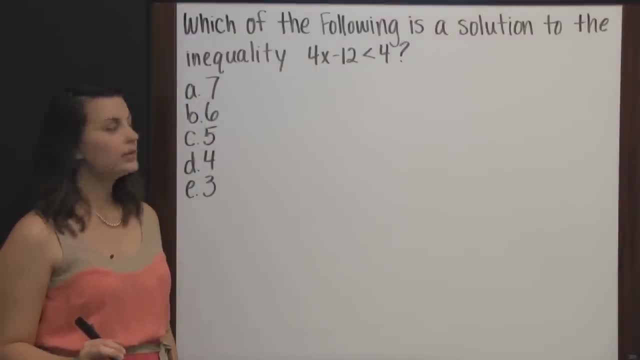 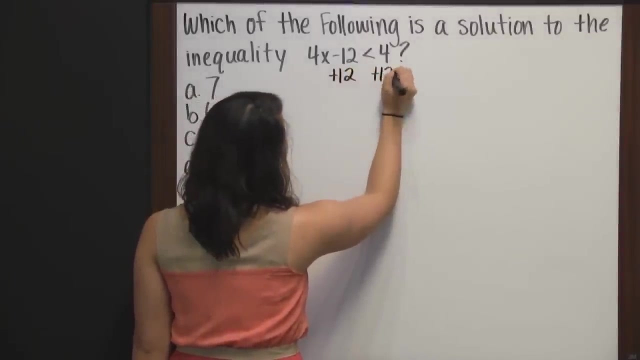 which is answer A. Which of the following is a solution to the inequality? 4x minus 12 is less than 4?. First we should solve for x in this inequality. So we're going to add 12 to both sides. bring down our 4x. 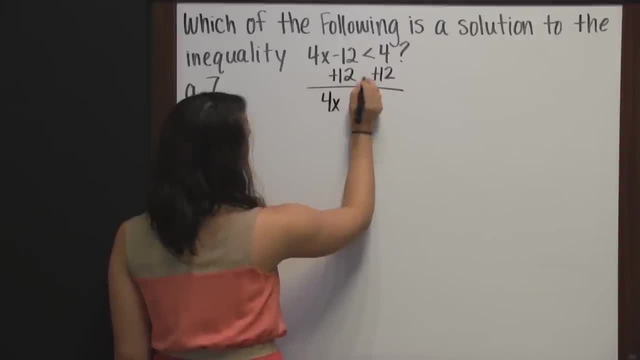 Minus 12 plus 12 is 0, so that cancels Bring down our less than sign and 4 plus 12 is 16.. Then we need to divide both sides by 4.. 4 divided by 4 is 1, times x is x. 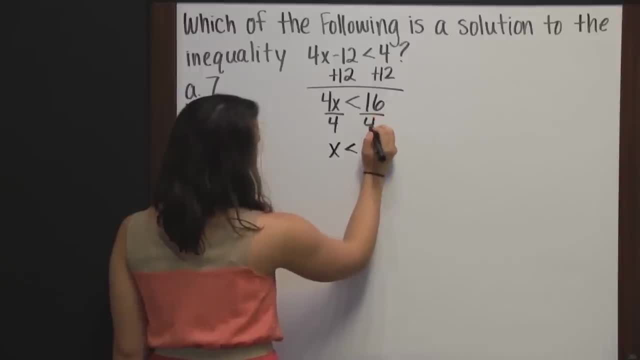 is less than 16 divided by 4 is 4.. Keep in mind when solving inequalities that if you multiply or divide both sides by a negative number, you must flip the inequality. In this case we didn't have to, since we didn't divide both sides by a negative number. 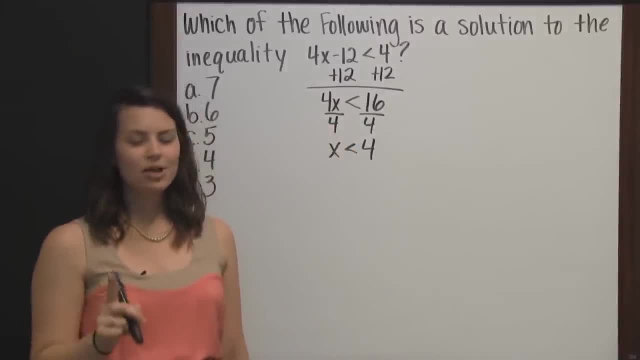 It's all about that negative. So now we can apply these answer choices. We want to find which one of these numbers is less than 4.. Is 7 less than 4? No. Is 6 less than 4? No. 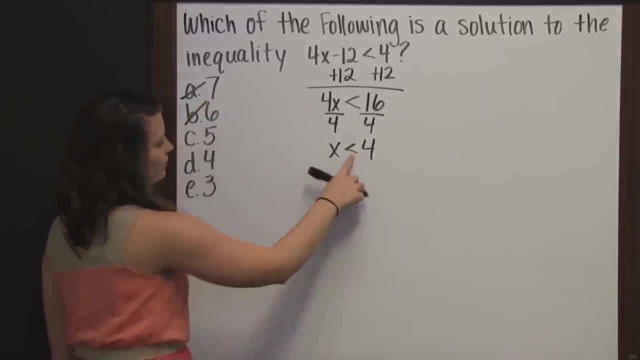 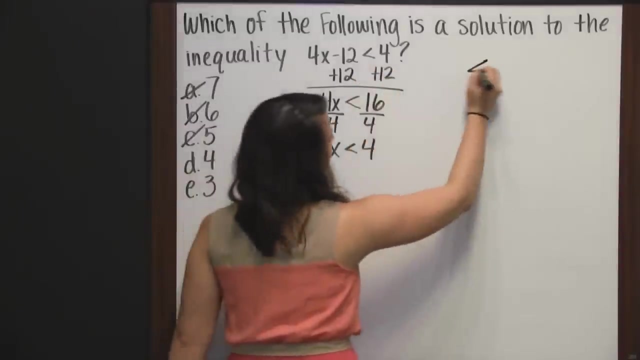 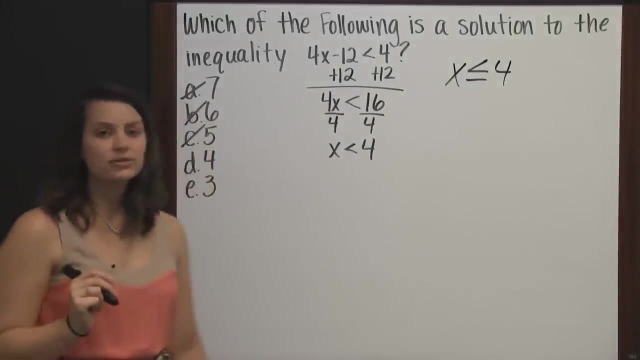 Is 5 less than 4? No. What about 4?? Is 4 less than 4? No. If this were a less than or equal to sign, if it said x is less than or equal to 4, then yes, 4 would be a solution. 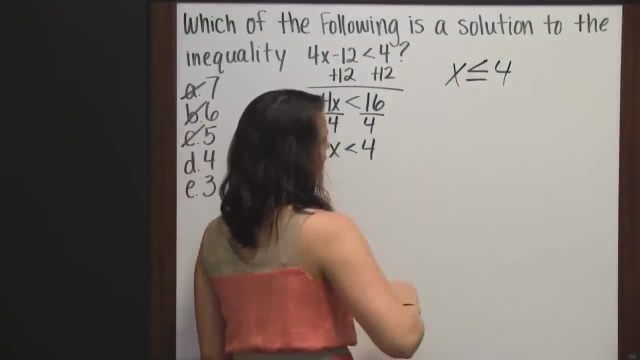 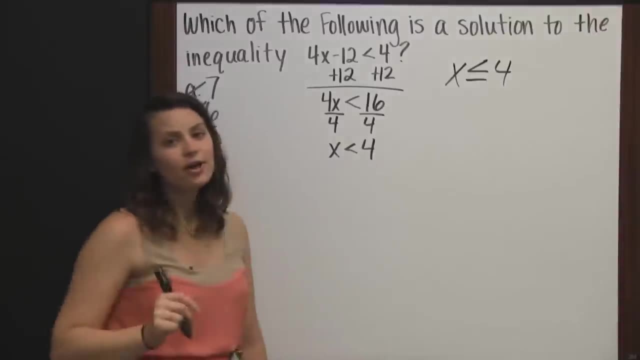 Because 4 is equal to 4. And it only has to be 1, either less than or equal to. But in this case it's not a less than or equal to sign, It's simply a less than sign, Meaning that this number must be smaller than 4.. 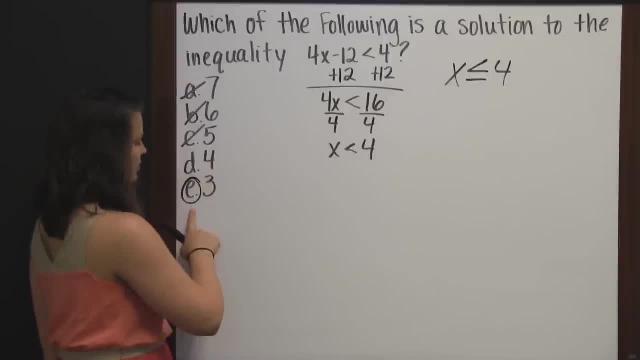 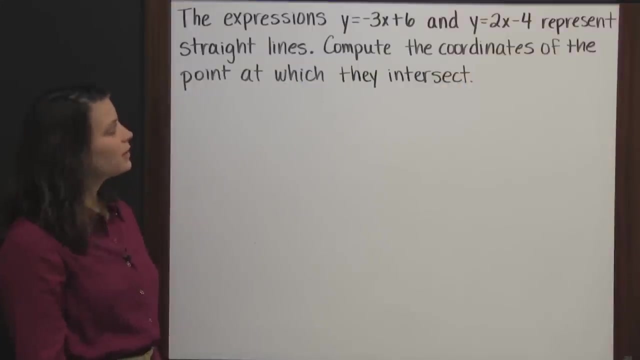 So our answer is: E, 3 is less than 4.. Or 3 is a smaller number than 4.. The expressions y equals negative 3x plus 6 and y equals 2x minus 4 represent straight lines. Compute the coordinates of the point. 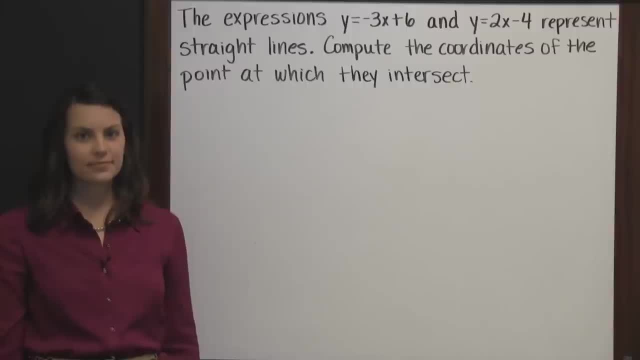 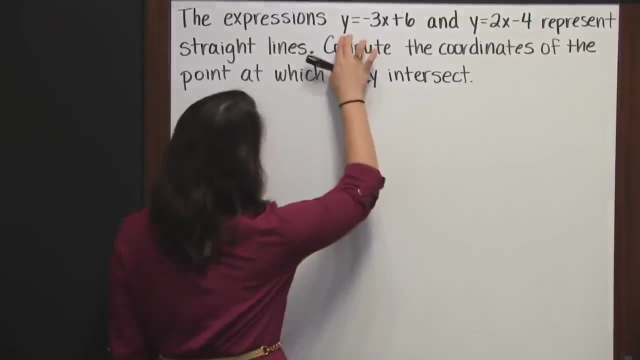 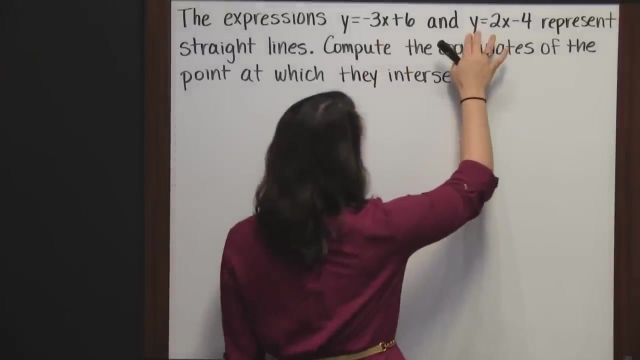 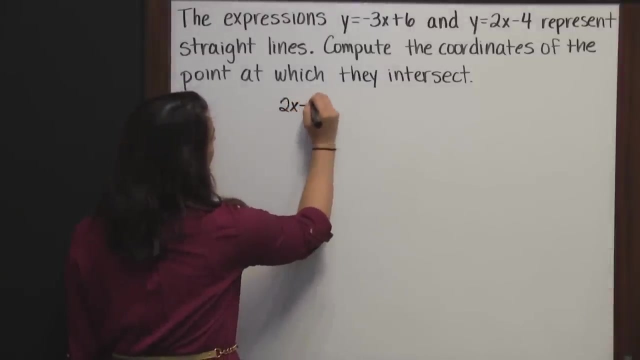 at which they intersect. This can be done by substituting 2x minus 4 for y in our other expression, Or by substituting negative 3x plus 6 for y in this expression. Either way, the result is 2x minus 4. 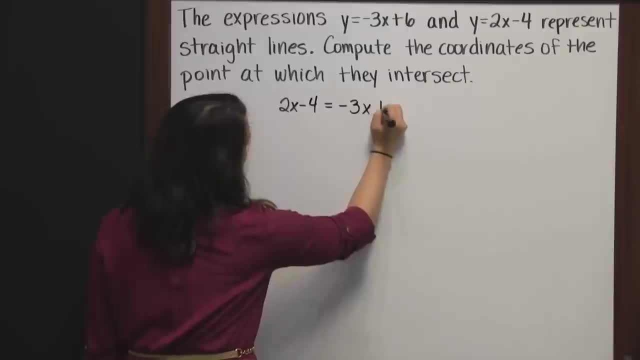 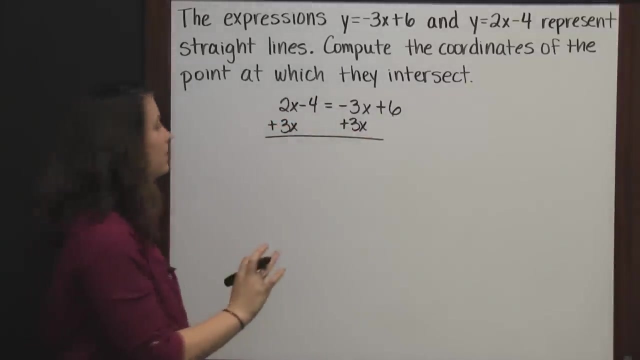 equals negative 3x plus 6.. Now we need to solve for x. First I'll add 3x to both sides so that I can get all my x's on one side of the equation. 2x plus 3x is 5x. 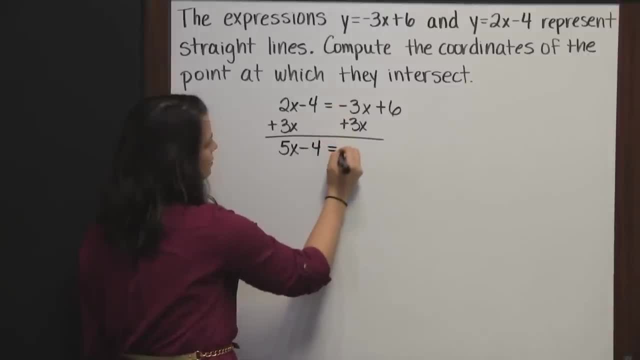 minus 4 equals negative. 3x plus 3x cancels and I'm left with 6 on the right side. Now we need to add 4 to both sides. Bring down the 5x Negative. 4 plus 4 is 0.. 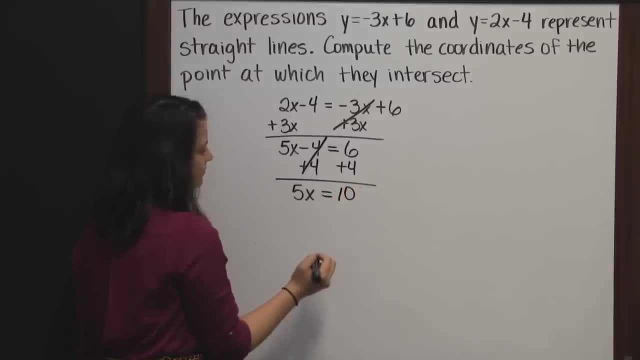 Negative: 4 plus 4 is 2x. Remember to add 4 plus 4.. So that's positive 4 point 4, minus 1. sort of negative 4 plus 1 and 0 is. And now on to this question. 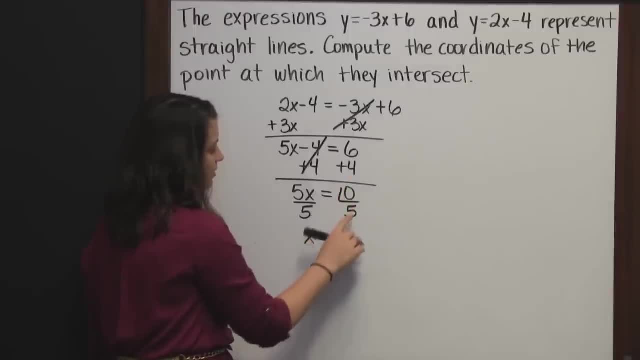 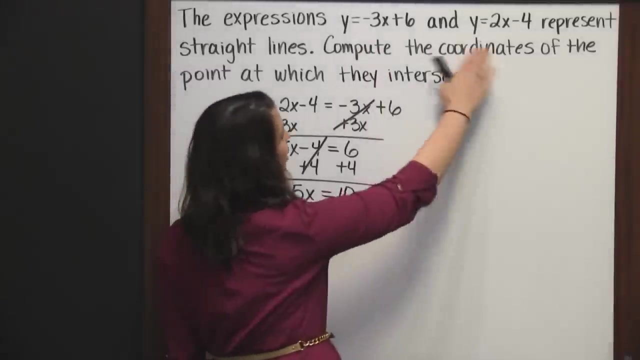 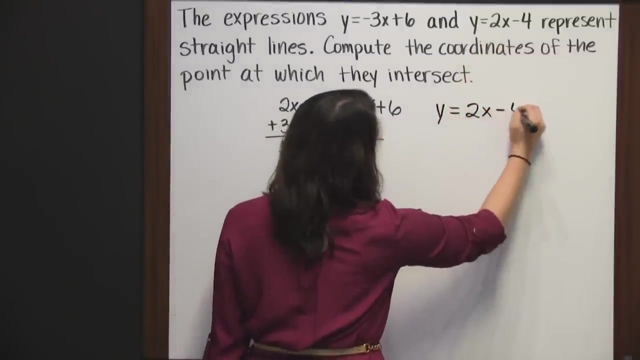 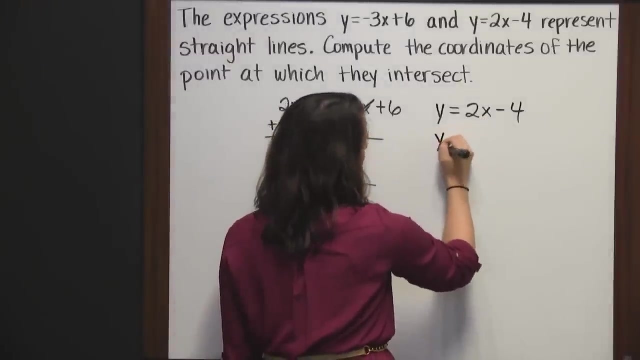 how do we solve for x, To solve for a certain докумptious professor or Здetry-Chem's lecture, or to substitute 2 for X in either one of these expressions, and I'm going to use the second one. Since X is 2, we need to replace X with 2 to find Y. So Y equals 2 times 2 minus 4.. 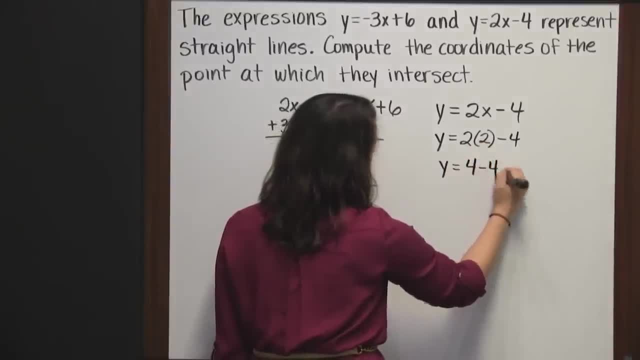 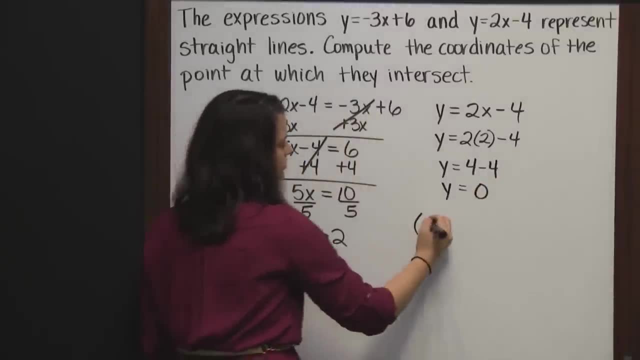 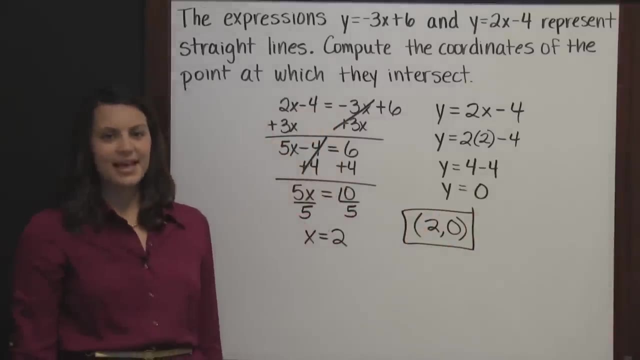 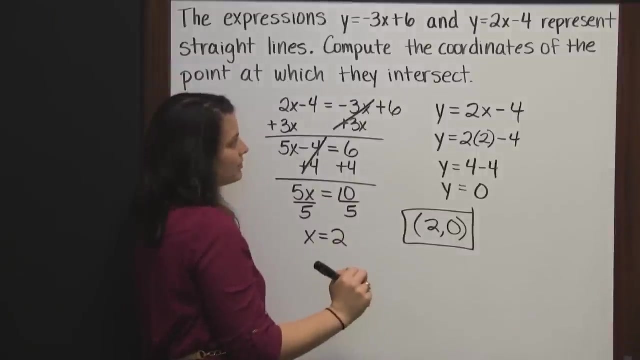 Y equals 2 times 2 is 4 minus 4.. So Y equals 0.. Our ordered pair is 2, 0. And you can always check this by plugging this ordered pair back into both of your expressions and you should. 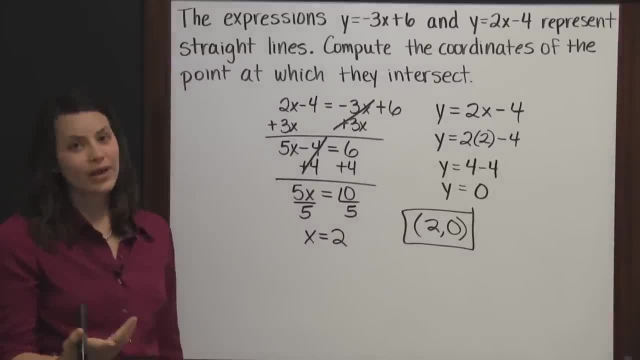 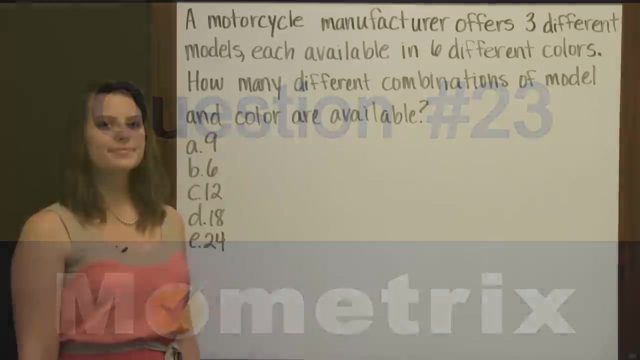 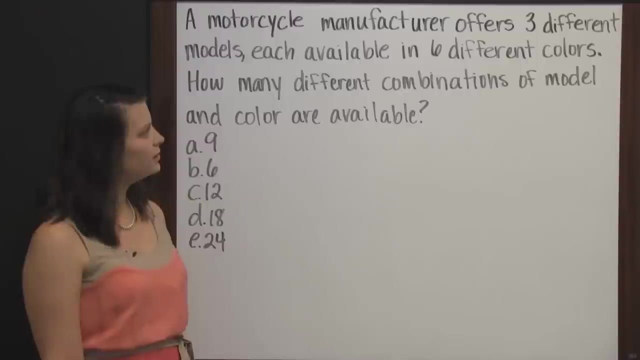 get a true mathematical result Equation there when you do that, And if you didn't, then you know that you've made an error somewhere in your work. A motorcycle manufacturer offers three different models, each available in six different colors. How many different combinations of model and color? 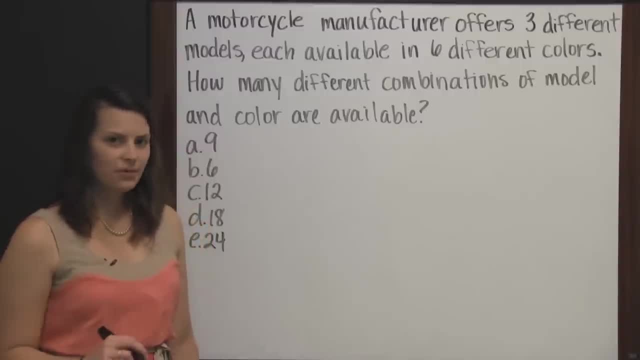 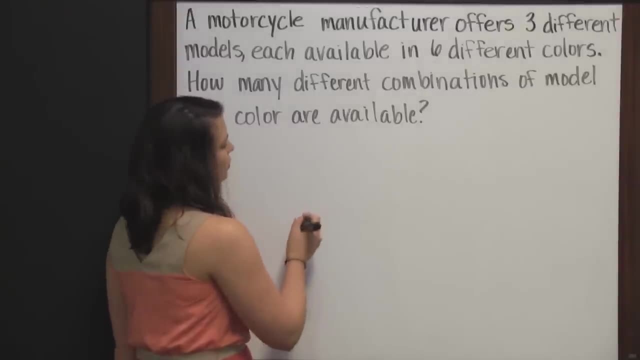 are available. There are a couple of different ways we could figure out this problem. First, I'm going to show you a visual representation. So if we say, our models are A, B and C, These are the three different models of cars you can get, And then for colors we use the numbers 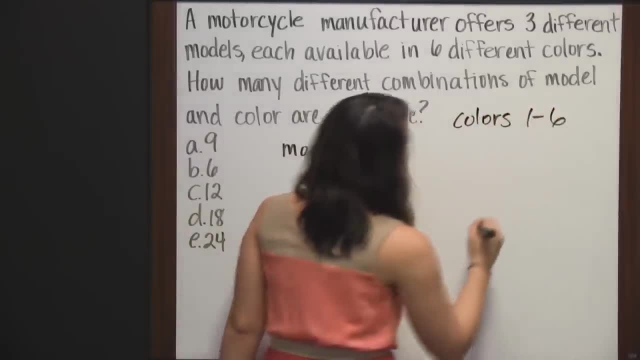 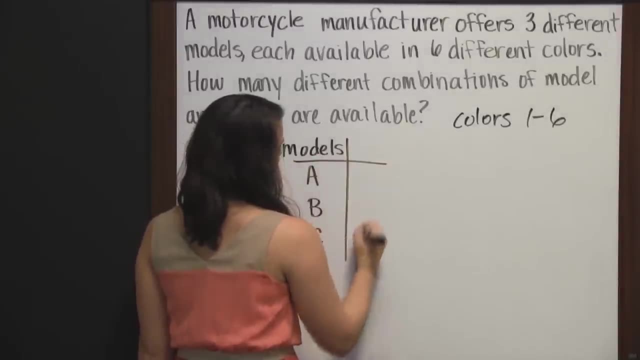 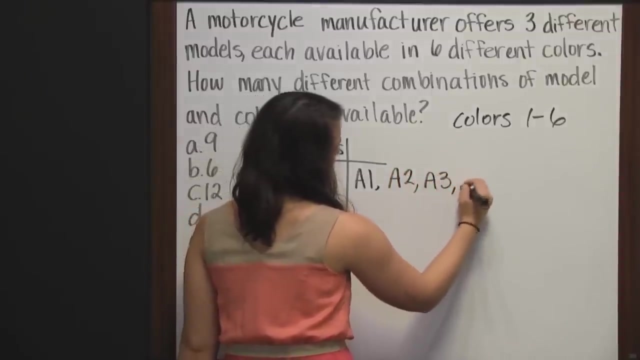 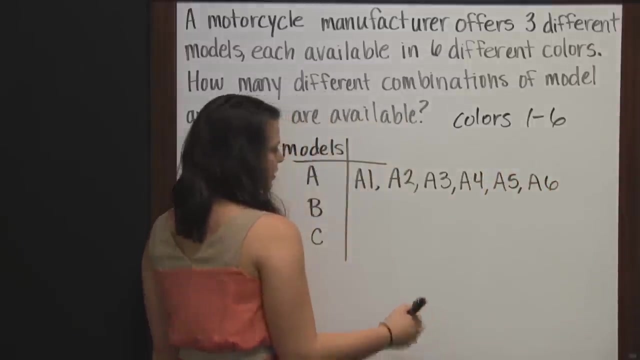 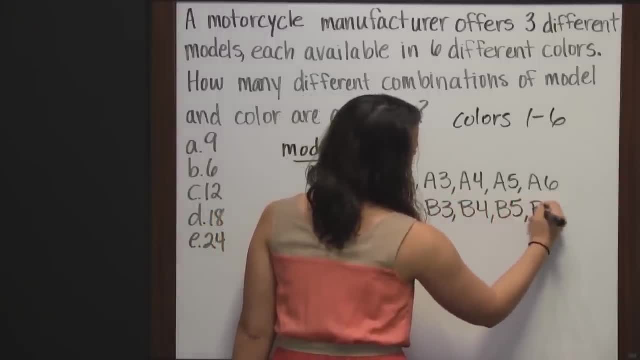 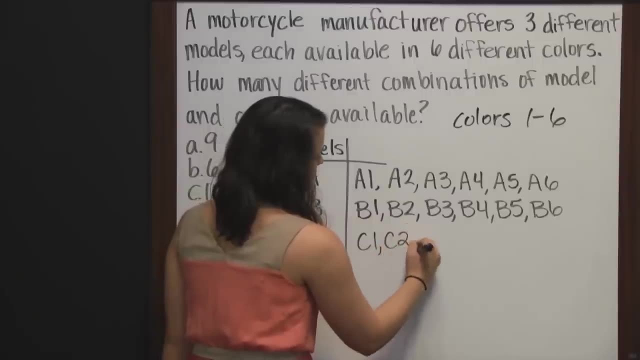 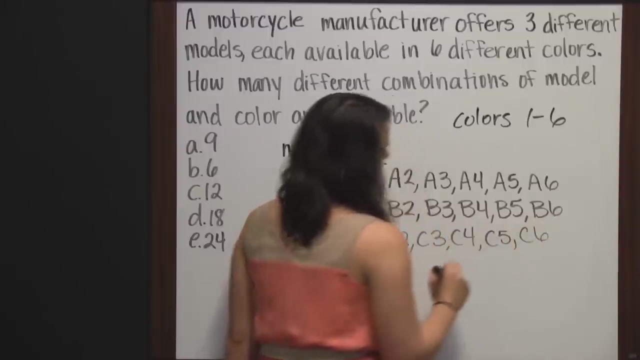 Same thing with model B. You could get model B in color 1, color 2,, color 3,, color 4,, color 5, or color 6.. And finally, the same with model C: Color 1,, color 2,, color 3,, color 4,, color 5, and color 6.. 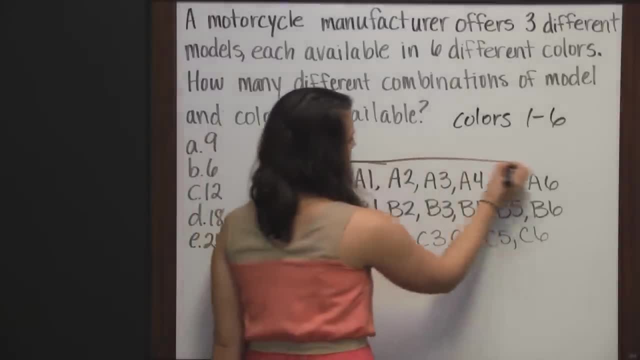 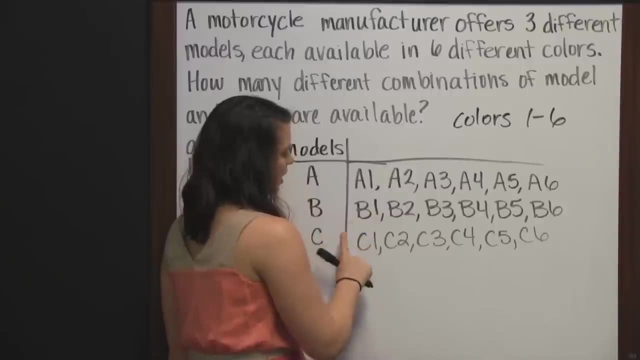 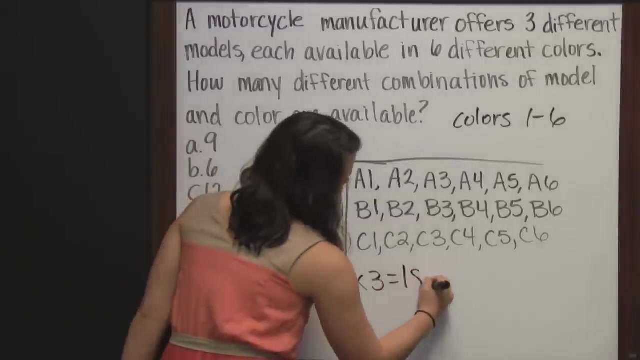 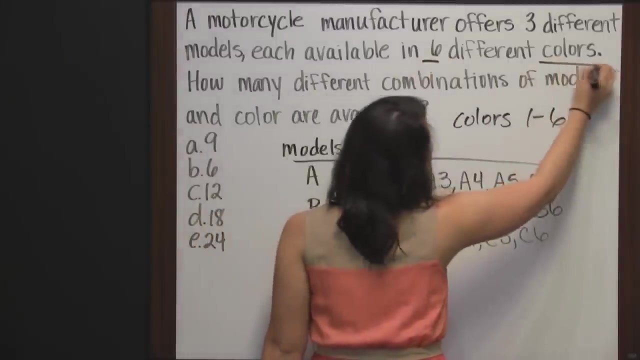 And if we count up all of these different combinations, we have six for model A, 6 for model B and 6 for model C, or 6 times 3, which is 18.. So, instead of writing this all out, we could have taken our 6 colors and multiplied it by our 3 models. 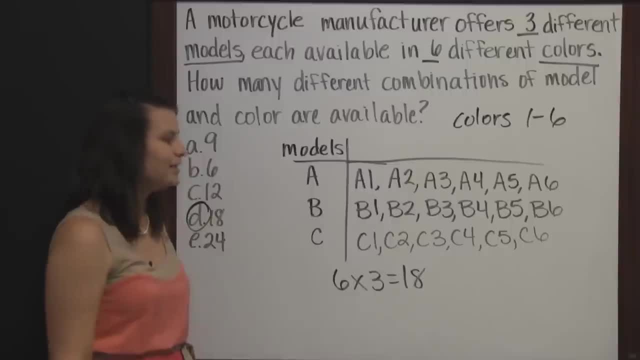 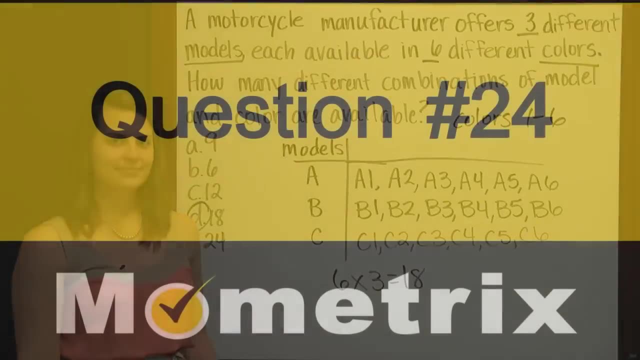 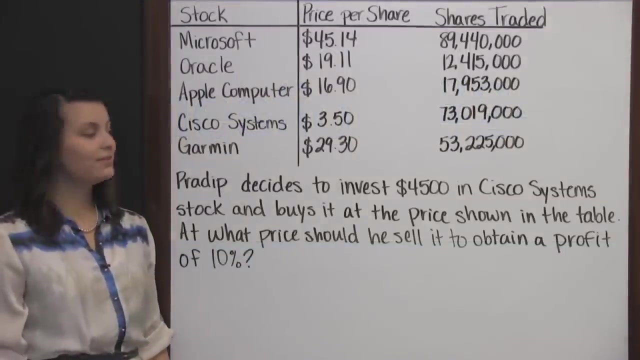 3 times 6 is 18, so there are 18 different model and color combinations. Pardeep decides to invest $4,500 in Cisco Systems stock and buys it at the price shown in the table. At what price should he sell it? to obtain a profit of 10%. So he's buying Cisco Systems stock at $3.50 per share. If he wants to make a profit of 10%, then he needs to sell his stock when the price per share is 10% higher. and there are several ways to solve this problem. I'll show you one. 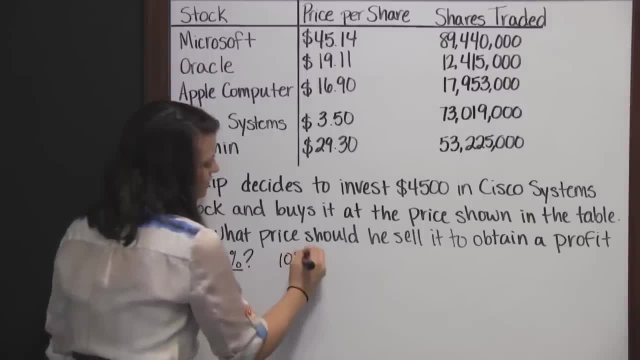 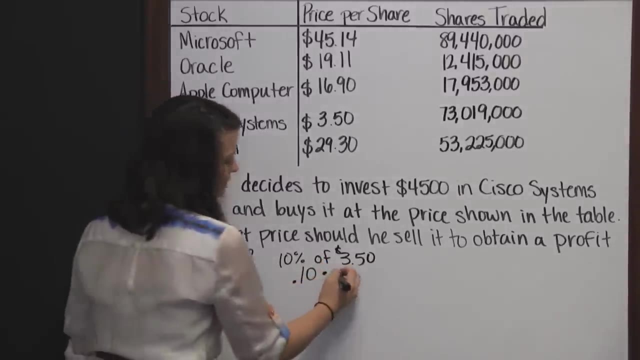 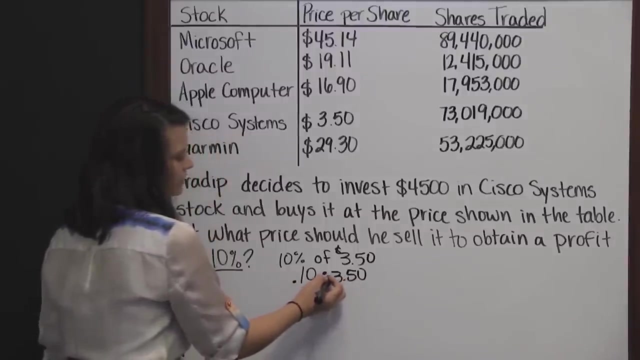 So first I want to know what is 10% of $3.50?? Well, of means to multiply. So I'm multiplying times 1 tenth or times 10 hundredths. And multiplying times 10 hundredths means just moving that decimal one place to the left. 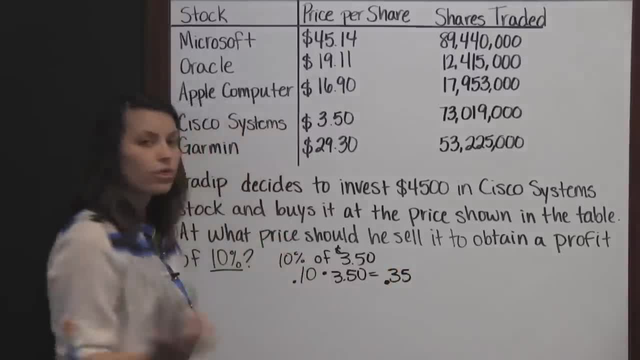 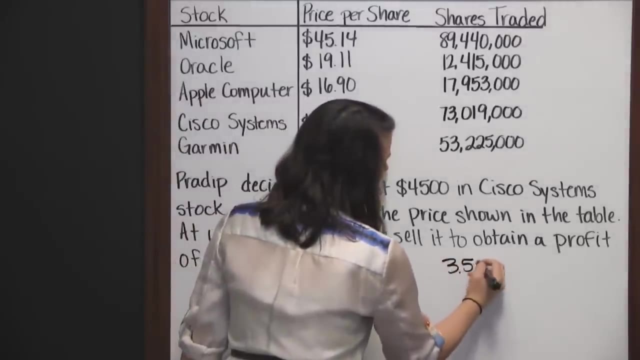 So that is 35 hundredths or 35 cents. So that means that his stock needs to be 35 cents higher. The price per share needs to be 35 cents greater. So 3 dollars and 50 cents plus 35 cents is 3 dollars and 85 cents. 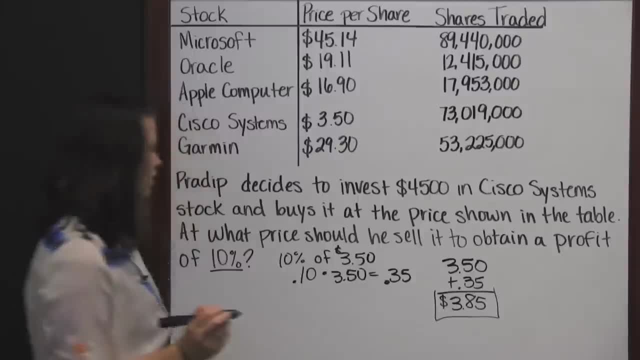 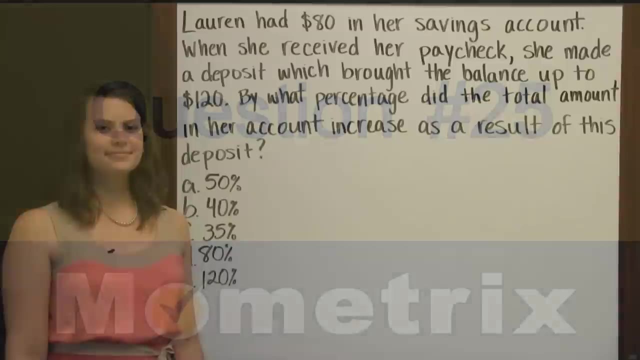 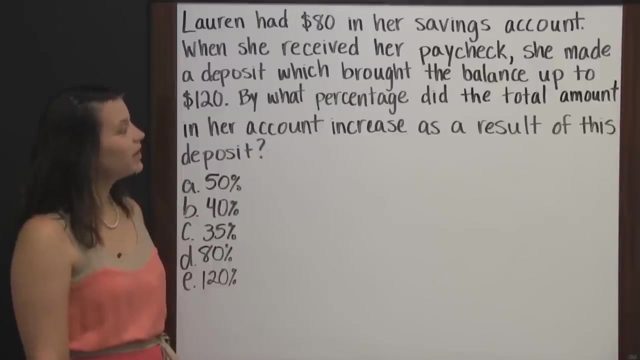 So in order to make a profit- a 10 percent profit- then he needs to sell his stock at 385 per share. Lauren had 80 dollars in her savings account When she received her paycheck. she made a deposit which brought the balance up to 120 dollars. 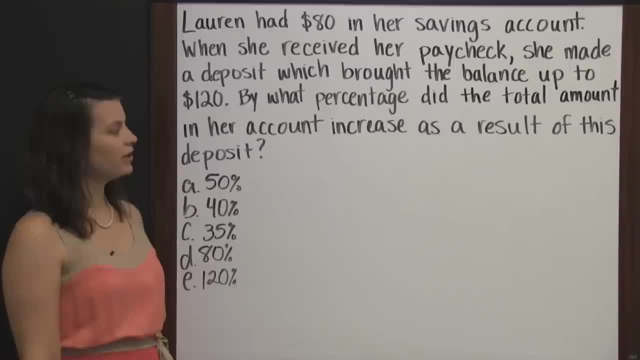 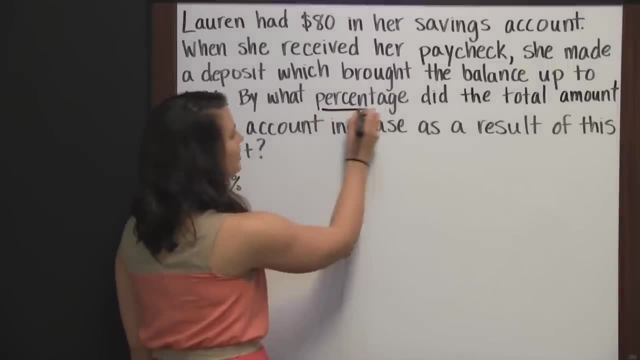 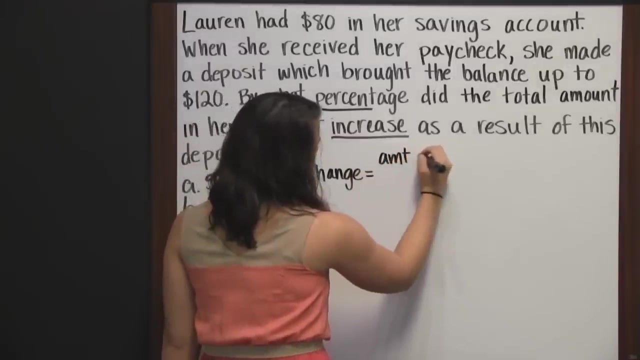 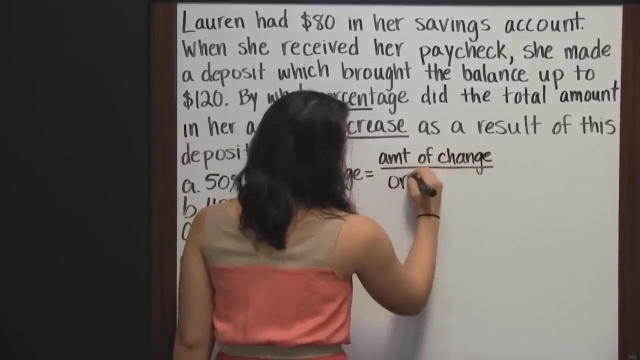 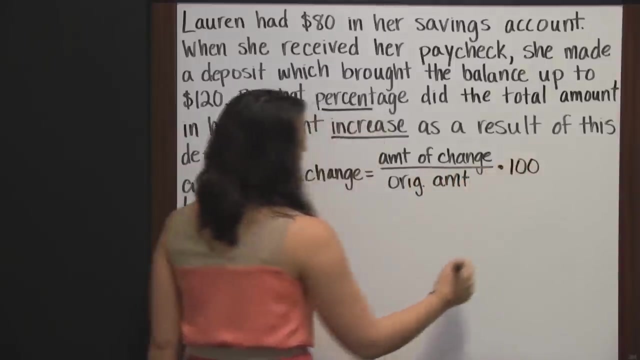 By what percentage did the total amount in her account increase as a result of this deposit? This is a percent increase problem And there's a formula for that. The formula to find a percent of change is to find the amount of change, divide that by the original amount and then multiply that amount by 100.. 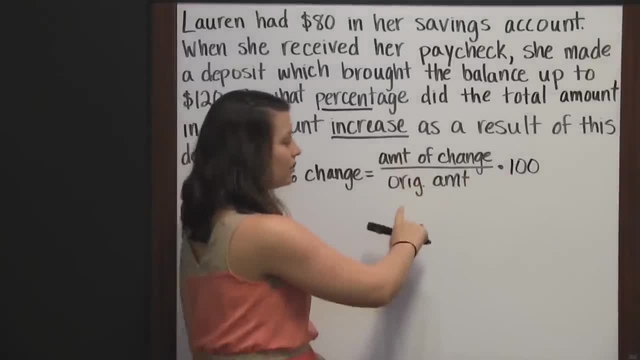 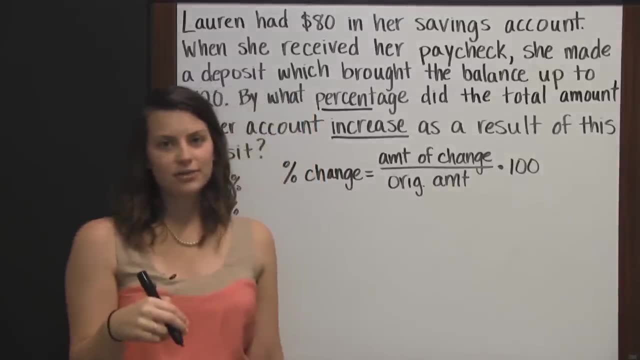 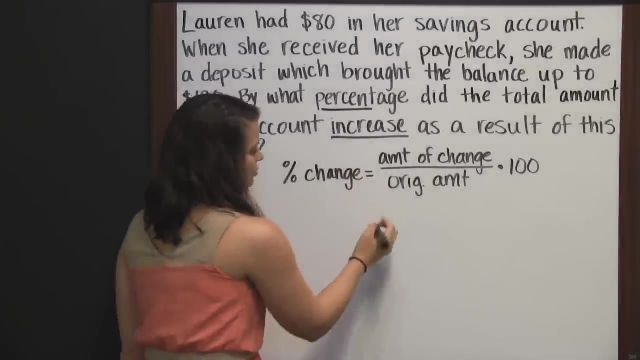 And the reason you multiply by 100 is because when you divide you'll get a decimal answer, And to change a decimal to a percent you multiply by 100. Or simply move the decimal two places to the right. So first we need to find our amount of change. 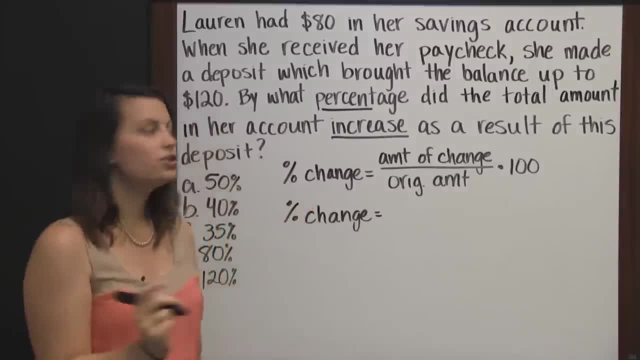 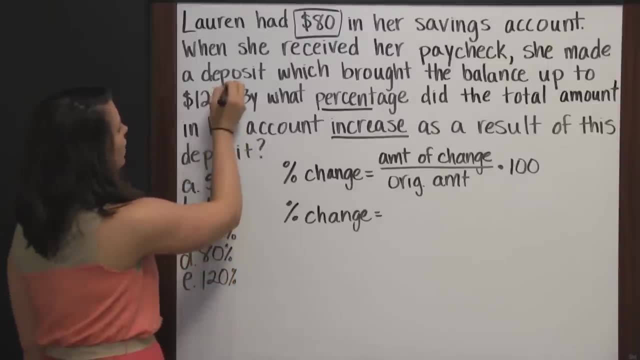 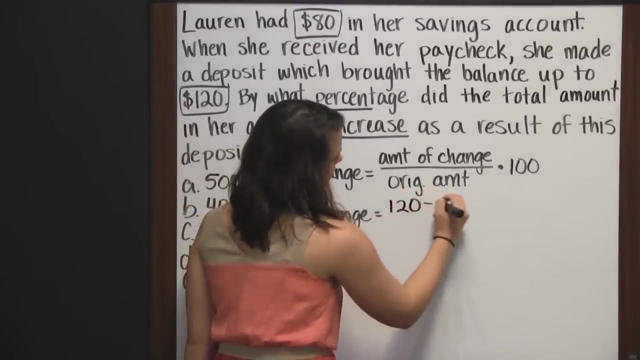 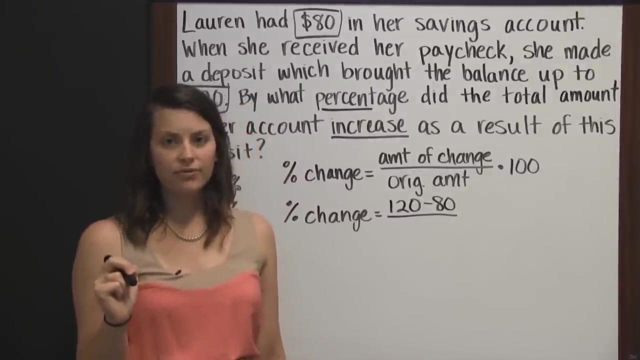 The amount of change is found by subtracting the two amounts. So she started at 80 dollars and her balance went up to 120 dollars. So the change is 120 minus 80, divided by the original amount, So what she had in her account before she made her deposit. 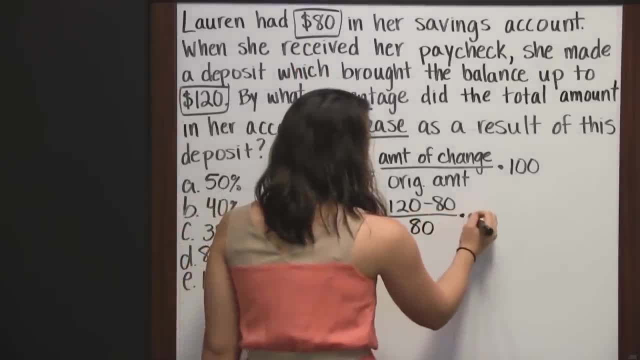 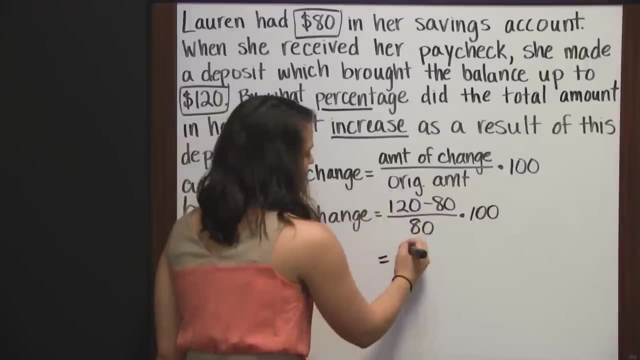 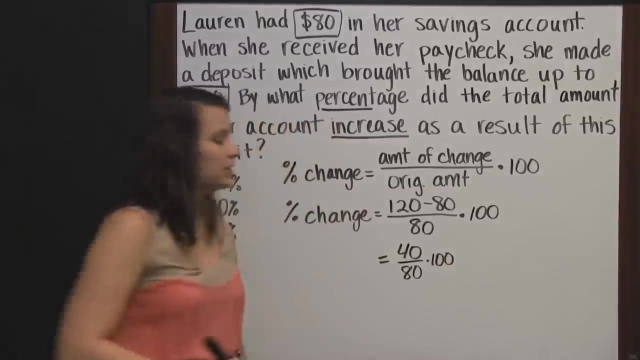 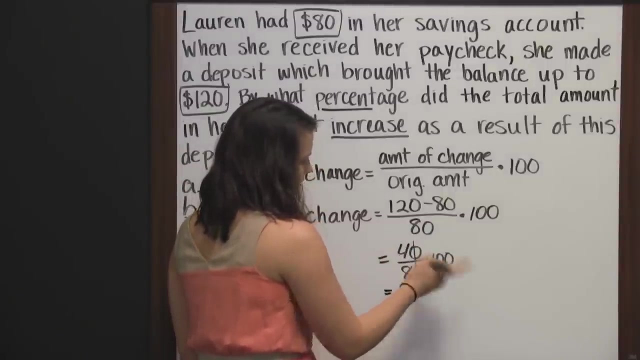 the 80 dollars, And then we multiply that by 100. So the percent change is 120 minus 80, divided by 80, times 100.. To simplify this, we can first cancel a zero, So we have 4 eighths times 100. 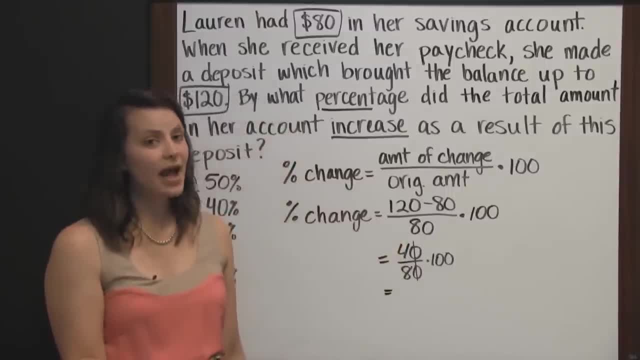 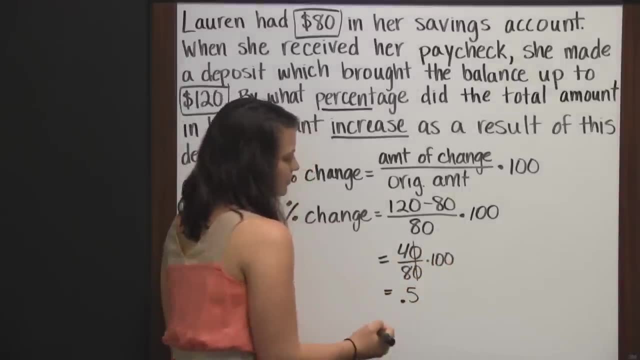 And 4 eighths can be simplified to 1 half or, since we want to change it to a percent, 5 tenths, Which again is equivalent to 4 eighths or 1 half. So we multiply that times 100.. 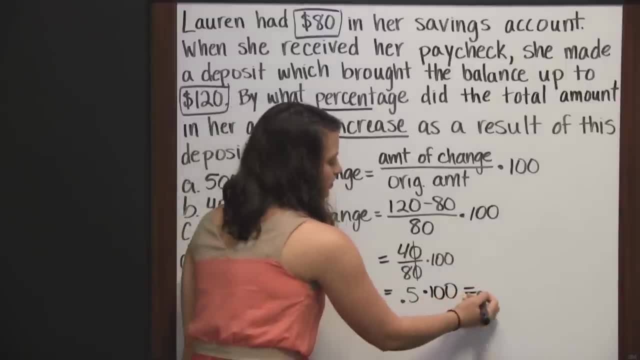 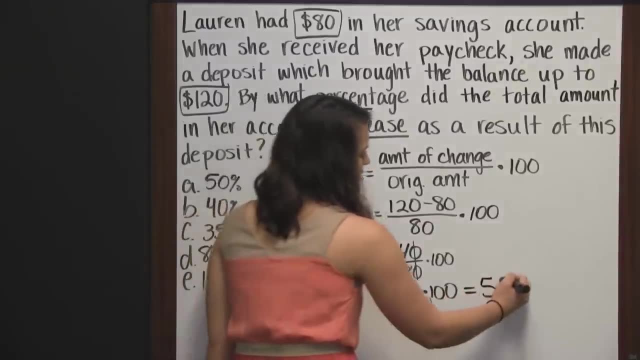 This is our decimal, but we want a percent. So multiplying by 100 simply moves your decimal two places to the right And we have to fill this empty seat with a zero. So it's 50 percent. It was a 50 percent increase. Answer A.